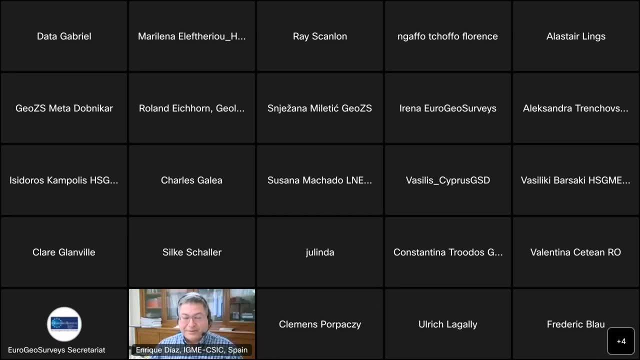 talk more about the different scientific practices that we have been working in the past and these technologies. Let us welcome Dr Roland Eichhorn from the European Geo-Geological Survey of Ireland, If you want to share your screen and the talk from Roland. as I was mentioning, is called a bottom up approach to enhance visibility and awareness of Bavaria's geoharitage in Germany. 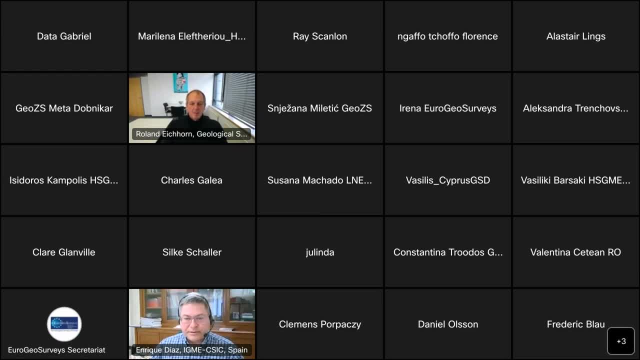 Um, He is from the Bavarian geological survey and please, if you're interested, you can. we will open mics later. for after all the 3 presentations, I think it's better to 1st have all the 3 presentations and then respond. If you want to ask anything directly in written to the speaker, you can put it in the chat. mention who the question is directed to. 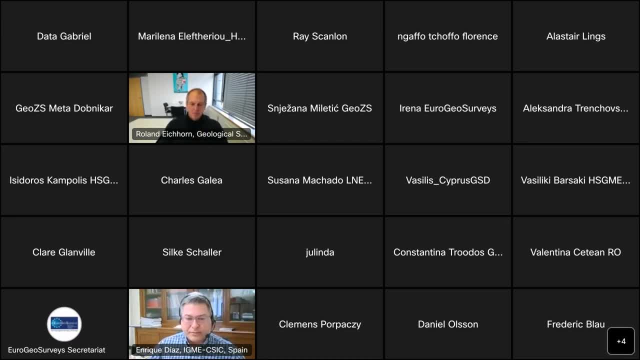 And then That person, the speaker, will try to respond to your questions and, uh, let's start. if you want to share your screen, Yes and thank you. Good morning to everybody. My name is Roland and Ricky has made already the introduction from Germany, Bavaria. 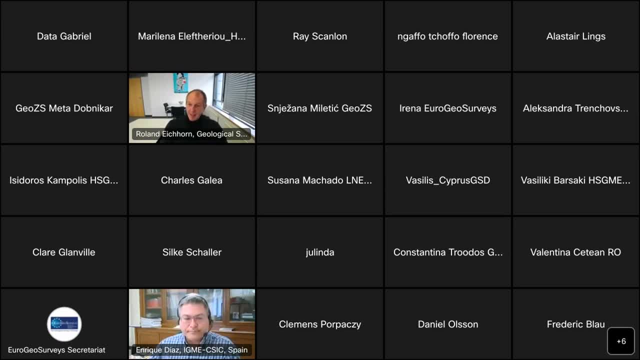 I'm the head of the geological survey and I have to especially greet 1 of the audience. He is not my. I meant. not only my mentor is now a retired geologist, But, as I might say, he's the Godfather of geo heritage in Germany. 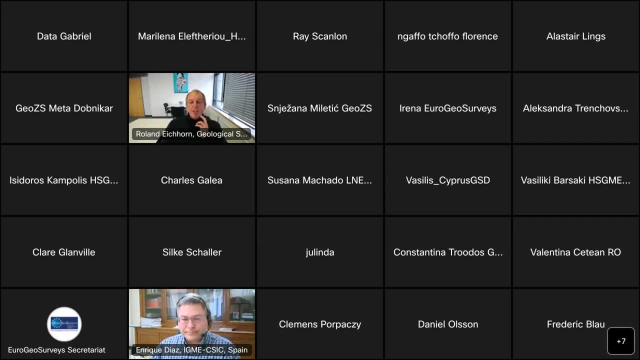 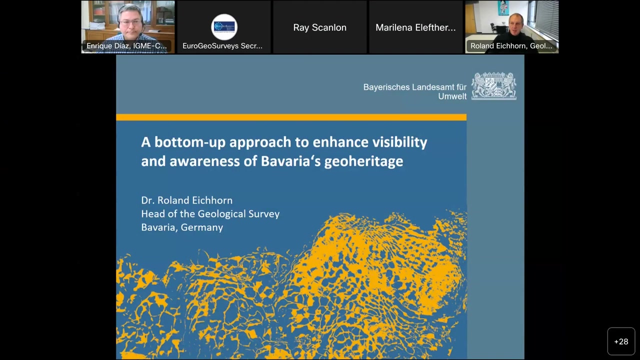 So I'm not sure what I should make the presentation, and not only So. I beg your pardon if I'm totally wrong with our presentation. So I start sharing my screen. So, and Ricky, can you give me a sign whether you can see the screen? 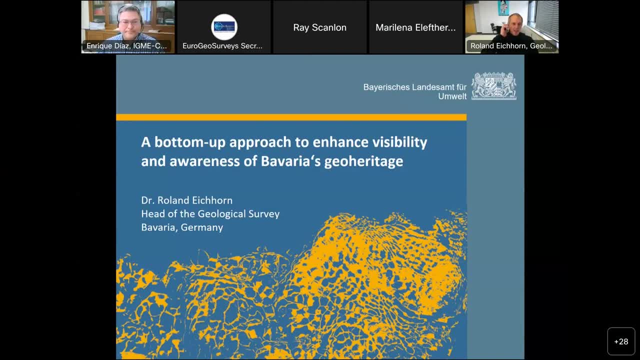 All right, so here we go. It's a complicated title, a bottom up approach to enhance visibility and awareness of various G heritage. To put it in a nutshell, it is something like an advertising campaign. Why are we try to promote the geo heritage inventory? 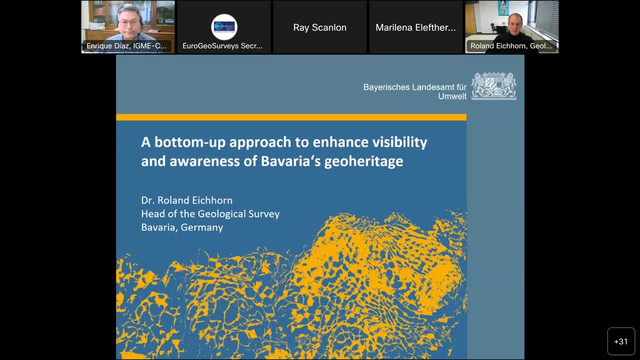 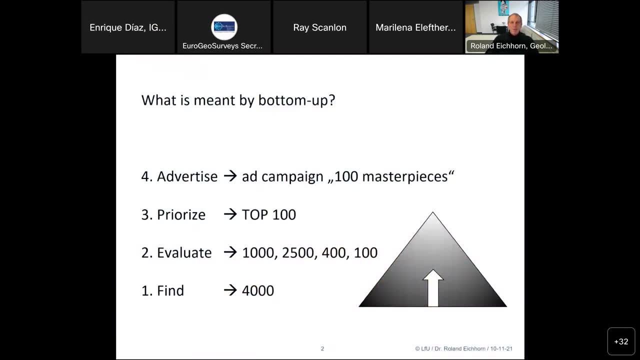 Okay, And how we did this. I'm going to talk about, 1st of all, what is meant by bottom up. We have to start in the line on the bottom. 1st, We had to find All the geo sites in Bavaria. 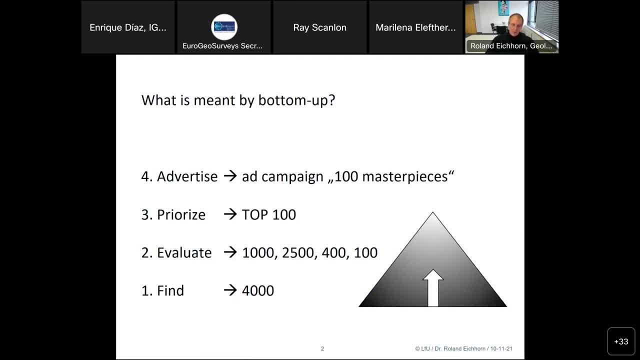 It had been 4,000. and from there, from that bottom Of the, this was our foundation, so to speak. we had 4,000 geo sites And now we had to invent a procedure. How can we promote these geo sites? And I will give you away from point 1 to point 4.. 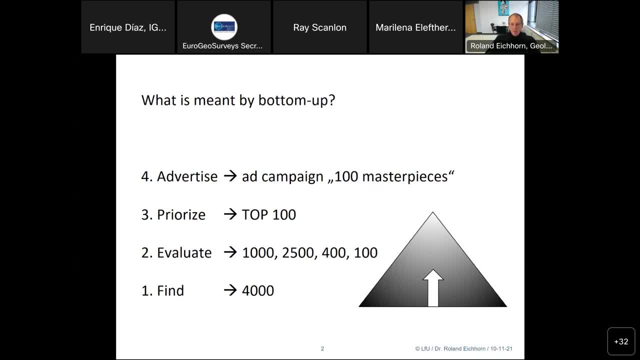 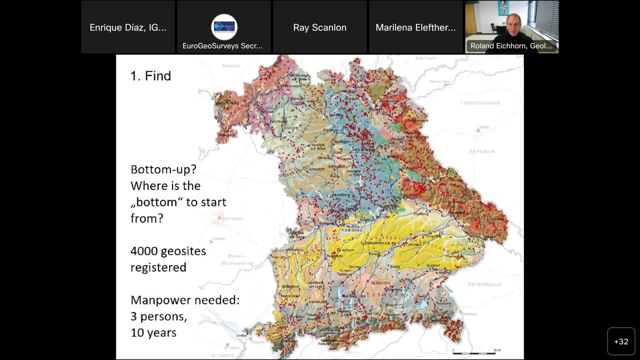 How we can make a campaign to Promote the need for protection Of 2 sites, and we will start by 1.. 1st, if we want to make a successful at campaign, You have to know what is on the bottom. That means how many geo sites or what is your geo heritage inventory. 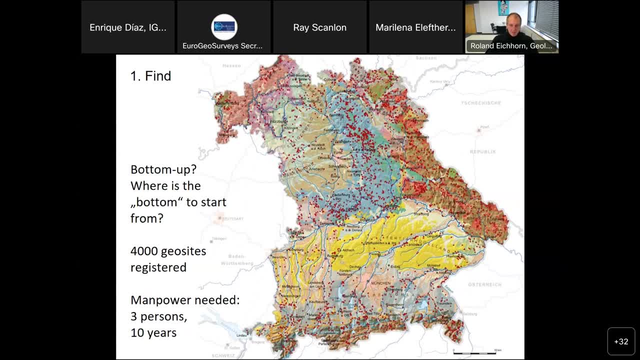 We did these for at least 10 years. We needed manpower- 3 persons- And You can see here the outline of Bavaria and in the background the geological map of Bavaria, and it is very obvious That all the red dots are geo sites, but they are not. 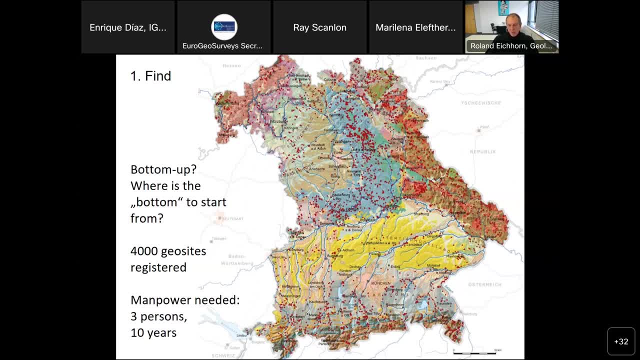 Scattered, I would say partially. There are regions. I'll show you here these Area in yellow. this is essentially only sand and gravel, So In my opinion, very boring. You can't find so much interesting geo sites Down in the South. they are beginning: the Bavarian alps and of course the odds with the mountains. uh show a very beautiful landscape. 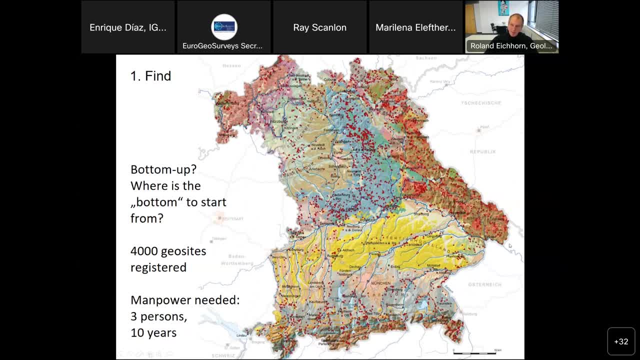 We do have here in the brown red area On the East- these are lower mountains, the Bavarian forest or, Which is also very beautiful, And We do have here in the middle blue. these are to rest Cars like area. there are a lot of. 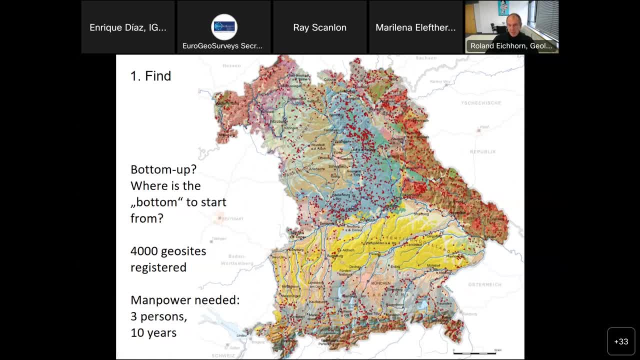 Geo sites, but these are only some uh land forms and uh caves, So it is, let's say, um, only a very Special kind of cheers, Okay, Well, we do have the bottom. now What we have to do, we have to evaluate. 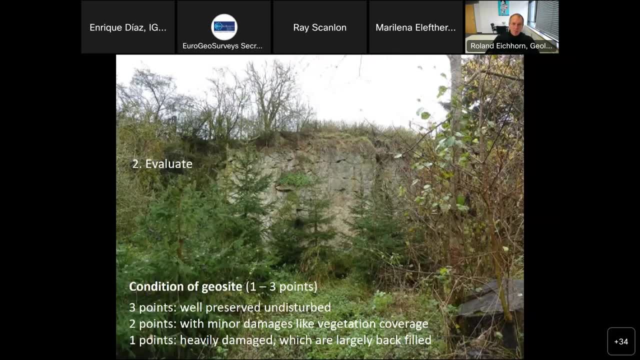 All the geo sites in order to get the most precious ones, the most valuable ones, into uh uh knowledge, And this is 1 parameter we used for the evaluation. The condition of, And as you may well see, this is a quarry where a lot of Christmas trees are growing. now, hopefully, in 3 weeks, all the Christmas trees are away. 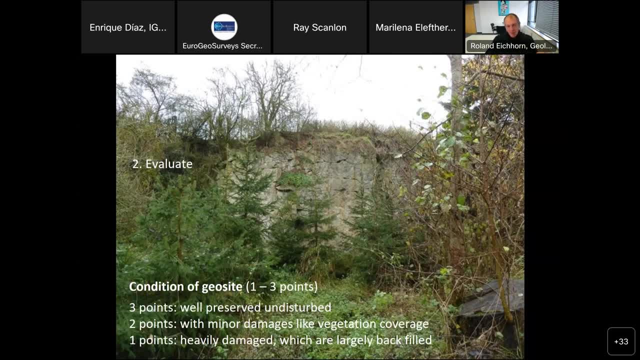 We will see. but now, if you want to get to evaluate this special quality, I would say 2 points would be okay, because it is not well preserved, Not very accessible now in that condition. But it is also not heavily damaged, because if you cut the trees 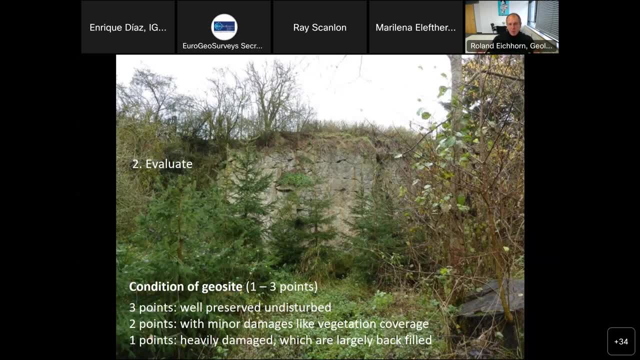 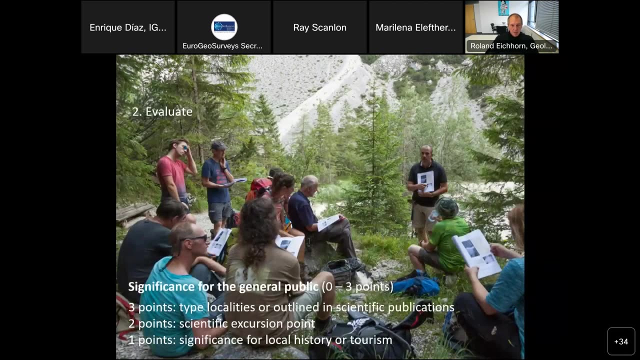 And you clean the area, then you will have a very good quality, a very good wall. So For this parameter, I will give 2 points, only to give you an idea how we did every and each geo site Very right. A 2nd parameter, only to give you an idea. 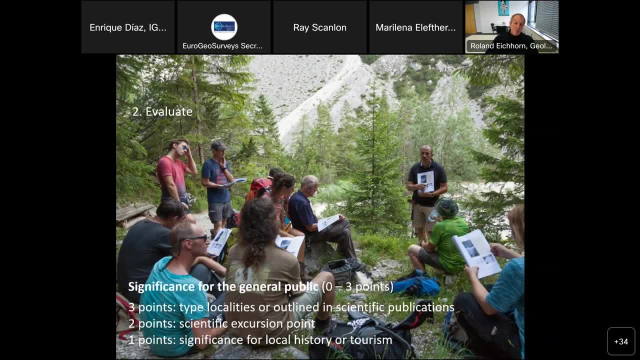 The significance for the general public. We invented 3 different categories. Therefore it is a type of, Or it is in a scientific publication that is prominent in the scientific publication. We will give that to you. Only 1 point, If it is only for the local history of a tourist in. 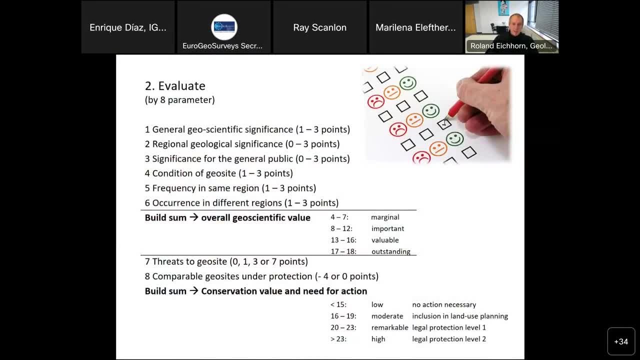 Okay, if you do that Now it's starting to get complicated. We went to 8 parameters, The general to your scientific significance. only to give you here an idea, that means How many sectors of sheer scientific Um work is. 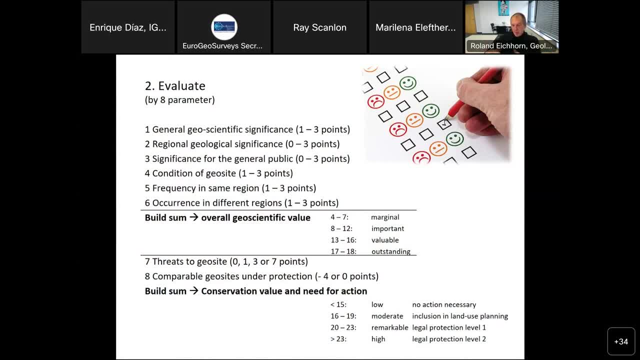 Um, uh, Covered by this, she goes out. Let say it is important for crystallography, for geophysics or for paleontology. the more the better. Then, regional geological significance: significance for the general public: condition of the geocyte, frequency and occurrence. 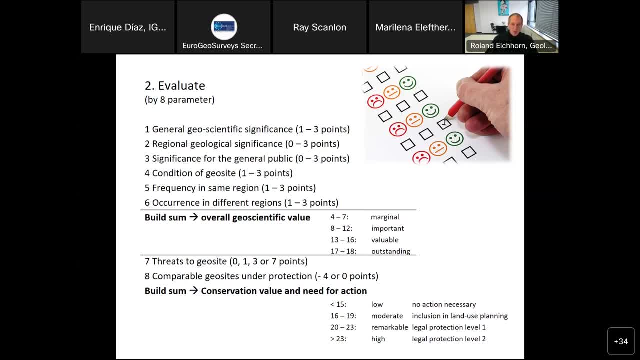 You get the idea, Then you build a sum and you have the overall geocyte, the scientific value. And after evaluation of the geoscientific value, we took it a step further because we want to know whether there are threats to the geocyte or comparable geocytes under protection. 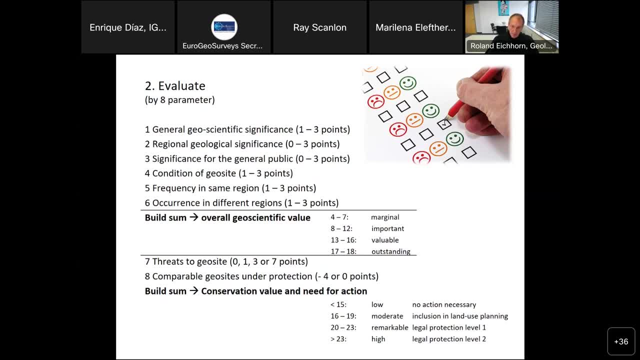 And then you get the overall sum. With this method I think we had a very good estimation. not really objective- it's still subjective- but far better than only describing with words the significance of a geocyte. Because if you want to go into legal business, 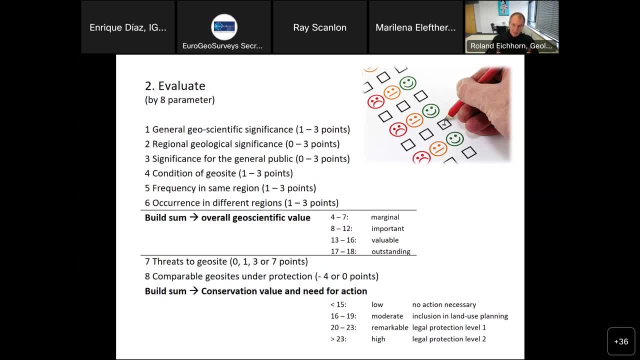 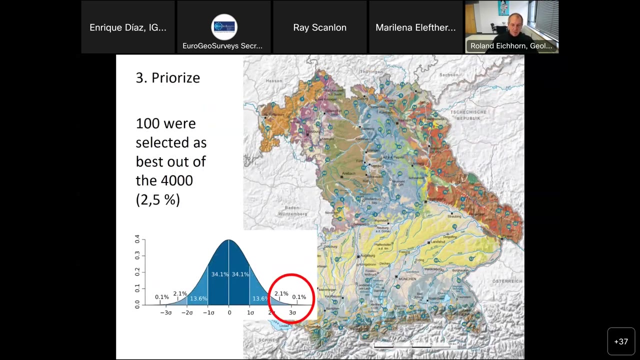 it's always better to have some clear data numbers. This is our experience over 30 years of geocytes protection. Numbers is far better than only words. Well now, if you had evaluated all the 4,000 geocytes, this was quite easy to prioritize them. 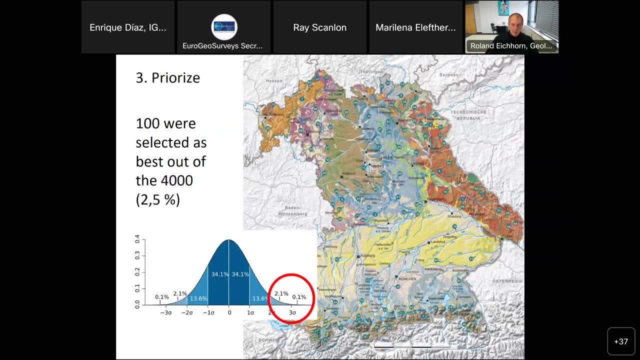 because we had some kind of a Gaussian distribution of all the 4,000 geocytes. Statistically, this is what you might expect, what you get, And we took the two sigma, three sigma percentage of the best ones, And these were about 2.5%. 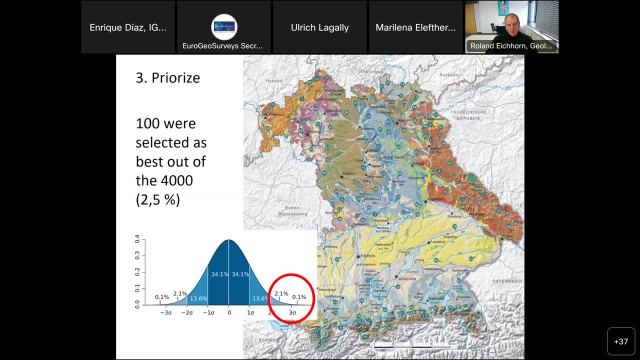 So this is only an estimation, Because we we thought about what kind of how many geocytes we want to put into our advertisement campaign. Now, while the number 100 is a funny number, you can take 111 or 99 or whatever you want. 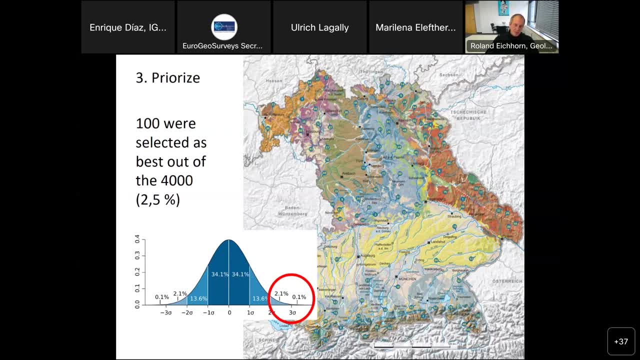 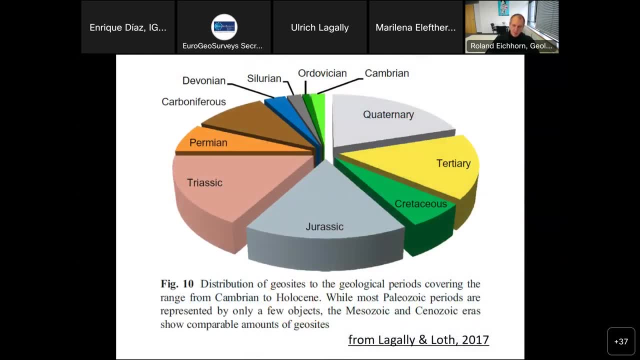 We thought about. 100 is a clear and distinct number. This is only for orientation is to see. you can have it from a paper by Lagali and Lod. We in Bavaria have. we are very lucky because we have a huge portfolio of geological periods. 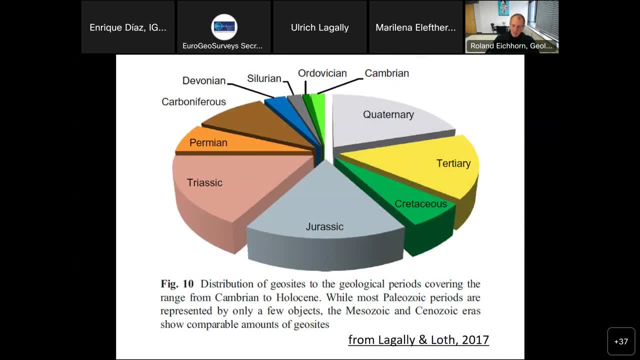 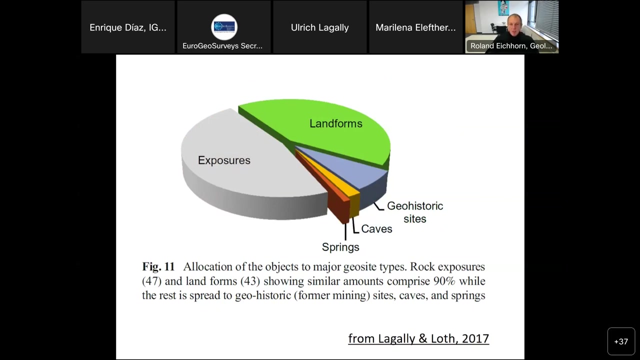 Practically all the periods of the geological past can be covered by geocytes in Bavaria. Of course, the older they become, sell them, But this is only for you as orientation. The same thing is true with this pie chart. Most of the geocytes are landforms and exposures. 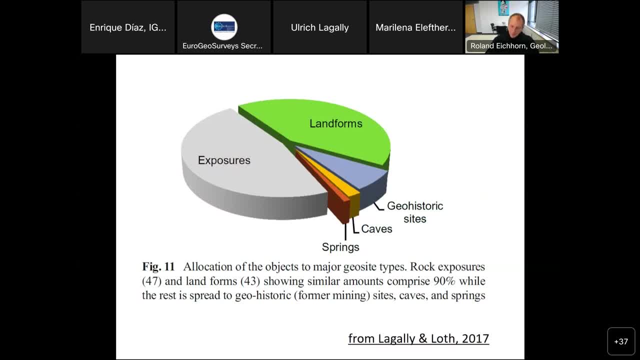 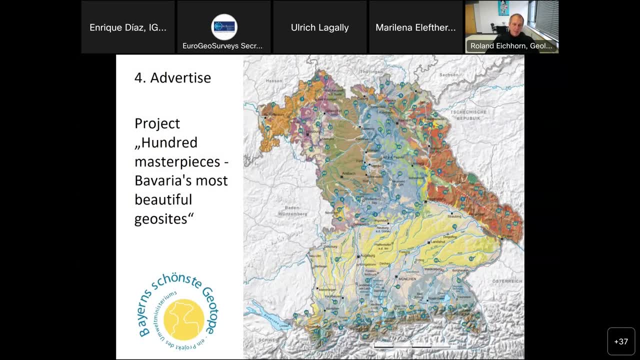 which is quite what you might expect. let's say, All right, if you had done that, Now it's start the advertising campaign. We invented a name for our project- 100 Masterpieces, And we created a logo for Bavaria's most beautiful geocytes. 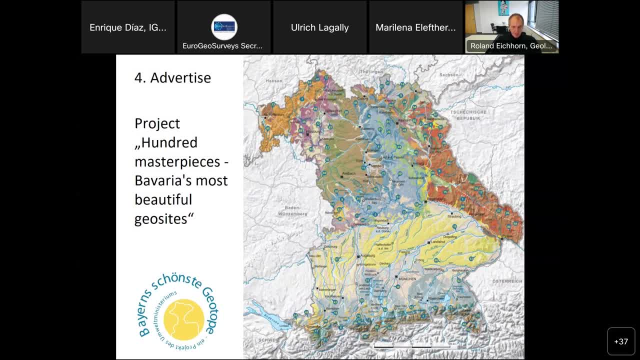 We made a logo which you can see on the bottom left And you can also see once again the outline of Bavaria and where the 100 geocytes which we want to add in our campaign are located And you can see. we also focused on the effect. 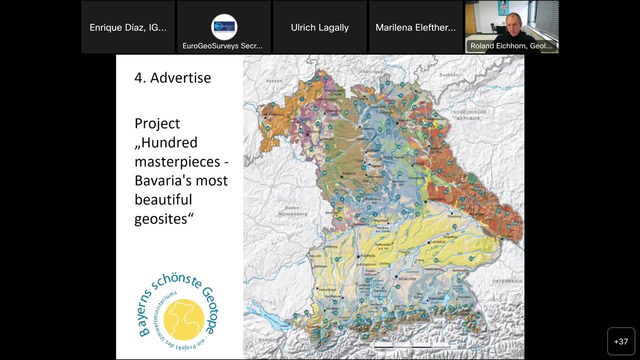 that we want to have them scattered all over the country, So that we even, as you remember, the yellow area with only sand and gravel does not have so many geocytes. We at least wanted a few of them located within that area. So what do you have to do if you want to successfully? 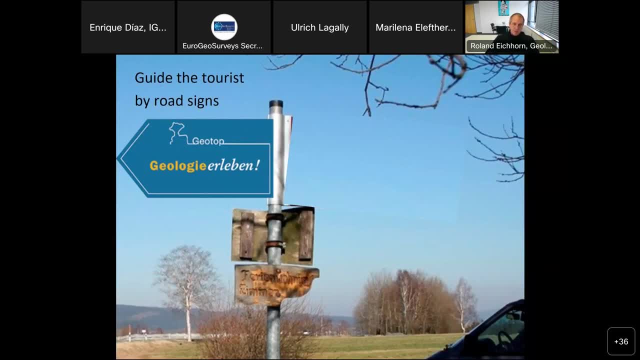 make an advertisement campaign, First of all you have to know. you have to show the direction to any tourist or hiker. You have to show the direction. So we invented a road sign, which is quite easy. I like the color blue, like Uli Lagalle as well. 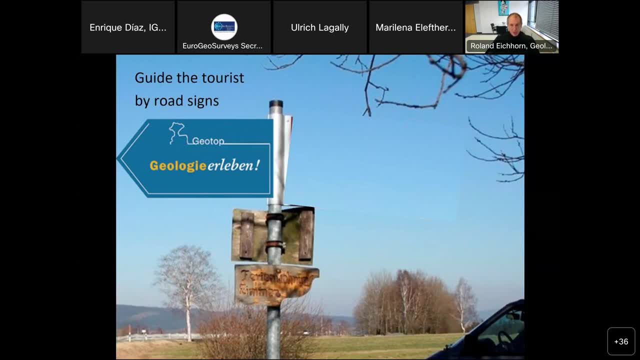 So we made a road sign in blue and we put it on a traffic pole where all the other signs were as well. But- and that's the first step- Bureaucracy is overwhelming. So my first advice: first ask the road authority for permission. 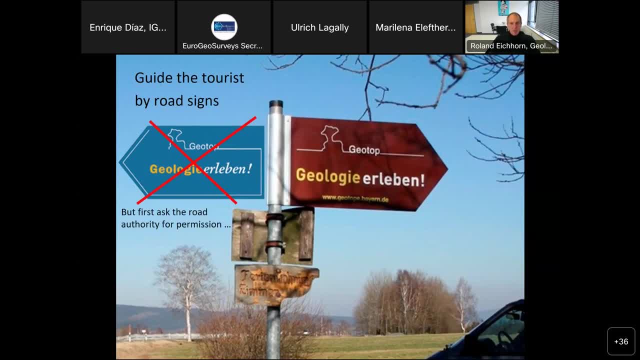 because we learned it the hard way. You can't simply put a sign on official road pole and you can't use a color you want. In Germany it is obligatory that the color of a road sign is in brown if it is touristic. 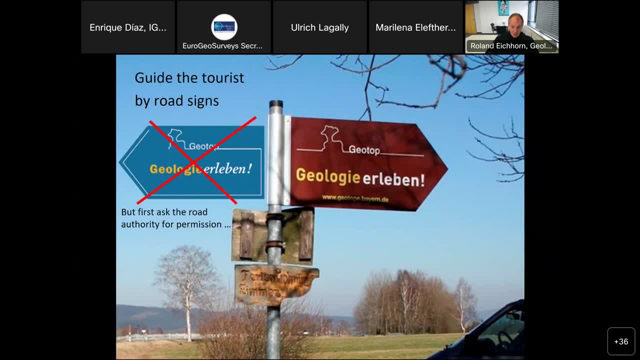 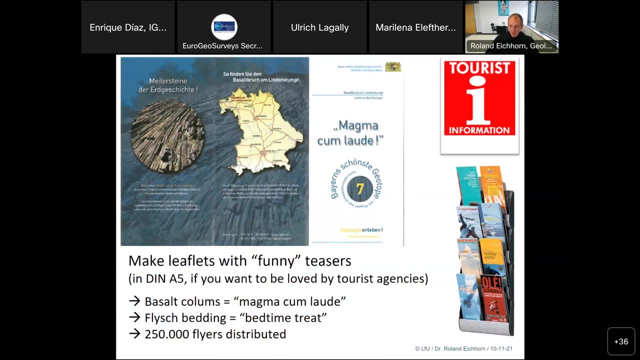 So, 1st advice: ask permission. 2nd, not only the road sign is important. If you have a tourist, you should place some advertisement, Let's say leaflets, In the tourist office. so we made 1, which, by the way, is important to have it a 5.. 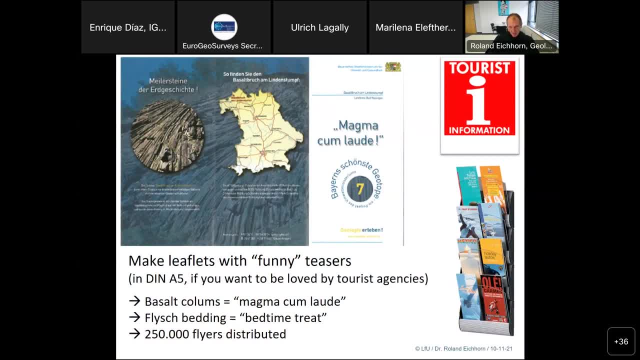 Then you will be loved by tourist agencies because, you see, most of the leaflets will go into some kind of these. How to say this leaflet giveaway- Uh, I don't know the English word for the thing on the right side, But I think you know what I mean. and then it was for us a very good idea to make a very funny teaser. 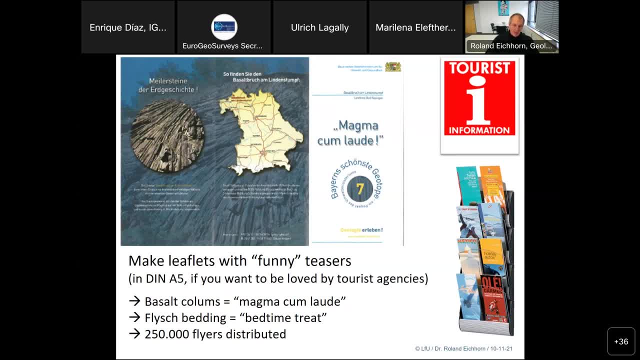 Uh, this is very difficult to translate in a foreign language. So let's say the flesh bedding. we had a geo side with fluish and they have a very good layering of bedding. So we don't tell it as we don't say: this is fluish bedding, but it's bedtime tweet. 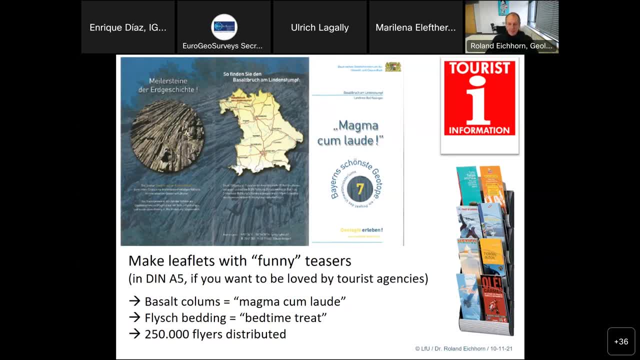 Or the it's called or something like that. So this is funny and, uh, few of the tourists think, uh, they want to know what the funny uh teaser is all about. And at least we, we are quite successful: uh, a quarter of a million. 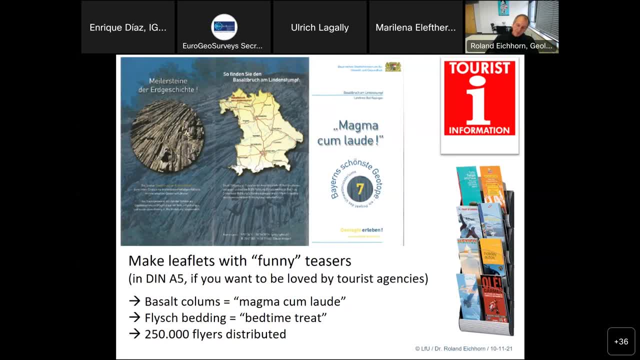 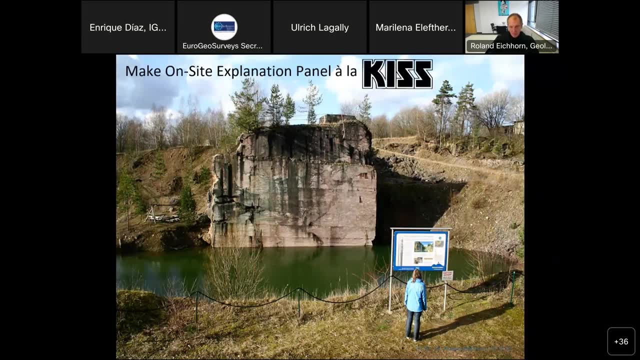 Uh, a quarter of a million. Uh, a quarter of a million. A million of these flyers have been distributed over the time. So if you had all that, it is. the 3rd, very obvious part is that you have to make an onsite explanation, handle a la case. 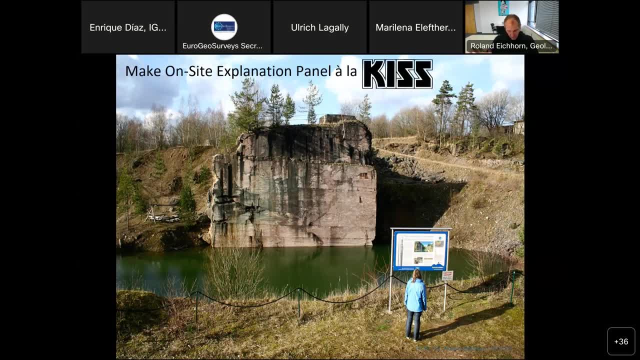 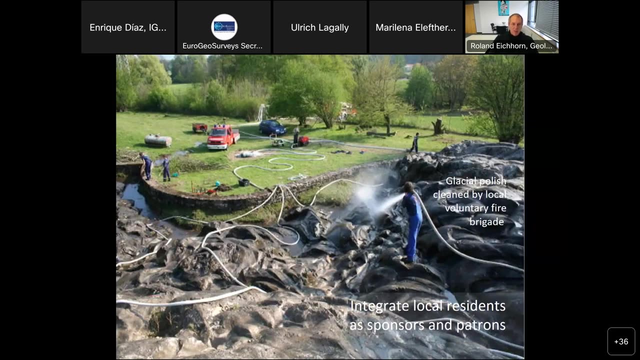 The, the rock band I'm very fond of, But the method. the method is keep it short and simple method. And now, this is probably the most unusual and the most successful part of the whole campaign, because the 3 things: uh leave a flyer, uh a road sign and the panel. Okay, Everyone knows that he has to do that. 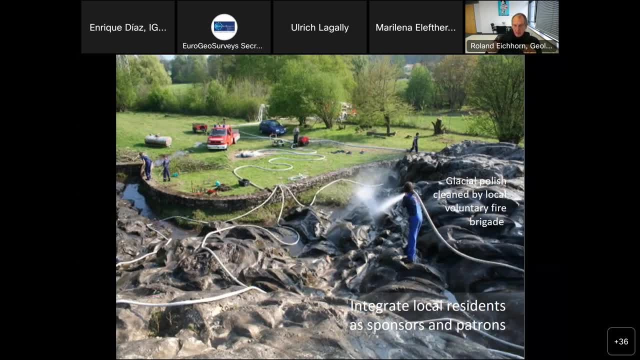 But now this is essential. we had the idea that we want to integrate the local residents As sponsors or patrons of the geo side. Here you can see a picture. this is a glacial Polish and it is clean by local voluntary fire brigade. 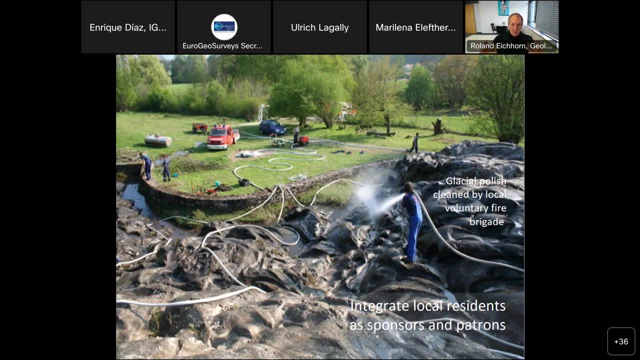 And if you do that now, suddenly the neighborhood is really interested in the geo heritage in the neighborhood. They are very proud of the geo side And then, um, it's far better uh as uh compared to Doing it for yourself as. 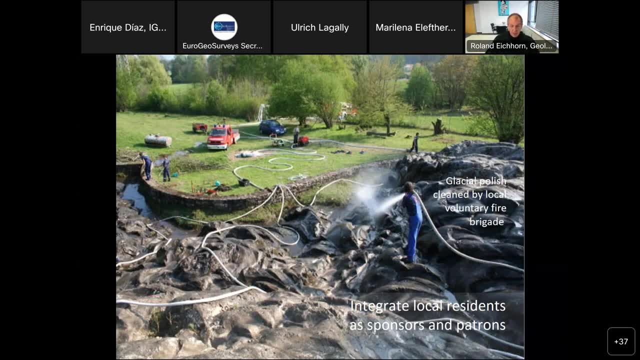 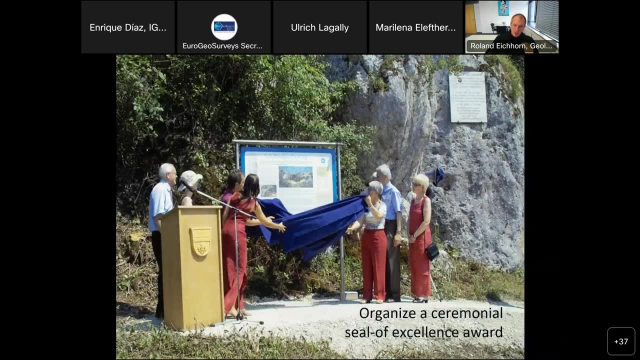 Um office as as an administration agency. This was very essential, and if you do that, then you should also organize a celebration, Organize a ceremonial- let's say, seal of excellence or what That means- if the sponsor or the village 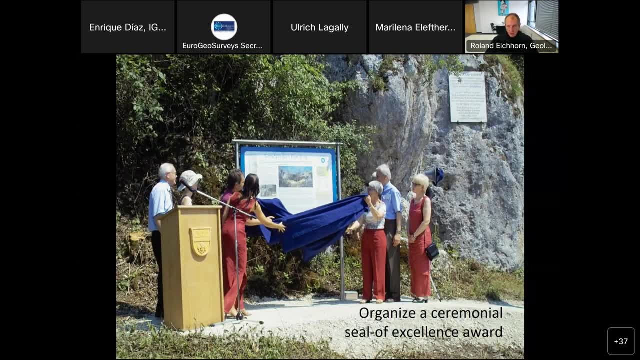 Which wants to protect, to the geo side, which wants to, uh, wants to keep the geo side clean. Give it um a seal of excellence, and the seal of excellent can be promoted by, let's say, a minister, Or um a very famous person. 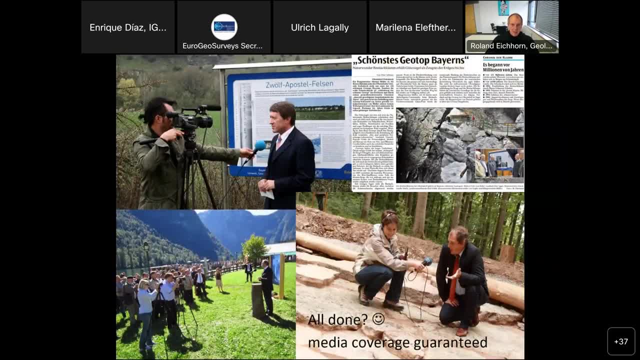 If you do that, media coverage is guaranteed. we had about 1 to 2000. media coverage is informed from TV or radio or articles in newsletters. This was a very, very huge Success and because it was so huge, We can say that in Bavaria that geo sites are now really renowned. and well no. 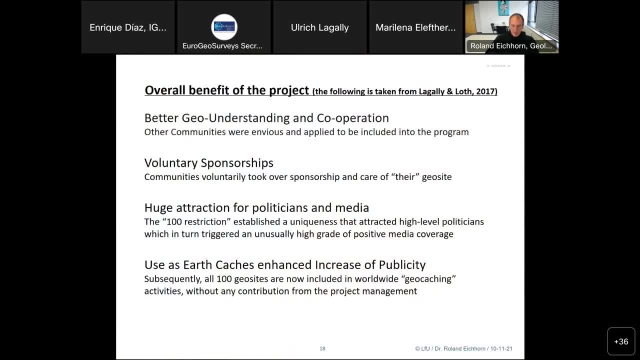 So no further pictures. Let's come to the overall benefit of the culture. First, as I already told you, it is a better understanding of the necessity For the geological heritage, and we uh um Experienced a huge cooperation between our geological survey. 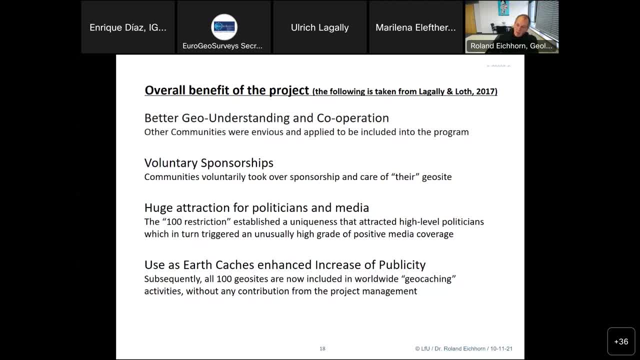 And the sponsors and patrols, uh, in in the neighborhood of the. It goes so far that other communities, even the envious and wanted to be included into the program. This was this. networking Is now far better as it was Before we started the. 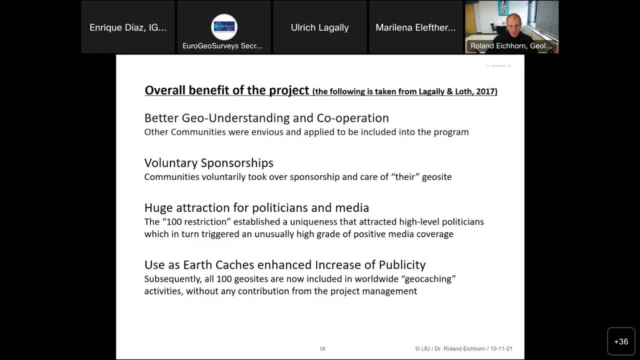 The voluntary sponsorship is, of course, the the most successful aspect Of the whole ad campaign, because now they care for their And it was a huge attraction for politicians because, as you know, if you have media coverage, a politician is very near. 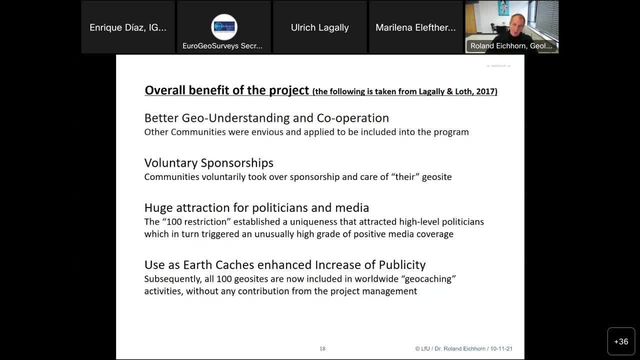 And these attraction to high level politicians In turn, so we get an unusual high grade of positive media coverage. It was a self fulfilling prophecy and This wasn't uh, let's say, a bike catch uh the uh, they uh discovered our 100 geo sites and they are all now included in a worldwide geocaching activities without any contribution from our project management. 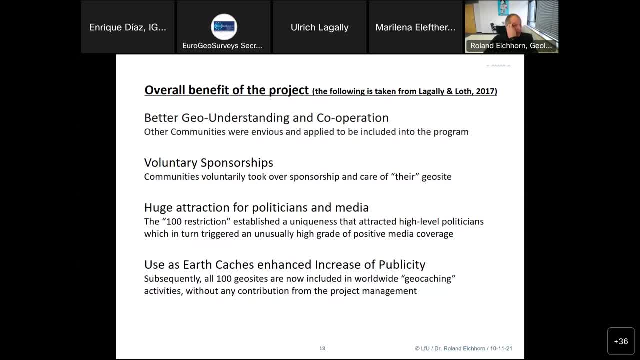 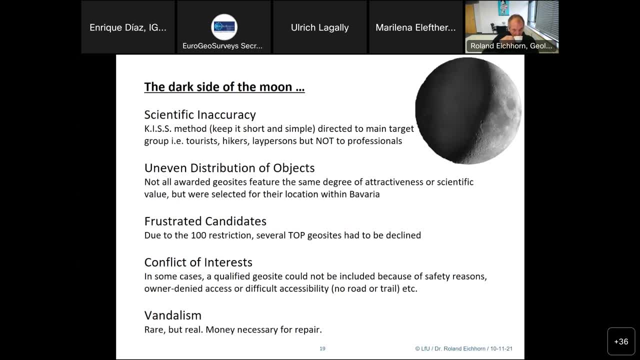 But where there is light, There is light, There is light. There is also the dark side of the moon. The case method, of course, Has to be scientifically accurate, Because we focused on tourists, hikers and lay persons, and not professionals. 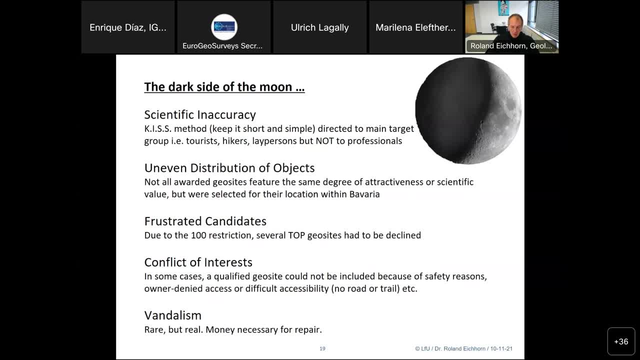 That means with our information alone. it was not possible for Students geology To use that spot for their excursion. they had to have more and further information. So we had to accept that that it is really only for Lay person. it had been an uneven distribution of objects. I already told you that We can't do. we can't. 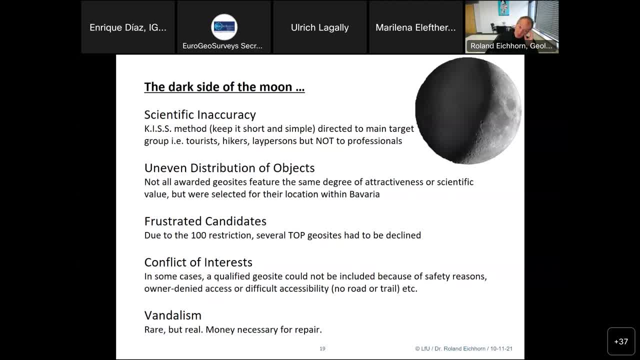 Invent a new geology. Yes, There had been a few frustrating candidates. Yes, We had to say that, But Yes, we had to say that, But Yes, We had to say that, But We had to say that, But. 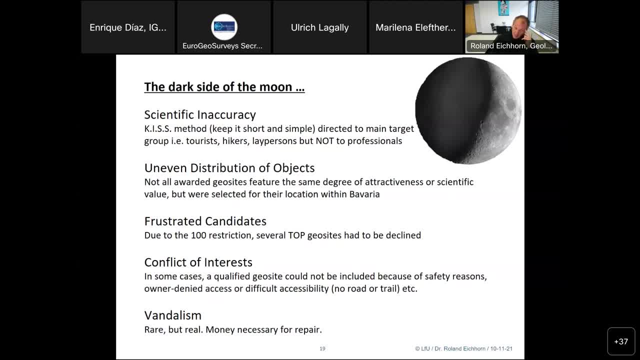 We had to say that. but it was absolutely necessary to fix the number of top geosites. If you open it up and say no, now, 10 years later- let's say we found now 130 top sites- you make you a little bit unbelievable. 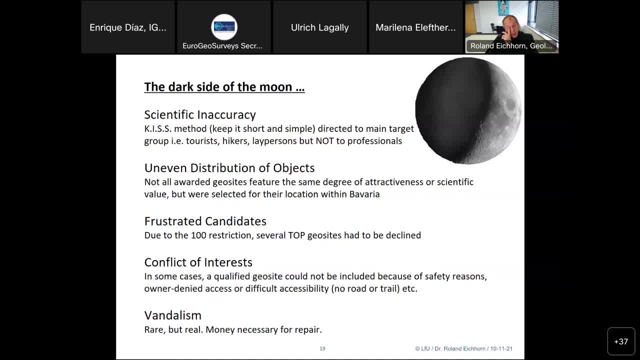 Conflict of interest. In some cases we had. we would had really really integrate. we wanted to integrate a few of the top geosites but it was not possible due to safety reasons, because it was a very dangerous area or the it was privately owned and access denied, or there had been no roads. 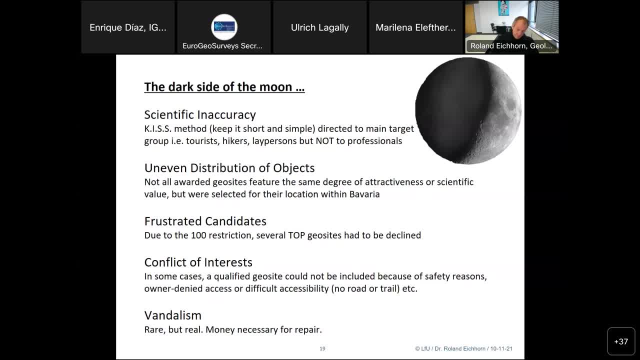 or trails to go there? Yes, of course, And yeah, That's crucial. But the reality of today, vandalism gravity, is rare but real. To give you a number: from our 100 geosites, at least two per year have to be repaired. 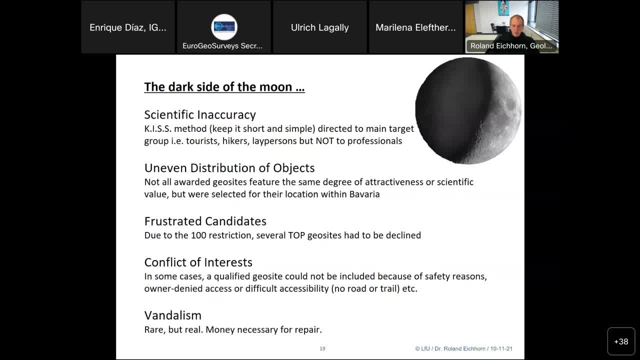 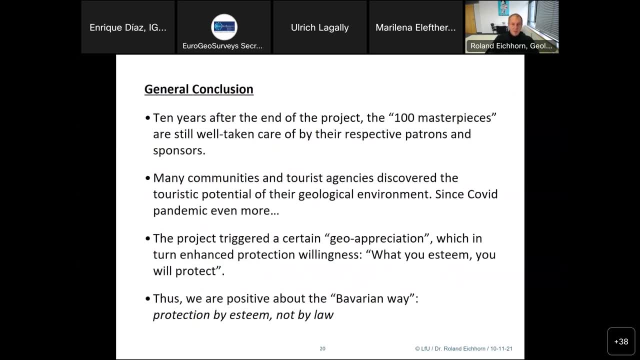 So you need not too much money, but you need money to make it clean again or to repair it again. So last slide to sum it up, general conclusion: Ten years after the end of the project, The 100 masterpieces are still well taken care by the respective patterns. 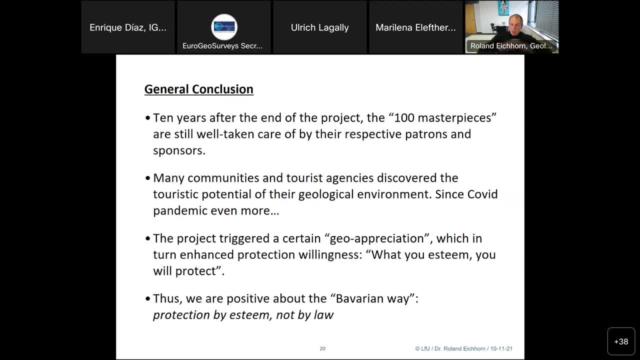 Many communities discover the touristic potential of their geological environment. And yes, the second half of that statement: since COVID pandemic, even more. yeah, that's true, Really, we had a tenfold increase of telephone calls or emails because during the pandemic, 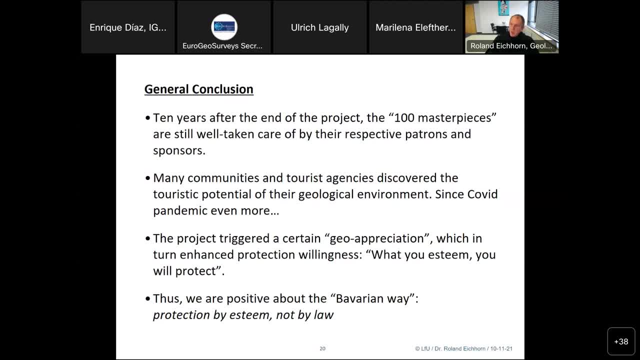 a lot of people Can't go to their worldwide travel in summer holidays. but they bought a e-bike or mountain bike and they tried to discover the neighborhood. And then they stumbled over our, over our geosites and started to get interested in. 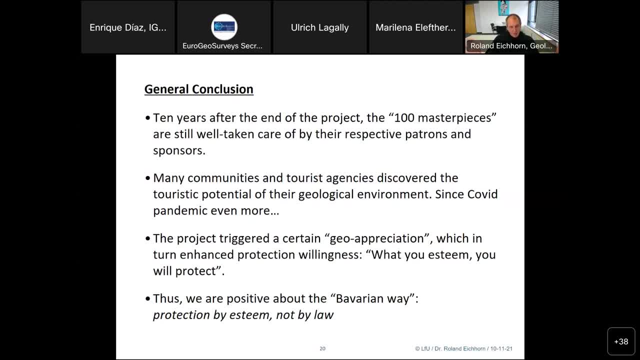 geosites. So This was one of the few positive aspects of the pandemic, if any. Yes, of course The project triggered a geo appreciation. It is very important, but everyone who is in the business knows that only what you esteem. 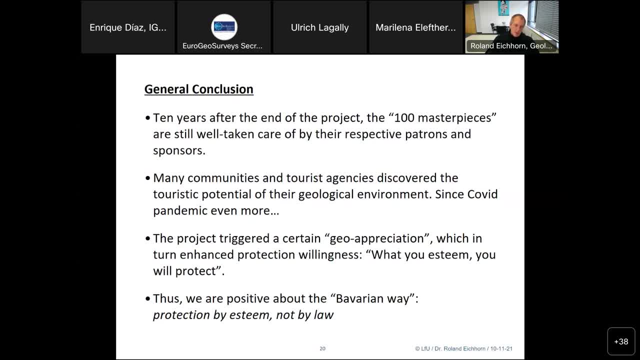 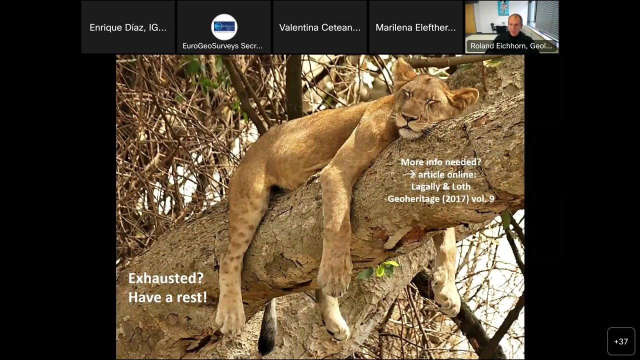 you will protect, And this is the most. put it in a nutshell, this is the most important conclusion. We think that it is that you are more successful if you can protect by esteem and not by law. I think So. if you want to know more, there's an article online. you can Google it in geo heritage. 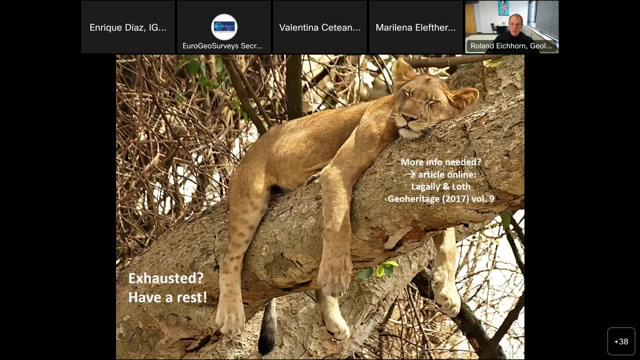 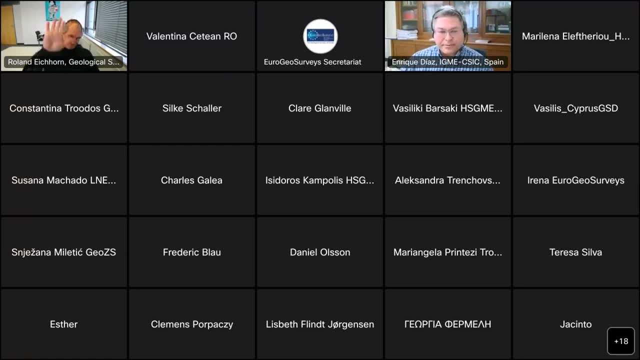 Thank you very much for your attention. I close the screen and been open for discussion. Thank you, That's excellent. Uh, thank you very, very much, Roland. Very good, I'm sure that there there will be Uh. 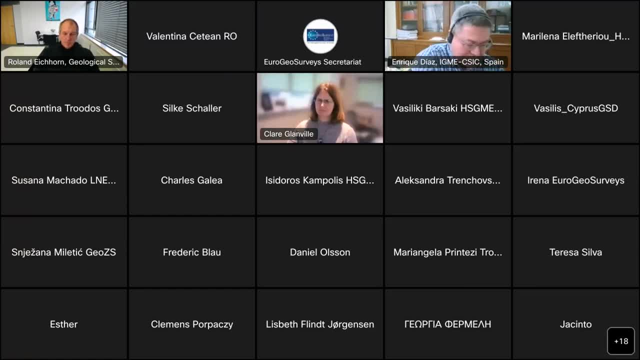 Uh, There will be a lot of interest, because it is always good to learn from the good and from the bad experiences. I mean not that your experience is bad, but from you. know what I mean. it is better not to make mistakes. 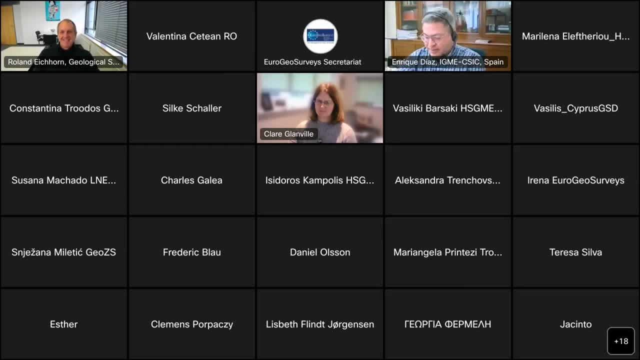 And it is the best thing is when somebody recommends: don't do this, because then you, you don't know what consequences can be and all these things. This is excellent And to To learn, To learn from from others, and uh, now we will have uh the talk from uh uh Claire. 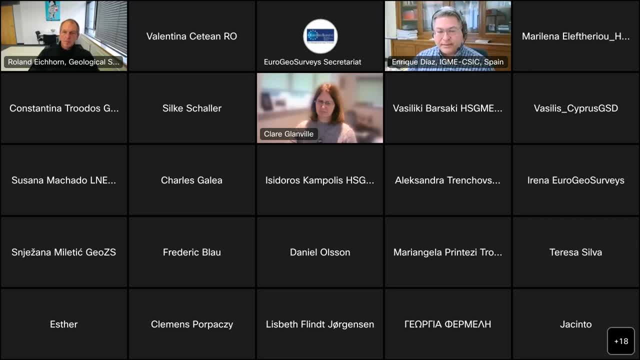 Glanville about county level audits in Ireland promoting and protecting the local geo heritage. If you can, Uh, share your screen, Okay. Thank you, Enrique. Um, Just bear with me when I share my screen, Okay, Thank you. 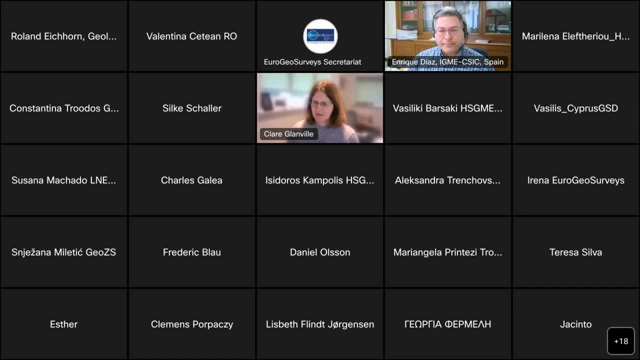 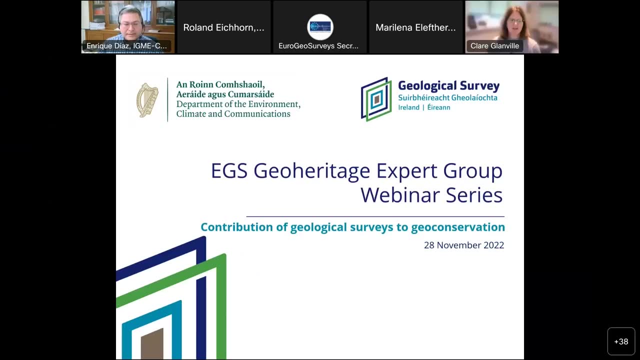 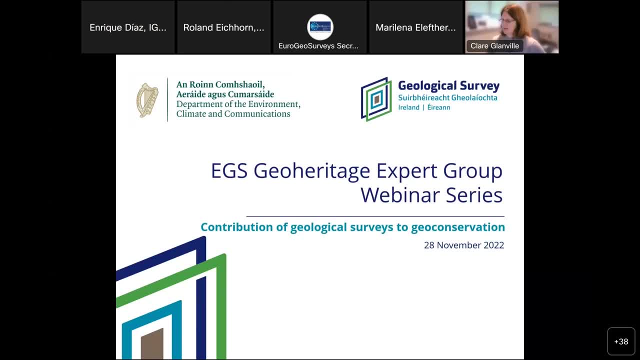 Yes, can you see my screen? Yes, yes, Okay, that's great. So my name is Claire Glanville and I'm the senior geologist with the geo heritage program at the Geological Survey Ireland, And likewise, I'm very glad to be here for the first of our eurogeo surveys- geo heritage. 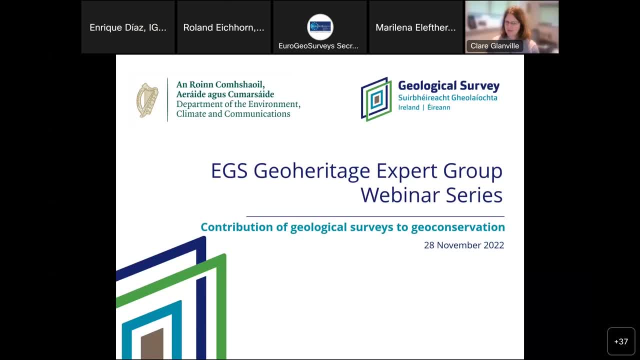 geo heritage expert group webinar series talking about the contribution of geological surveys to geoconservation, and this is just the first of a number of them, so I'd like to welcome you all as well in that respect. so I'd just like to talk to you a little bit about county level audits in 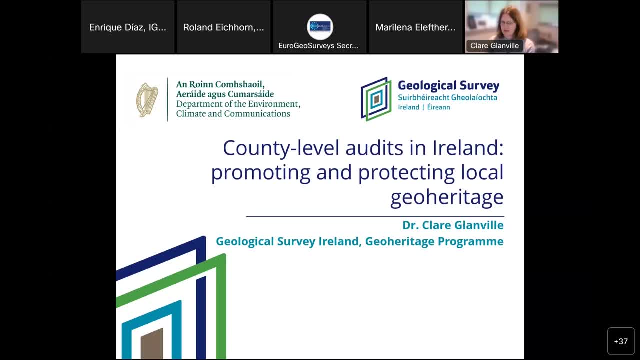 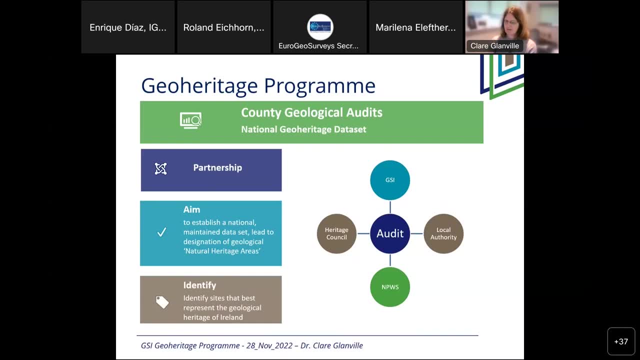 Ireland and how they're used in promoting and protecting local geo heritage. so first of all, a little bit of background about our geo heritage program and the what we call county geological audits. the program was first established in 2004 with the aim to identify sites that should be designated as natural heritage areas, or NHAs, under the EU habitats directive. 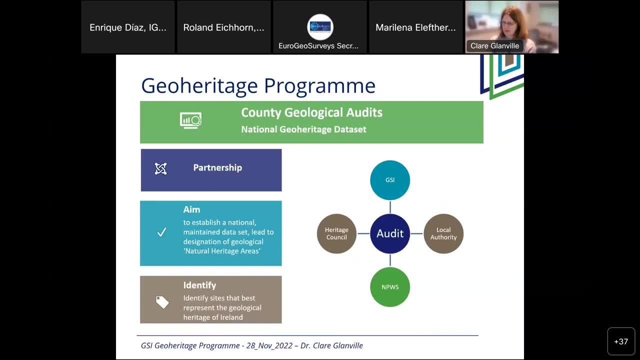 and due to the volume of work required and resources available, soon became obvious that this needed to be a partnership project. so, although the geological heritage program exists within the GSI, we opened the audit process up and just a sort of a partnership which included the local authorities and ourselves, with funding from the geo heritage council. 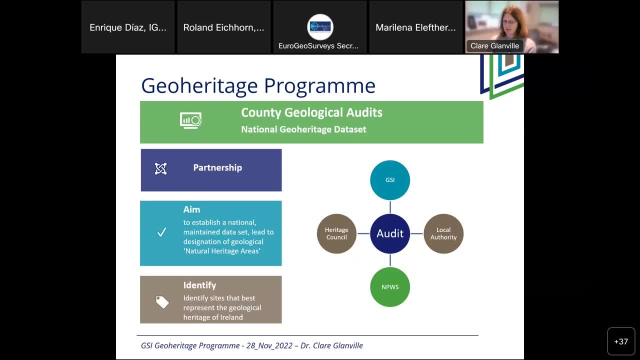 and the national parks and wildlife service also have a role in this partnership. so the aim of the project was to establish a national data set that could be used to support the designation of geological heritage areas, and so an important part of that was first to identify the best represent, the sites that best represent the geological heritage of Ireland. 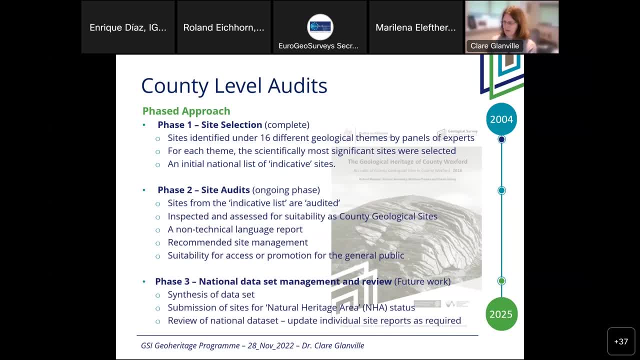 and we took a phased approach, as I said, starting in 2004 with the identification of sites based on 16 geological themes. this was completed very quickly. it was largely a desk based study and focused on the knowledge of the theme experts as well as previously published research. 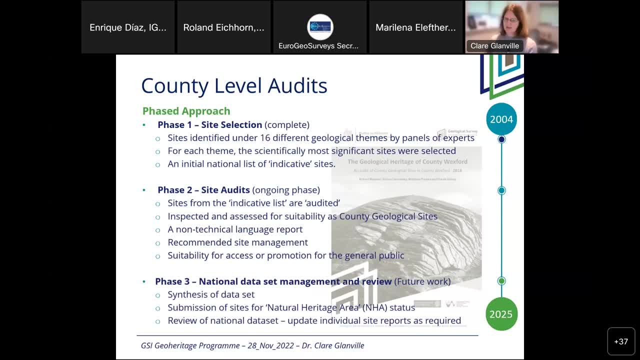 and it led to what we call here an indicative list of sites, of geoheritage sites. the next step was to look at these sites and to audit them. so all of this process is a little bit before where Roland is in Bavaria, where he was discussing the advertising. 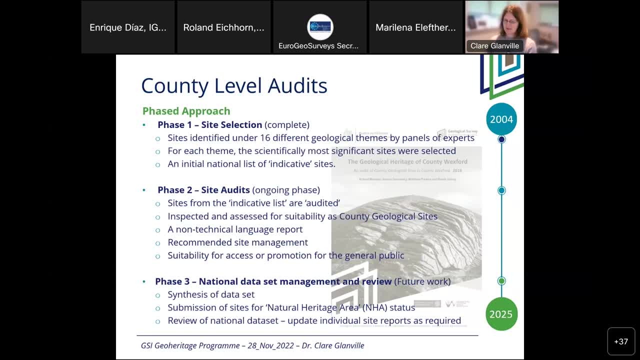 and the evaluation of sites. but our next step was to move to auditing these sites, so sites from the indicative. well, it was done in partnership so it was very easy for us to kind of sort of copy and paste all of the sites and share with the local authorities as well. the planning makes a big part of this project. 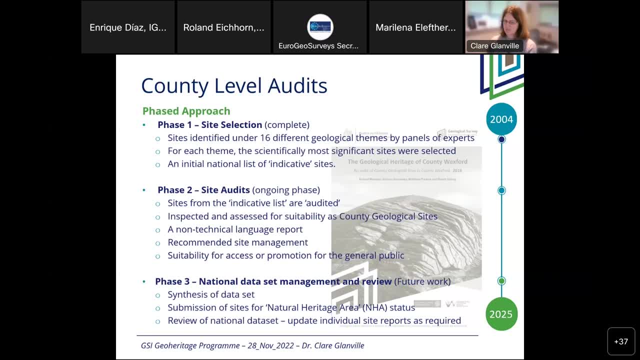 So it was very important to have the local authorities involved. So we did it on a county basis, county by county, working with each individual local authority. as time went on, And so for each county, the indicative list was examined and the sites on it were audited. 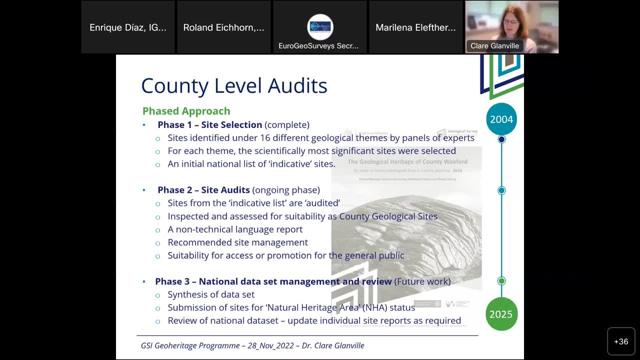 Additional sites were also inspected on a county level, based on local knowledge. So the sites were inspected and they were assessed for suitability as a geological heritage site or county geological site. we call them on this process. A non-technical report is produced for each site and recommendations on management suitability. 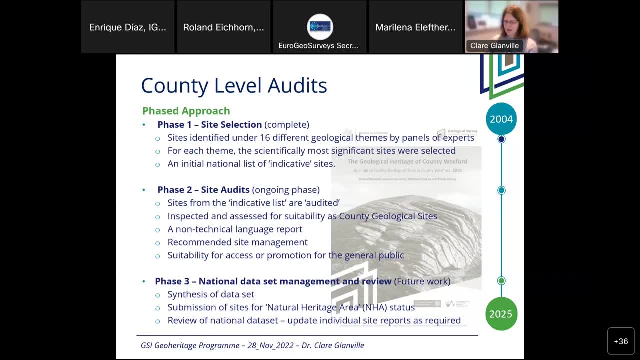 for access, promotion and that sort of thing. The third phase is only just beginning and it's largely future work and probably bears more resemblance to the previous one. The fourth phase includes a synthesis of what's now almost a national data set of geological heritage sites. 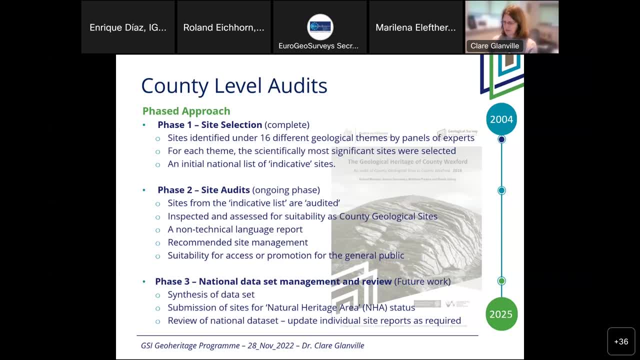 When you combine all the counties together, we've almost completed a national set. It will hopefully lead to the submission of sites for NHA designation, and we'll be working with our partners, National Parks and Wildlife Service, in that respect. And, of course, 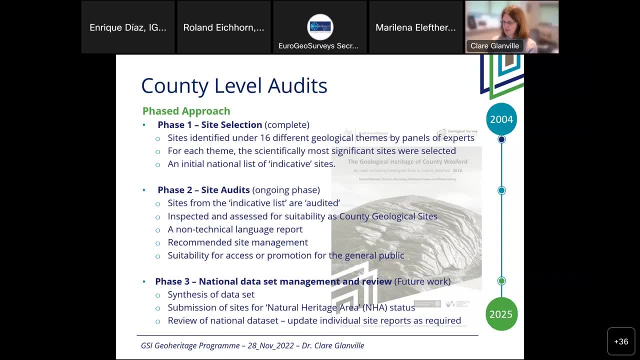 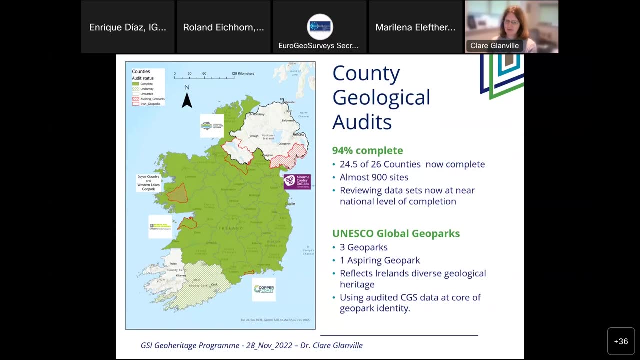 because this process has been ongoing since 2004,. there may be some individual sites that need to be revisited and reexamined, So this just to show you where we are to date. so about 94, 95% of the counties have been. 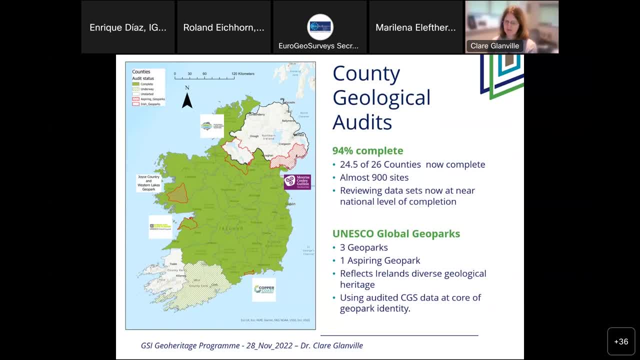 audited. You can see all the dark green areas are counties which have now been audited and there are units of county geological heritage sites for each of those. The pale green area in the southwest is County Cork. that's a three-year audit and we're 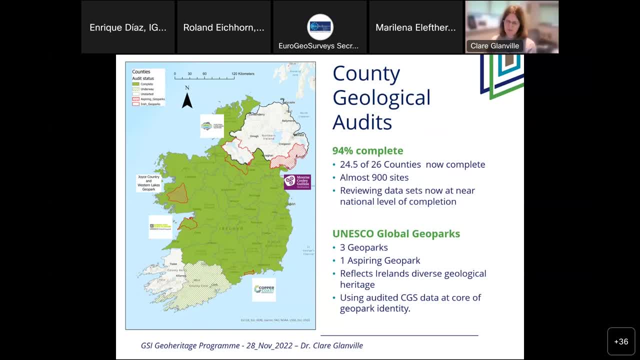 just starting the third and final year, So hopefully that will be audited by the end of 2023.. And Kerry is the remaining county in the southwest which we hope to start next year and will be completed in 2024.. You'll also see on this map I have included our UNESCO Global Geoparks and I just wanted. 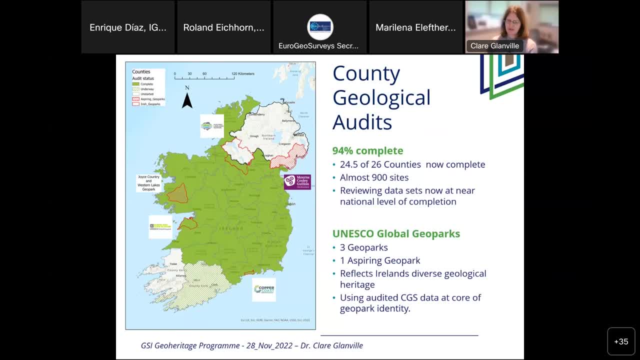 to mention that we have three UNESCO Global Geoparks in Ireland and one aspiring geopark. This reflects the great diversity of geological heritage and geology we have in the country. But the reason I included these here is because the geoparks build on the audited site data. 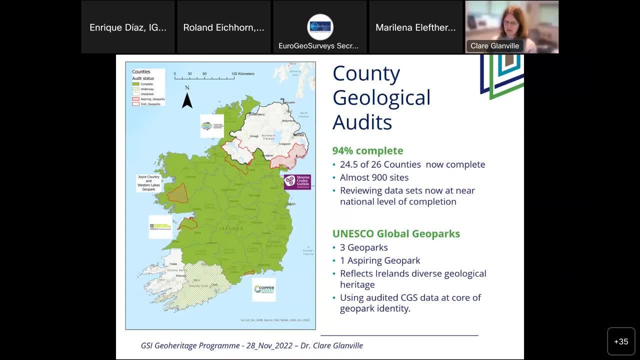 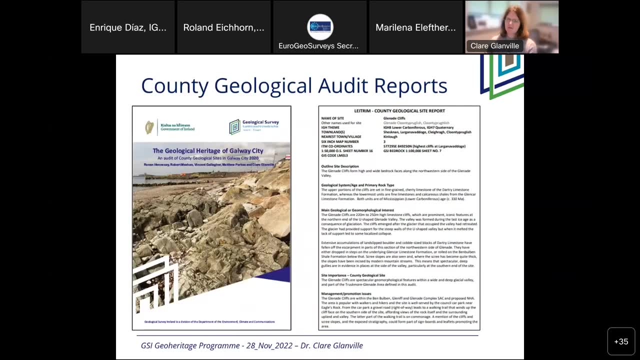 and they use it to develop the geoheritage narrative within their parks, So it's an important part of their projects as well. So when each county is audited, in partnership with the local authority and the heritage council, a county geological heritage report is written. 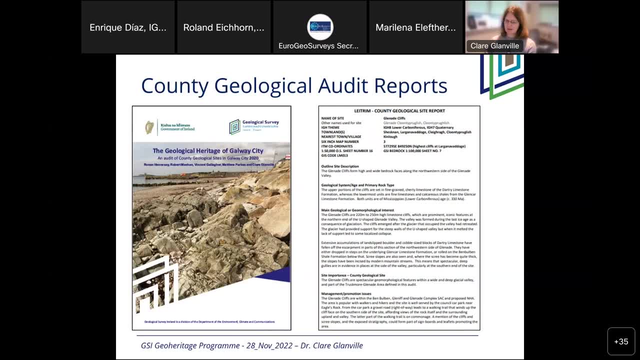 This is a short report, written in non-technical language. Discusses the Geology, the geology of the county and, in summary, talks about the context in which the geological sites are selected. a bit of background about the planning context: promotion. 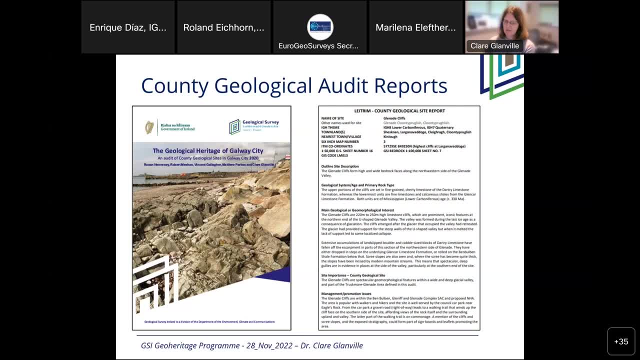 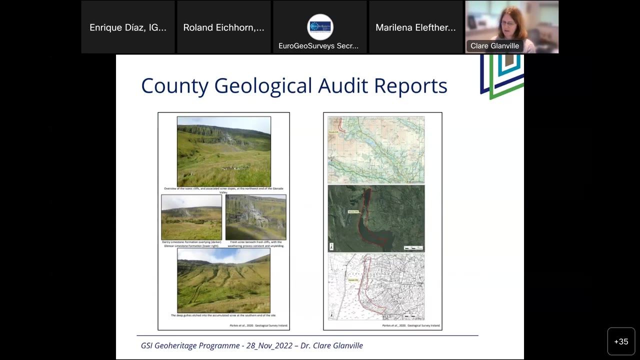 of them and management of them. An important part of each county report are the individual site reports, And so we keep these short, relatively short, Two to three pages. They include some information and also a photographic record, and the boundary of the sites is mapped. 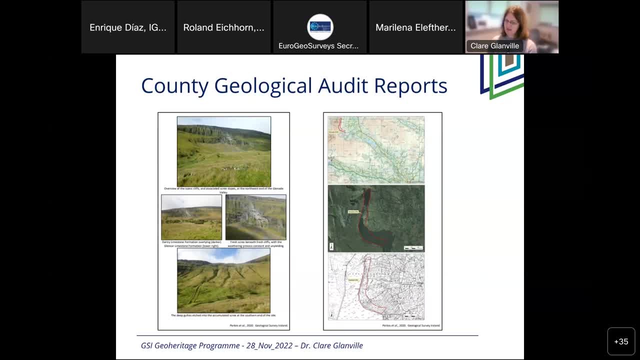 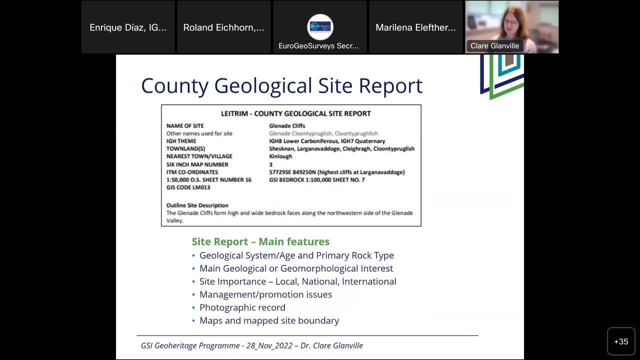 and these mapped boundaries are also available digitally for download as shapefiles or can be viewed on our website at Geological Survey Ireland. And The Transcripts And the Transcripts of each individual site report. They have a short section on the geological system or the age, the rock type, what the 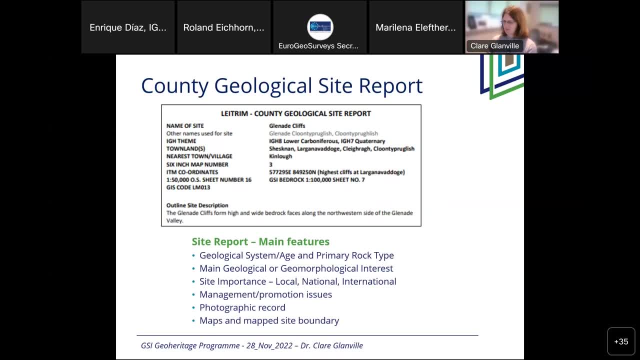 main geology or interest is if it's a landform or if it's an exposure. There's a section on the site importance, whether it's of local importance, national or international, or whether we think it should be recommended for one of these natural heritage. 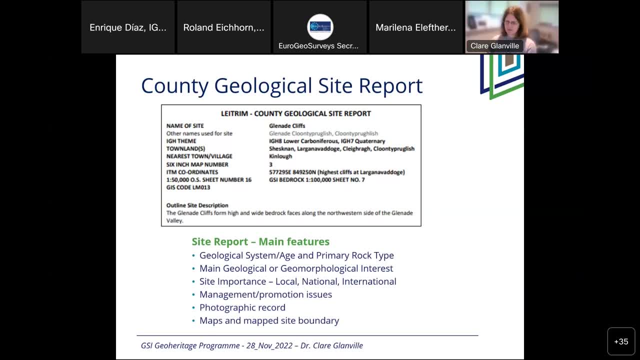 areas under the EU Habitats Directive, Indy course- And It also has a section where we talk about management issues and promotion, what the access to the site is like, whether it's under threat from natural processes or human influence And, as I said before, there's a photographic record. 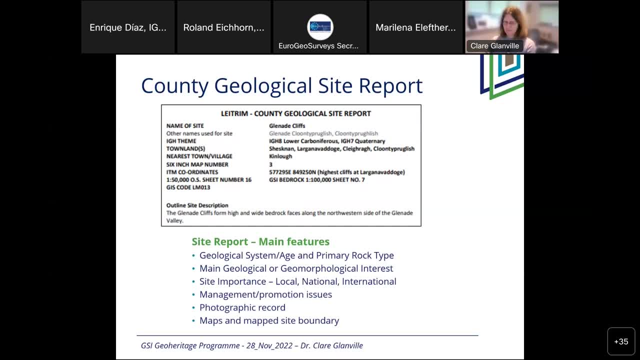 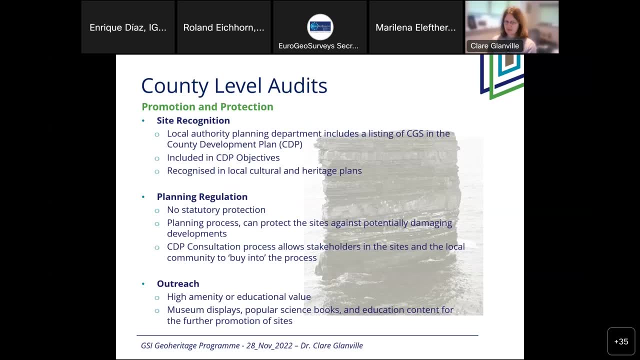 And the site boundaries are clearly mapped. So once the sites are audited, it's important, as Roland was saying, to get the information out there and make it usable and valuable. So the sites are recognized through the local authorities and their planning departments. 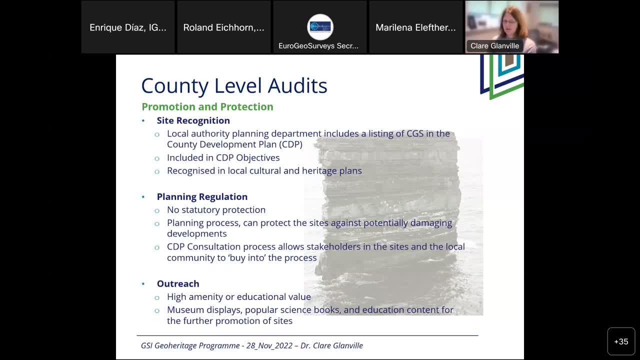 And that's why this partnership that we have working with the local authorities and the Heritage Council, is so important, because it provides an ownership of those sites within each county And The list of sites for each county is included in what we call a county development plan. 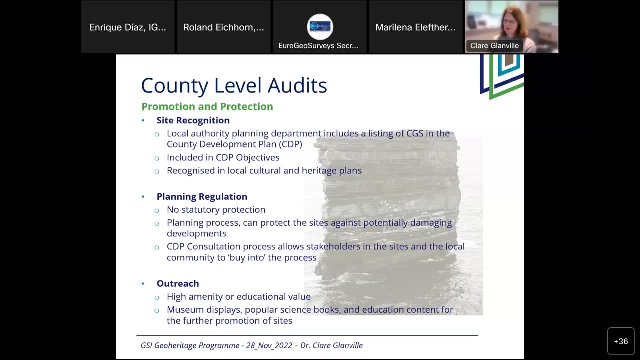 So this is a plan for the local authority as to their priorities and their objectives on a five year basis and it's renewed every four to five years. So they include a list in the counties that have been audited. They include a list of county geological sites with a map. 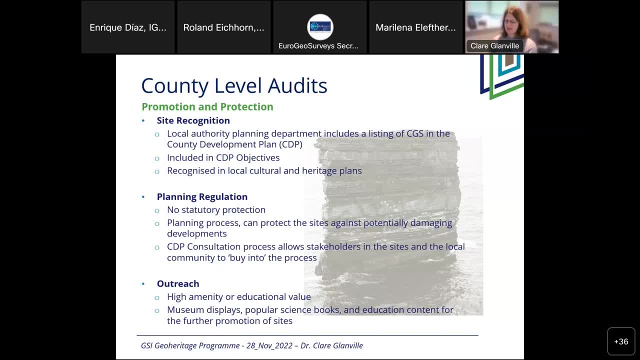 And Each site has an objective associated with it in terms of its promotion and its protection. The county geological sites are also importantly recognized in our broader national heritage plans and cultural plans And, of course, outreach is an important part of the process, as you saw from the previous. 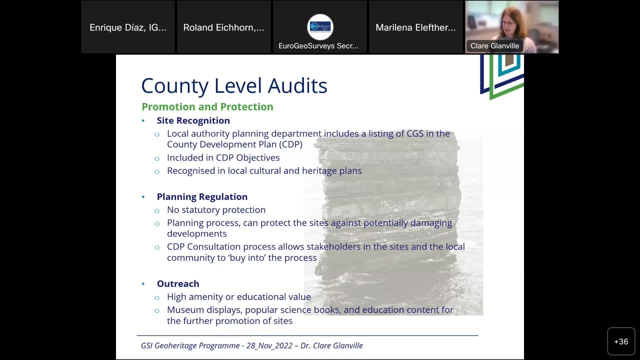 presentation by Roland And What we. as you said, many of these sites have high amenity and educational value, And so the outreach on the completion of a county geological audit includes things like museum displays which may travel between different libraries, local libraries within. 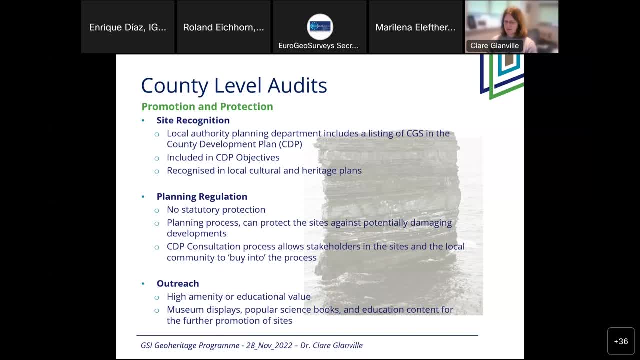 the county or larger museums, the production of popular geological or science books to make the Information in the audit more accessible to the general public, and some county councils develop educational content for their primary and secondary schools and other promotional activities such as guided walks and tours. 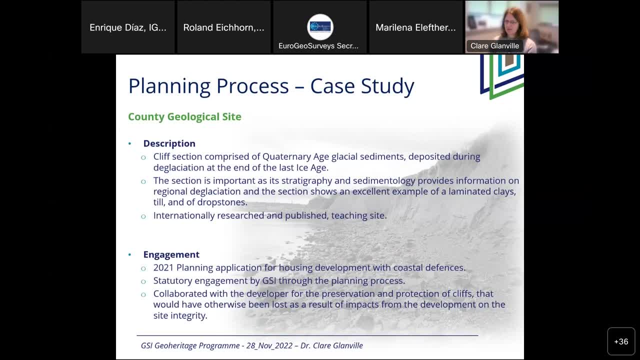 In the context of protection and promotion. I'd just like to give you an example of how this works Within the planning process In Ireland. this slide has quite a lot of detail, So what I'll do is move on to the next slide, and then I will just talk about some of this. 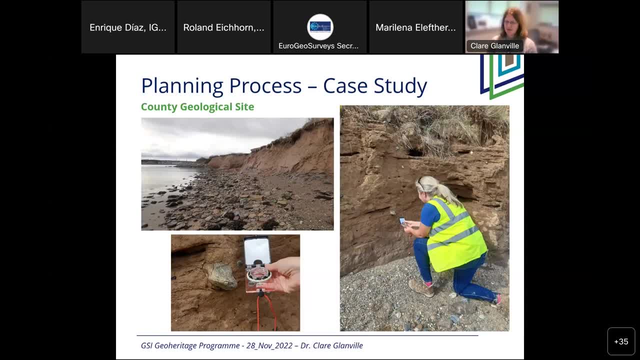 So this is a coastal site, It's a county geological site, It's a cliff section and it's composed of quaternary aged glacial sediments. In fact, There are five different fasces exposed in this cliff representing fire, Five different depositional environments at the end of the last ice age and the sedimentology. 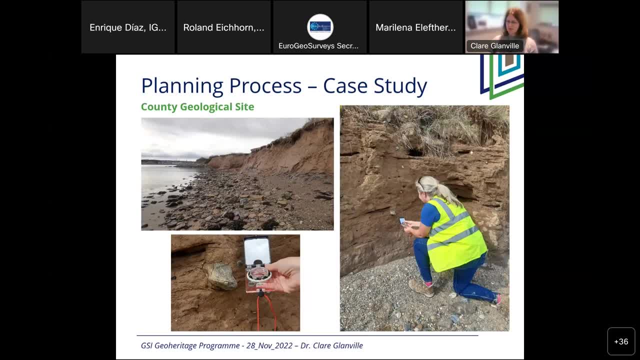 provides information On processes of regional de-glaciation. So this is an important site nationally As well as locally. this section shows excellent examples of laminated clays till deposits and drop stones. You can see some of these in the photos here. 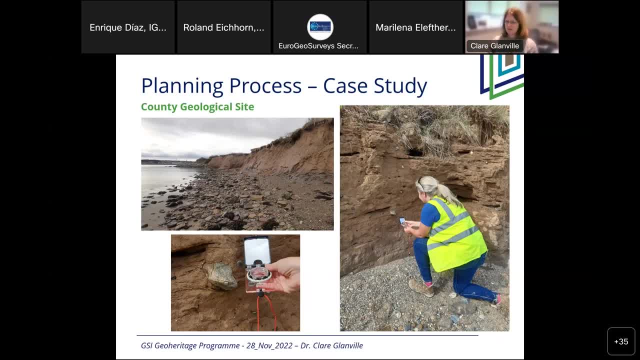 So, Because this site is a county geological site and it's listed, as I said, in the county development plans, when a housing development planning application was lodged with the local authority, the planning department were aware of this site And they made us aware of the planning application. 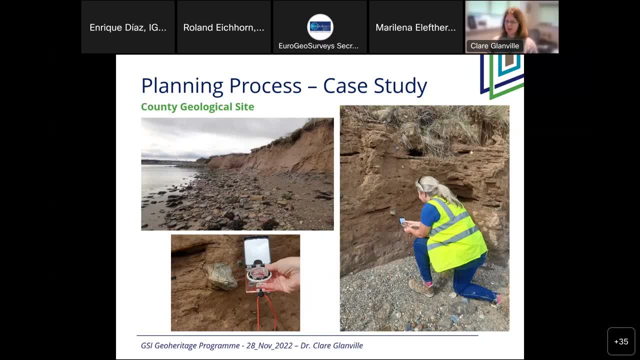 The development had proposed to Cover the cliff that you see here With rock armor to prevent further erosion From natural processes and weathering. This, unfortunately, would have completely obliterated The exposure and also access to it for future and study and research. 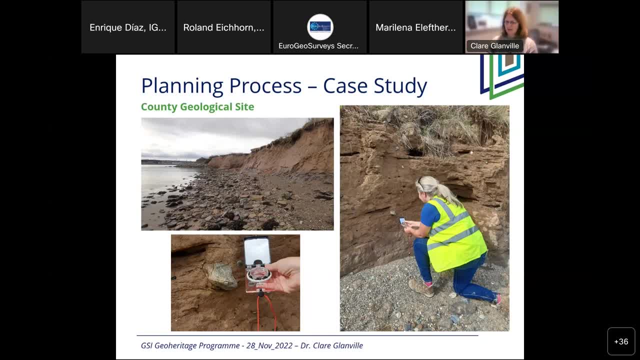 So we, Through this planning process, and because the sites have been audited and listed, We were able to engage with the developer. We went and visited the site by ourselves, first to assess its current condition, And then with the developer and their engineers too. 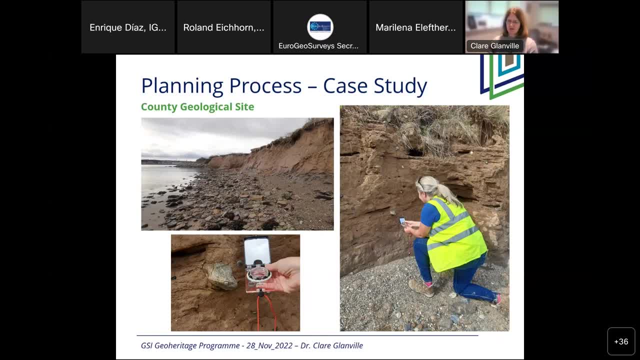 Look at the site and see what we could do in terms of Protecting the geological heritage here, And while there was a large section- probably 200.. 300 meters long- that they wanted to protect with rock armour, we were able to select a 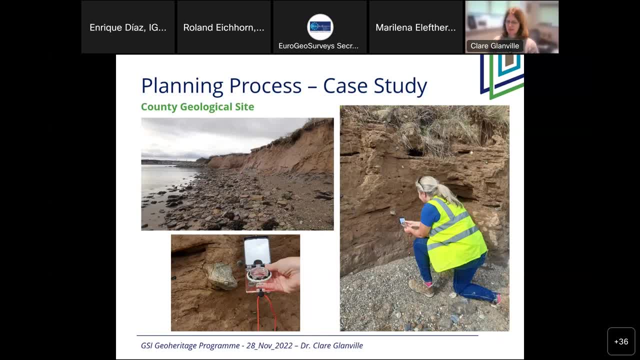 smaller section of the cliff of about 20 meters long, which showed the widest range of geological features and heritage that we wanted to preserve, And so we worked with them to examine, and their engineers, of course, to examine- different coastal protection techniques that may allow. 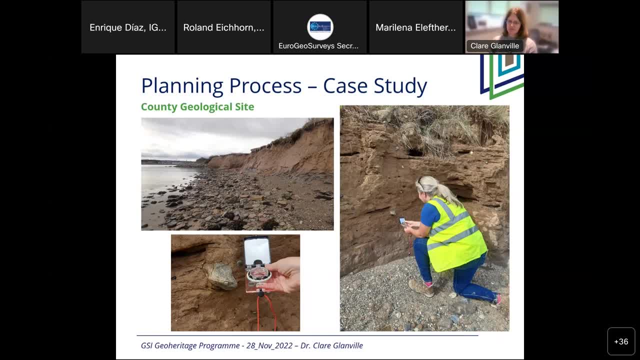 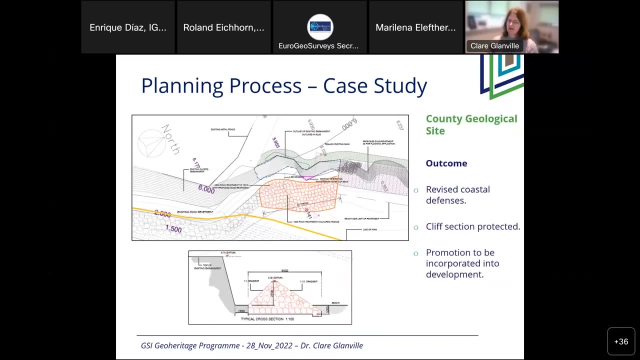 this site to remain open to the public, to have access and to preserve it, And so what we came up with, or I should say what their engineers came up with, was a proposal. As you can see here, this section is the rock armour up against the cliff face which they 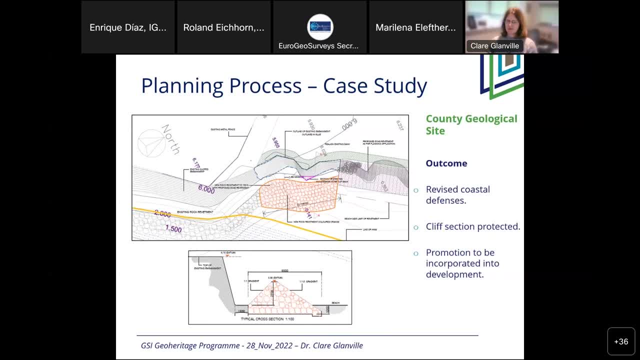 had originally proposed for the hold. This here is the section of 20 meters that we agreed that we would protect, And what they did was they proposed a stepped back rock armour. You can see it in this lower diagram- Sorry, the images are not great. This berm- a way of describing it- of rock. 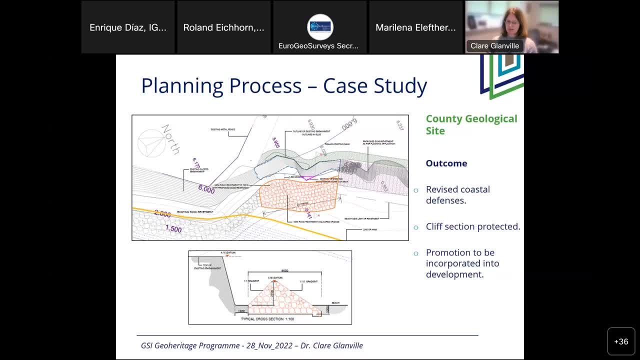 armour is stepped back by about one and a half meters from the cliff edge. It's designed to be porous so that the tide can still move through it, but the energy of the waves is taken, And so for this section the cliff exposure is protected and also the development. 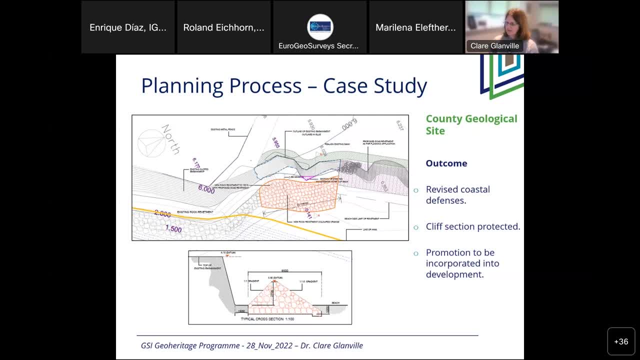 is protected. This was a little bit of a tricky site because it was… Okay, as it was a cliff site, it was already at the risk of natural erosion from natural processes, so we had to decide what was the value in protecting this site if, with given sea level rise. 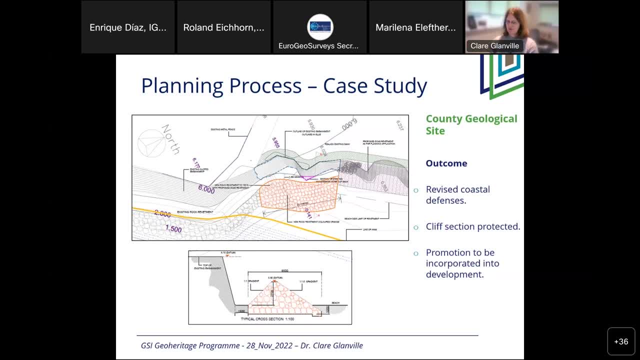 changes and estimates and stronger storms, whether this site was under threat from natural processes, whether there was value in protecting it and how much of it should be protected. so all of these things were taken into consideration, also the chance that without the natural erosion that the cliff face may slump and become obscured anyway. so these are all factors that had to be. 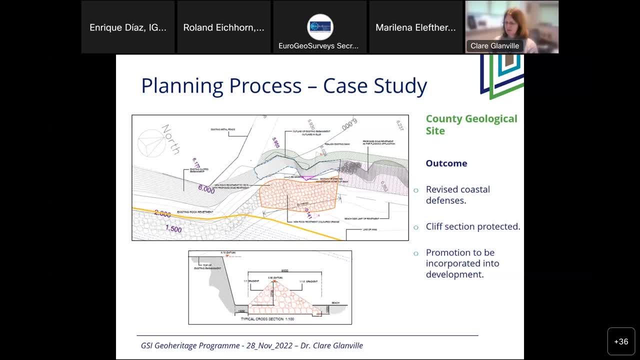 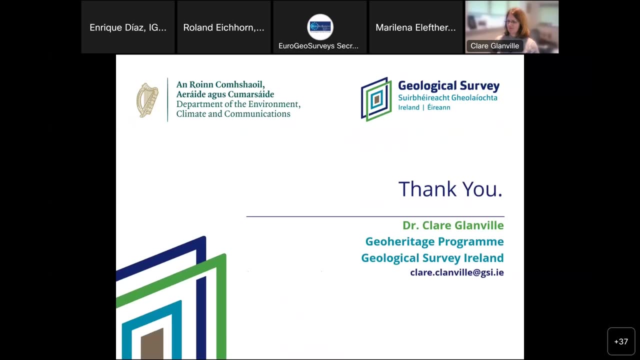 taken into account, but I think the solution that has been proposed takes as many of those boxes as possible, and I think that is about the end of my presentation, and so if you have any questions, I'm happy to chat to you about them at the end. thank you very much, okay, thank you very much, Claire. 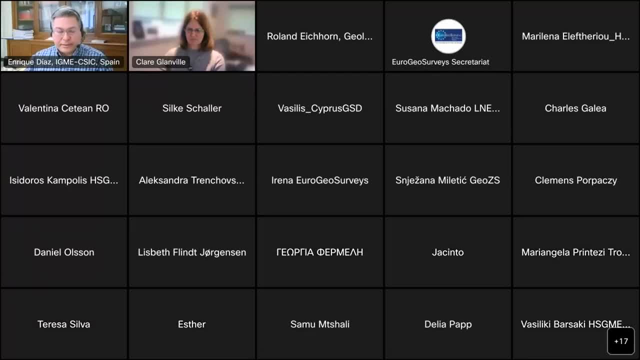 very interesting also to see the real examples, as I was mentioning, with the good things and the bad things, and we can talk about all those later, and so now we will have the video that was recorded by Nicolas. his presentation is going to be highlighting geo heritage in the world's leading tourist country that is France. by Nicolas. 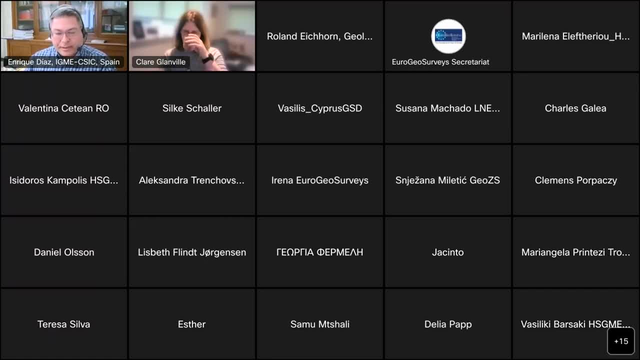 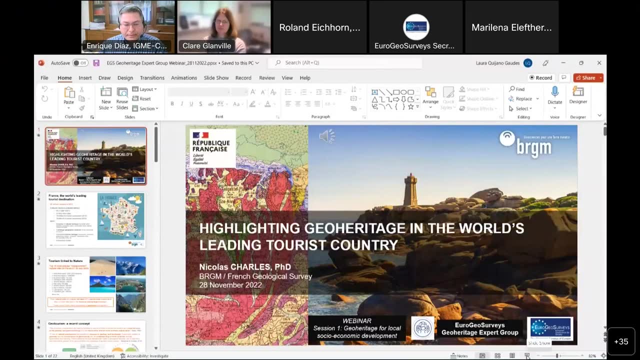 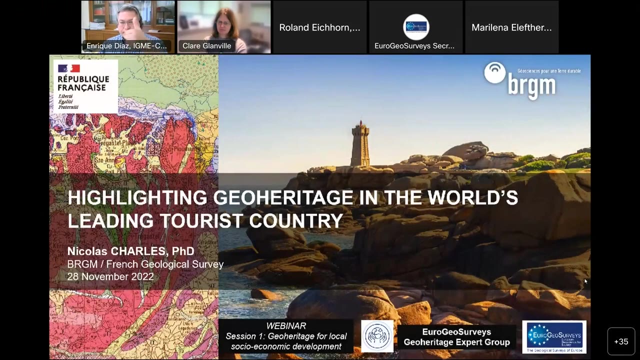 Charles, he's from the French geological survey, the PRGM. let's see if it works. if you want to begin the presentation, okay, good morning, ladies and gentlemen. I am very glad to take part to this first webinar organized by the eurogeo service charity expect group. this presentation will present the relatively unknown link between 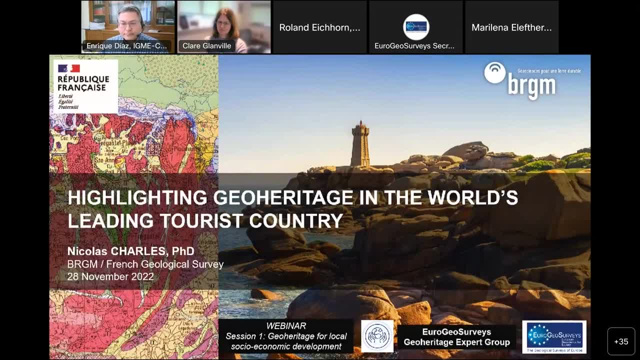 geraritage and tourism, an important economic activity in Europe in earth sciences, support of tourism which can be linked to geology school and geotourism. the goal of this presentation is to show how a digital survey can highlight geraritage and its conservation through touristic activities taking 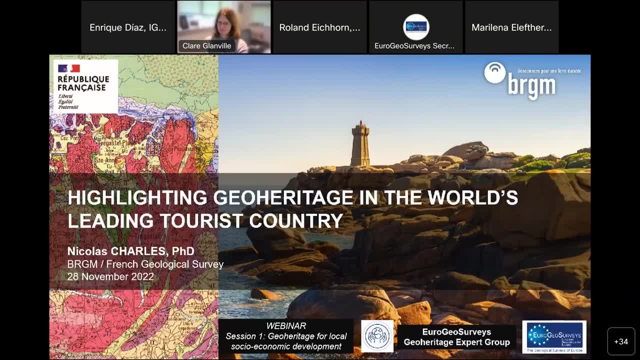 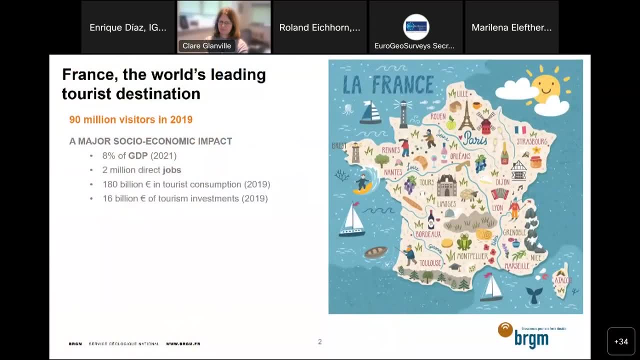 the example of France, the first touristic country in the world. as I just said, France is the first touristic destination in the world, with about 90 million tourists in 2019.. this has major economic inclusions, including food reserves. climatic tourism impact for this country, since tourism participates uh to eight percent of gdp, generates two million. 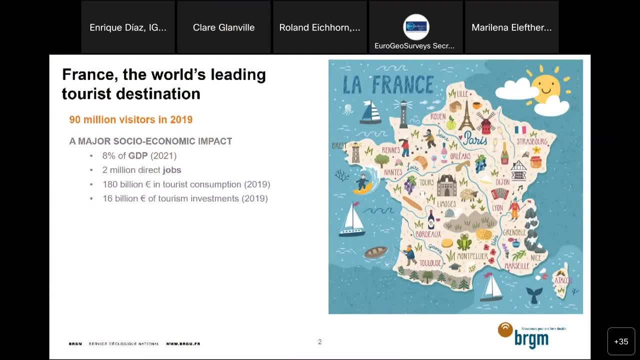 jobs and the tourist consumption represents 180 billion of euros in 2019. but why? this country is the first destination for tourists in the world. france is relatively a small country, but with a high diversity of natural heritage, with beaches, mountains, plains, lakes, icelands and the 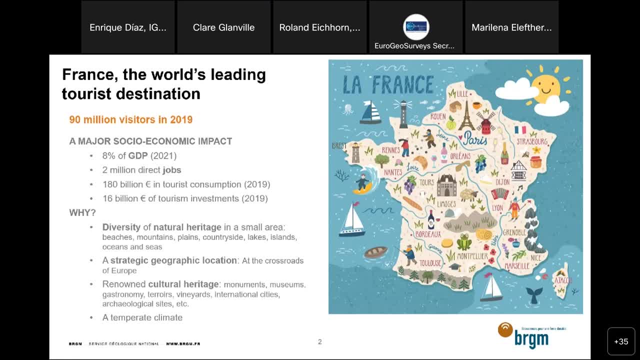 second largest maritime domain in the world, if we consider also the overseas territories. france has also strategic geographic position at the crossroads of the european continent, with international airports with big hubs, highways between north and south of europe or high-speed highways. moreover, the french category is internationally renowned, with a lot of monuments, museum, a famous gastronomy, the. 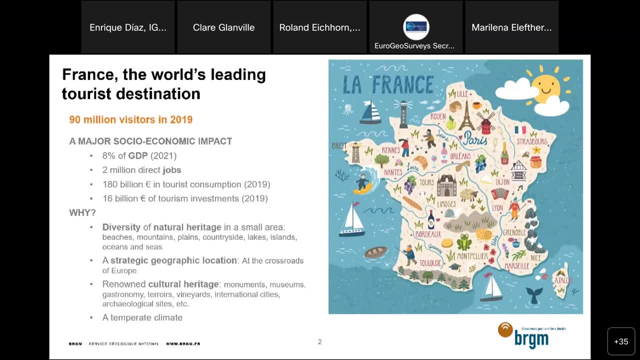 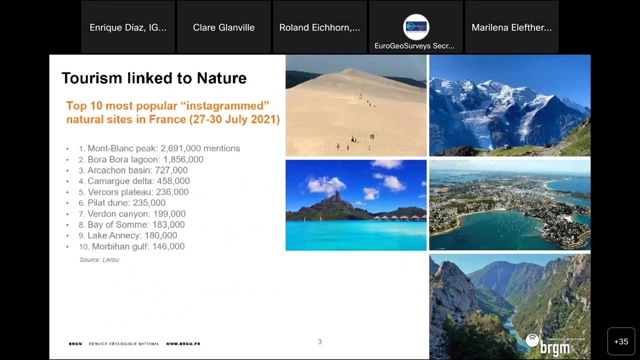 tradition of terrors and varniers, the possibility to visit international city and archaeological sites. finally, tourists also appreciate the temporary climate, especially in summer. on this slide, you can see a list compiled by a travel agency in france during a few days in summer 2021. this list represented the 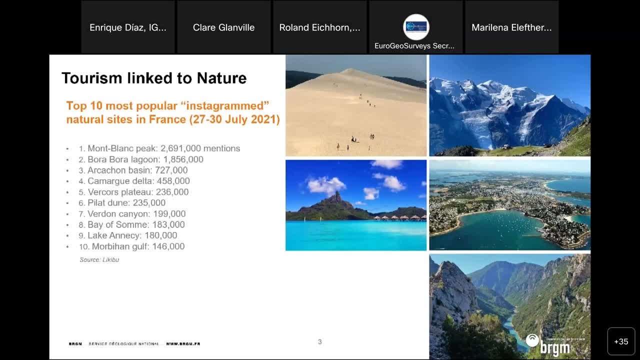 most mentioned natural sites on the application instagram, as mont blanc peak, the top of the european union, the verdant canyon or even the pillar dune, the highest dune in europe. we can note that all these touristic sites are natural heritage. with the geo heritage components, it's also noteworthy. 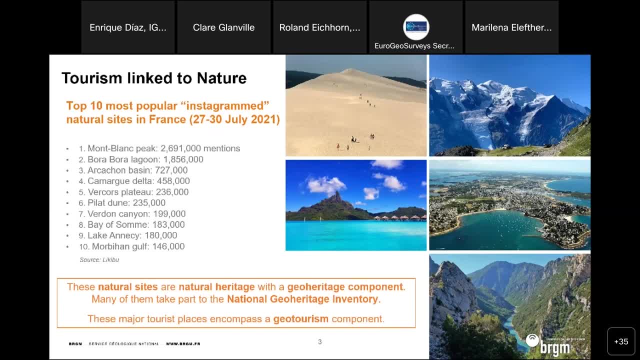 that most of these sites are taking part to the national heritage environment. as a result, most of these sites are taking part to the national heritage environment. as a result, we can note that all these touristic sites are not only a good example of a historical or archaeological site, but also important and significant for the future of portugal and all of its 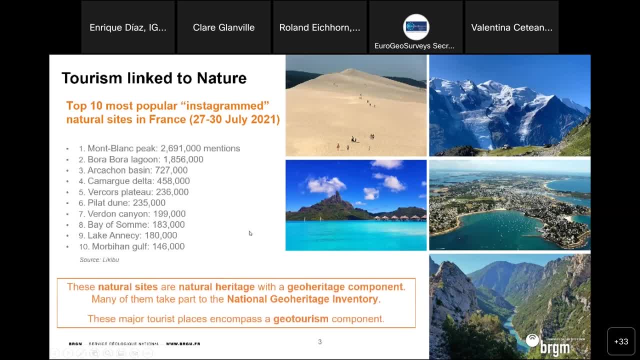 metropolitan and regionalavilies. we can note that the current rockükyn rockery project is a great opportunity to take place here coming after the summer 2020. we can note that all these touristic sites are natural heritage with the geo heritage components. it's also not worthy that most of these sites are taking part to the national 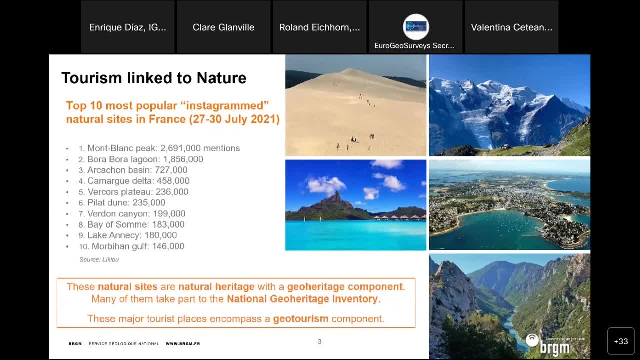 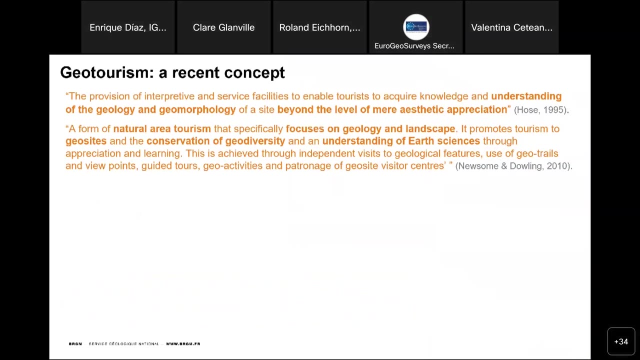 heritage inventory in france. as a research, we can say that these sites encompass a part of geotourism. but what is geotourism? geotourism is quite a recent concept, with the first published definition given by hoos in 1995 as a provision of interpretive and service facilities to enable 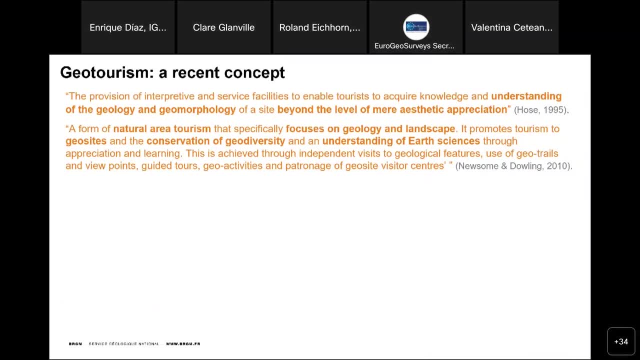 tourists to occur: knowledge and understanding of the geology and geomorphology of sites beyond the level of mere aesthetic appreciation. more recently, in 2010, newsom and doling gave a more precise definition. if i enjoy tourism as a form of natural reasons, that specifically purposes: 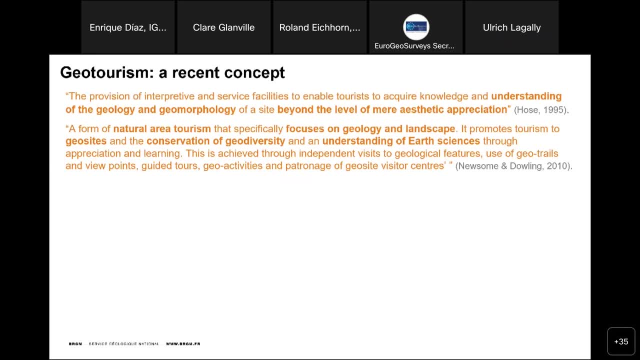 to escape. it promotes tourism in geosites and the conservation of geodiversity and understanding of pro-senses through appreciation and learning. this is achieved in independent visits to geological geo-trail and viewpoints, guided geo-activities and patronage of their site visitor centers. 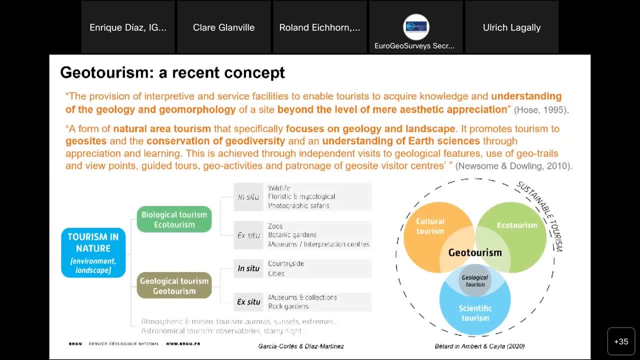 we have seen before that many natural sites are linked to geology. tourism in nature, as you can see on this figure to the left, aims to discover environments and landscape with a sustainable development approach, especially through ecotourism and the discovery of biodiversity, as, for example, in national parks and natural reserves. however, see a hipotic. 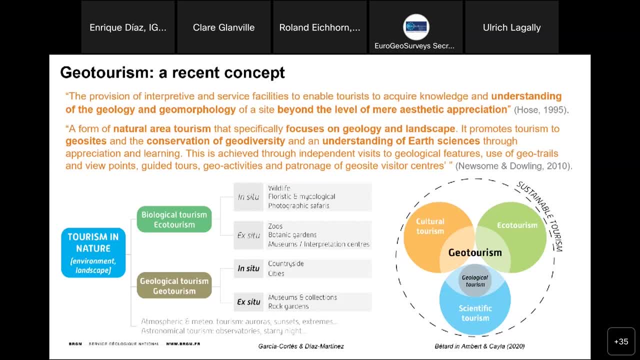 equivalent of biodiversity and biodiversity. biological heritage is often omitted. I'm referring to geodiversity and geotourism. We can visit in situ or ex situ sites. as you can see on this figure, Geotourism is also fully participating to sustainable tourism, as defined. on this figure by Beta. 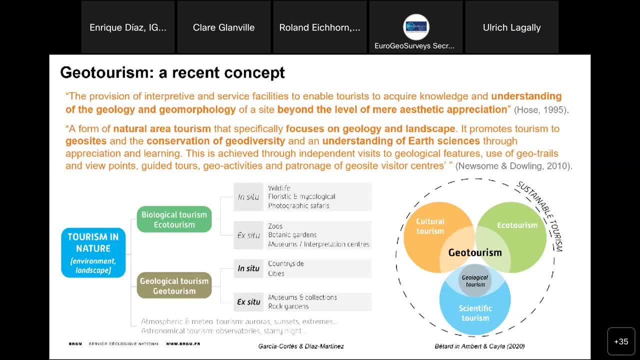 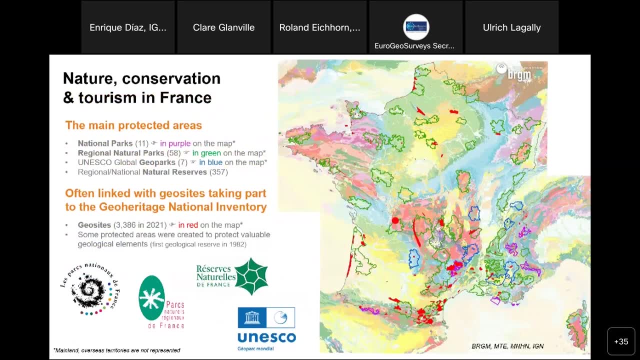 where geology can make the link between different types of tourism- cultural, ecological or scientific- Okay. well, on this map of Maine and France are represented the main natural protected areas, with national parks in purple, regional natural parks in green and UNESCO global geopark in blue. 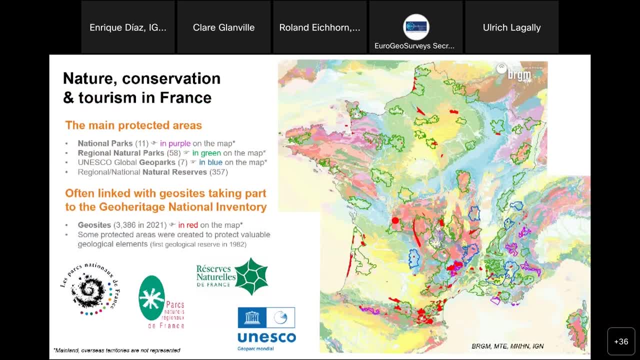 Moreover, red polygons and points on this map represent the geosites taking part to the national heritage inventory. Many geosites are included in these main protected areas and some of them are protected by the National Geological Survey. The conservation of these areas have even been created. 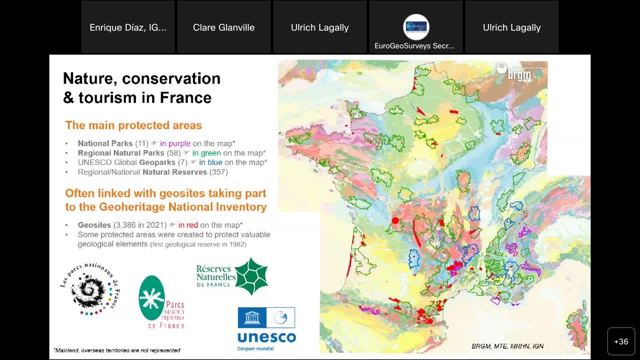 especially conserved by the geosites. As for the, that's so kind of bright, Please, everybody, mute your microphones please. However, geology is often not mentioned in these protected natural areas, even though geoharitage is an integral part. 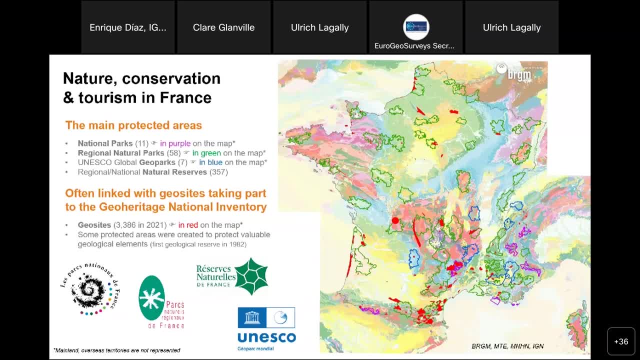 of natural heritage, and its conservation is as essential as that of biological heritage, So it's very important that we do this. Okay, However, geology has to explain and understand the Earth's history, the history of landscape and their evolution, and also the evolution of the environment of a special territory. 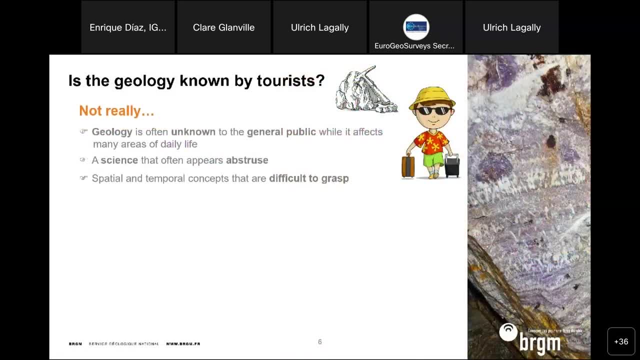 or a region To the question is the geology known by tourists? the answer is not really, because geology is often unknown to the general public, while it affects many areas of daily life. It is a science that often appears abstruse, and spatial and temporal concepts appear as 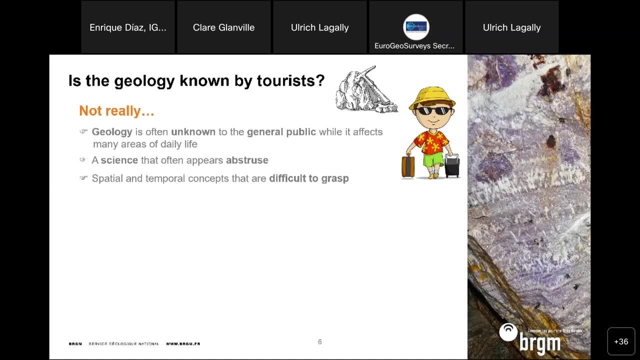 difficult to grasp, especially in terms of million years or billion years. But, at the same time, people never stop trying to understand the geographical, natural, cultural or socio-economic environment in which they live. These desires tend to respond to simple curiosity or fears, often linked, for example, to natural. 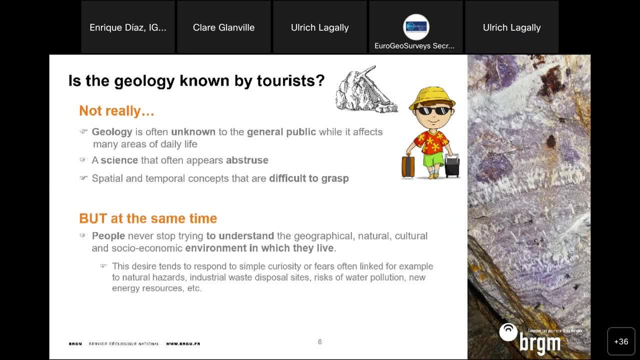 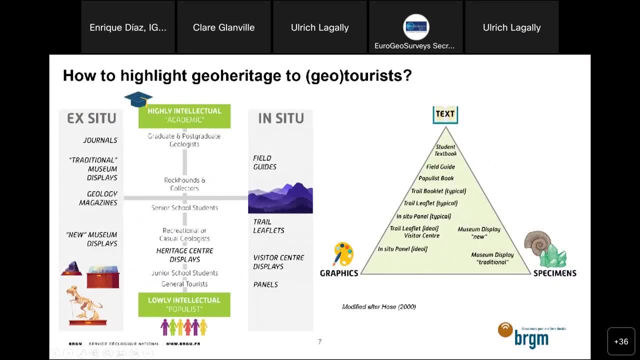 hazards: industrial disposal sites, risk of water pollution or new energy resources, etc. Well now, how to align geology to tourists and finally to geotourists. The first point is to identify the audience, as you can see on the figure to the left. 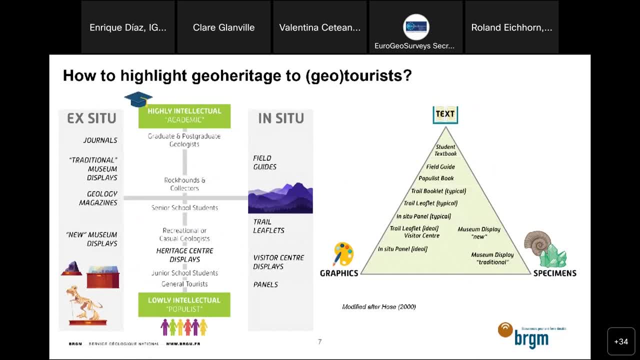 between the low-scale and the high-scale audience in order to adapt the type of communication, support with panels, leaflets, guides, museum displays, general public books, etc. You have also, as you can see on the figure, to the right to choose, the good expectations. 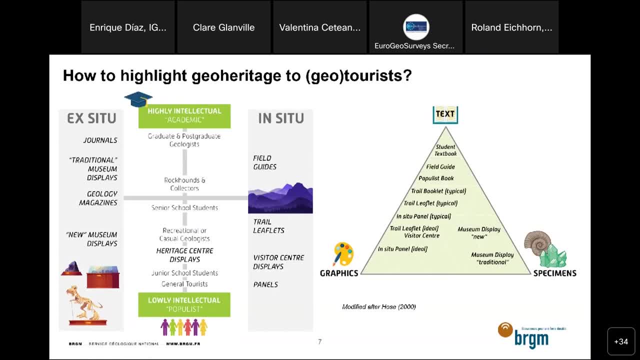 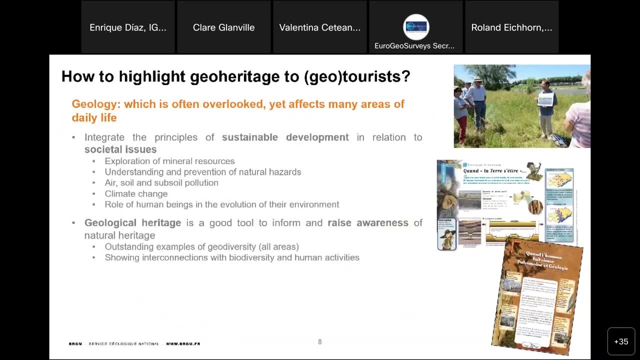 and the bad expectations. This is the equilibrium between texts, illustrations and specimens of rocks, minerals or fossils, As geology is often overlooked, while it affects many areas of daily life. as I already said, the best way to align this science is to integrate the principles of sustainable development. 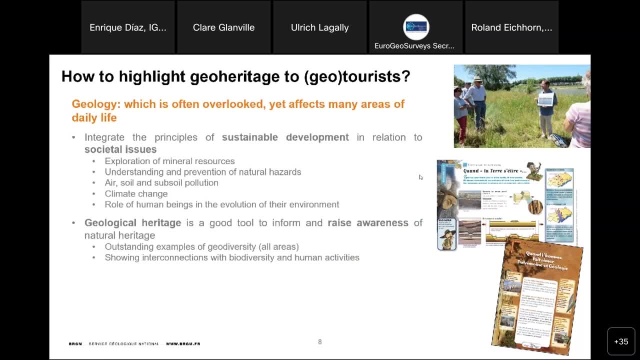 in relation to the socio-economic environment, like mineral resources, use, understanding and prevention of natural hazards Here soil and subsoil pollution, climate change and the role of human beings in the evolution of their environment. Geological heritage appears as a very good tool to inform and raise awareness of natural. 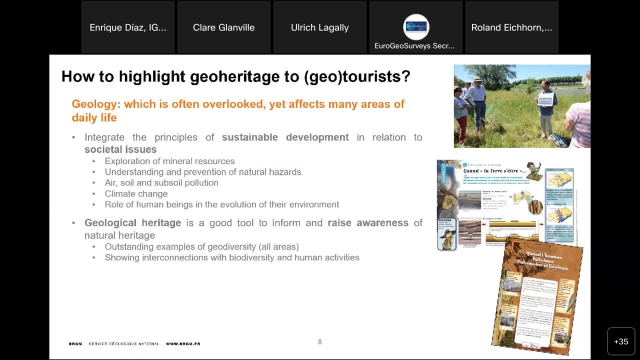 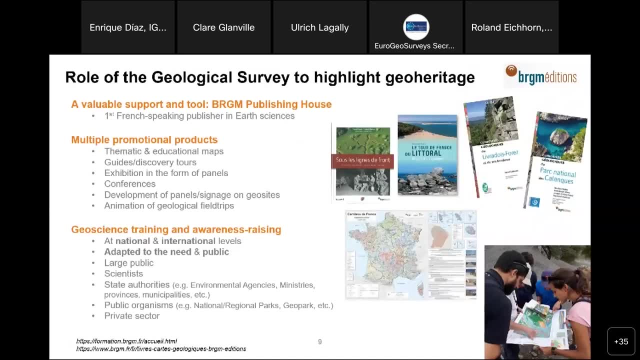 heritage, especially with outstanding examples like amazing landscapes, and that show interconnection also with biodiversity and human activities. But what can be the role of a geological survey? Well, first of all, it's important to understand the role of the geological survey. 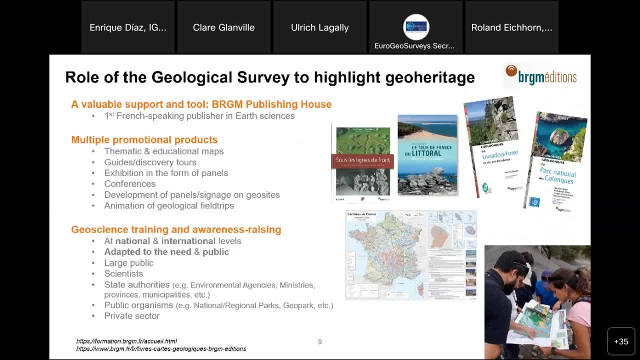 Let me present you the example of BRGM, the French Geological Survey. One of the best valuable support and tools for a geological survey is to have a publishing house or a similar department For BRGM Publishing House. it represented the first French-speaking publisher in earth. 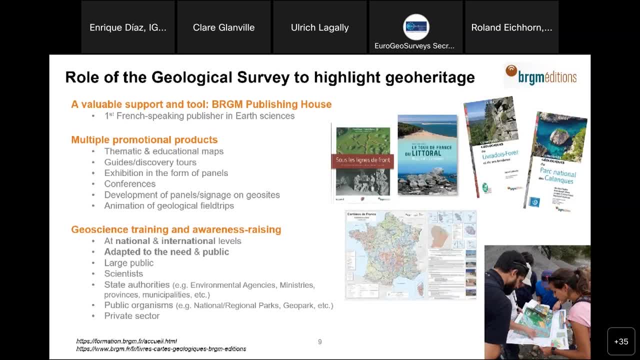 sciences. This department can provide multiple promotional products like maps, guides, panels for exhibition or site development. Conferences are field-tripped. Another main role of a geological survey is geoscientific training and awareness raising. It could be carried out at national or international levels and adapted to the needs of the audience. 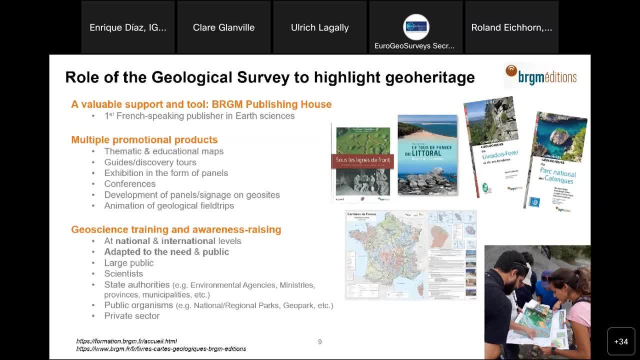 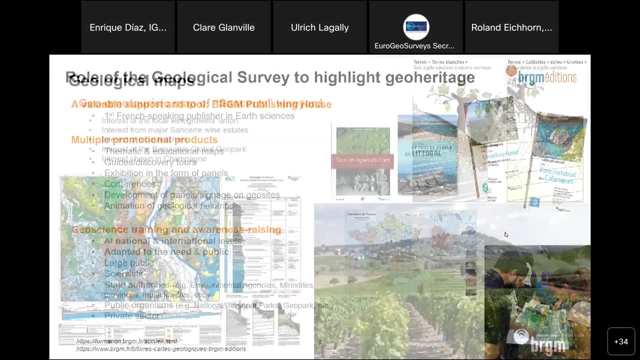 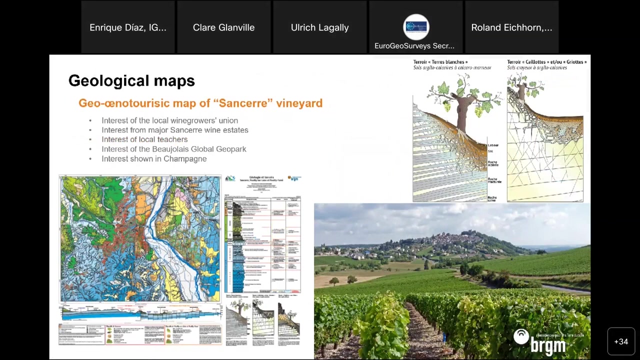 A survey can work with state authorities, especially those managing the natural protected areas, but also with public organism like university, but also with geoparks and national and regional parks, And even also with private sector. The first example here is this thematic map with a new geotouristic approach for the Saint-Servagnes. 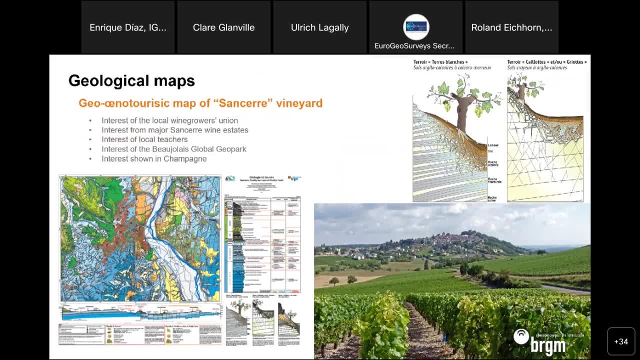 Yard, located in the center of France, close to the Loire Valley. We mentioned the link in this document between geology and terroir, with didactic figures showing the different profiles of soil, as you can see at the top to the right. 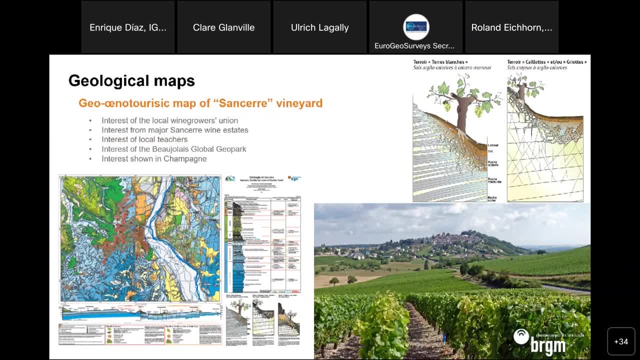 The location of vineyard plots. The location of the vineyard plots And the history of vineyard are also mentioned on the map. We get a great interest from wine growers union or from main wine estates of this area. It's quite an uncommon way to present a scientific document at the beginning, which is the geological 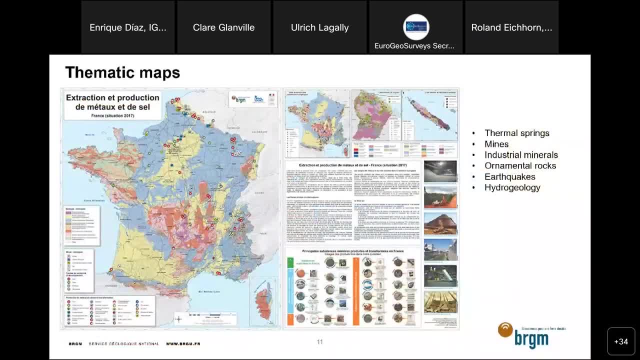 map Here now you can see another example of thematic map showing the sites where extracted some mineral resources and their daily life uses and application, as I exemplified at the bottom of the slide. Right of these figures, photographs, symbol and texts are balanced according to the targeted 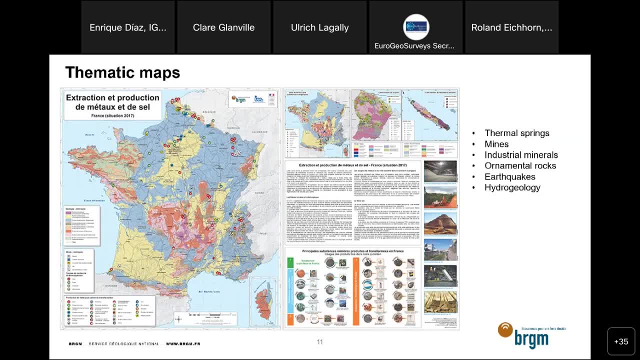 public Here more raw material industries and university. You can also have thematic map dealing with thermal springs, mines and also industrial minerals Or ornamental rocks and the link with built heritage. You can also have a map with historical earthquakes or even hydrogeological map showing the water. 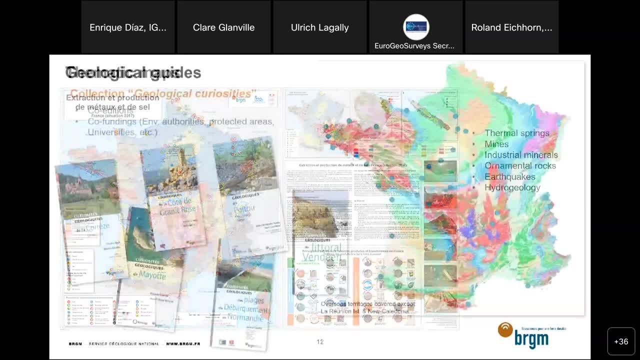 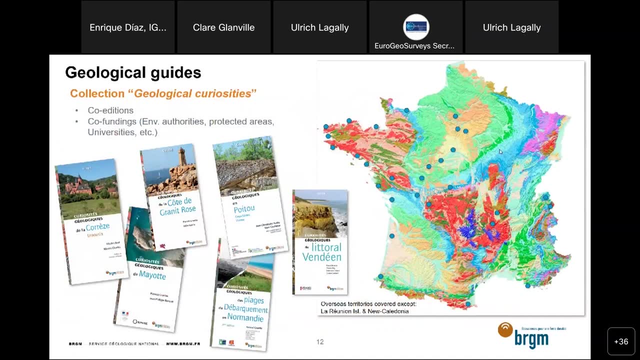 ground resources. Thank you, Thank you very much. you have some example here of titles in touristic areas of france. an important point also to mention is the co-editions with local actors and to find also co-founding to show the interaction with the different stakeholders involved in the territory for this collection of field. 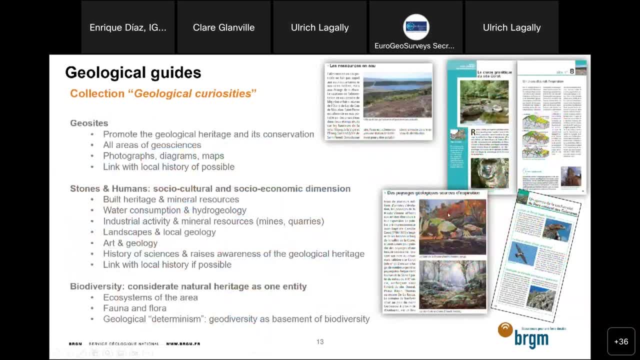 wise and title geological. you have different parts. the main one present different geosites promoting your heritage and conservation for a territory. this geosites covers whole geosciences, not only pure geology. you can have a geological geology, geosarts or even mineral resources. 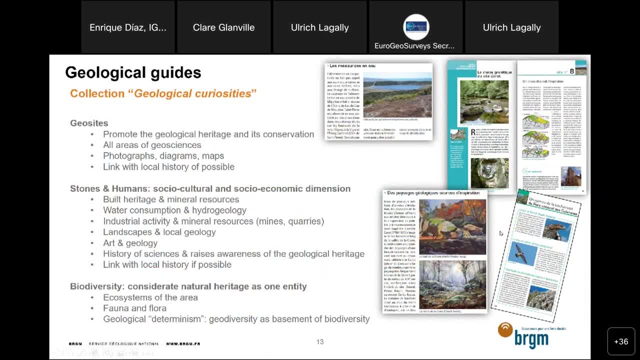 and this guide are profusely illustrated and balanced between photographs, diagram, maps etc. and texts. a link between geosites and local histories are so fostered. another main chapter for this book shows the links between stones and humans through social, economic and social cultural dimensions. that means, for example, built heritage and mineral resources. what kind of rocks? 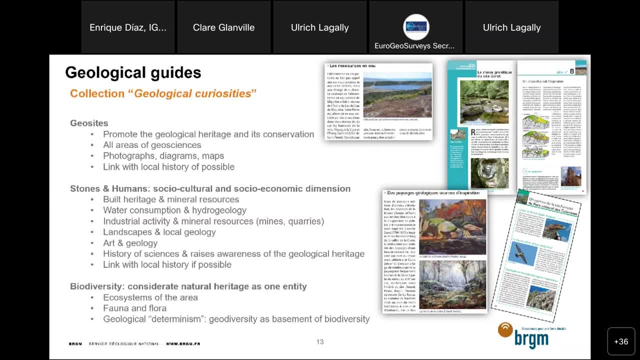 used in the monuments, water consumption and water, grown resources, industrial activities or heritage with active or former mines and quarries, or even art and geology, especially with landscape, to clearly describe natural heritage and highlight geo heritage. this kind of book also speak about biodiversity and we can just consider natural heritage and one. 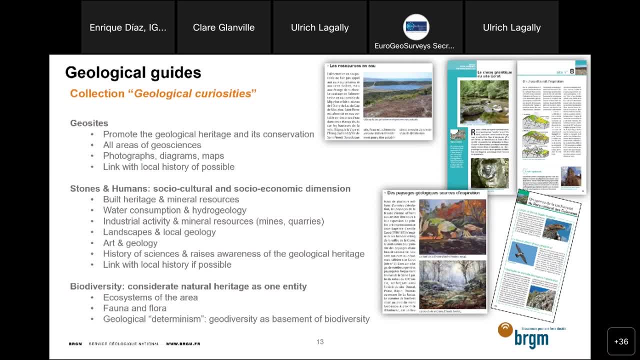 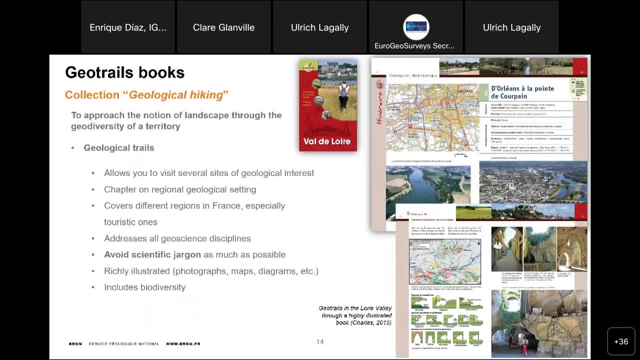 entity showing ecosystem fauna and flora and the strong links between geodiversity and biodiversity. another type of book can be the geotrails guise in order to approach the notion of landscape through the heritage of her territory. on another area, you can see the example here for the loire valley, a unesco world heritage sites in this region. 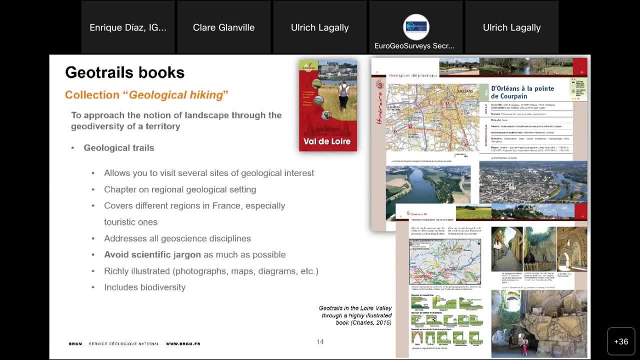 geology is not directly visible due to the lowland morphology of this area and linked to geology, must be addressed through other aspects, in this case, again with the stone used in the monuments, especially in the renaissance castle along the loire valley, for example. the stone is a 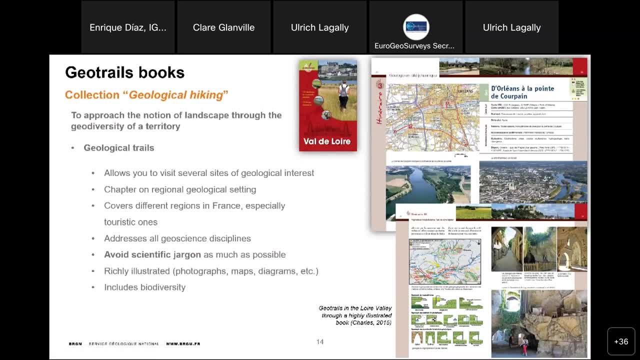 cretaceous siliceous limestone called tufo, and you can make the link with the history of people who extracted this stone in underground quarries which are now sellers on mushroom farm. you should avoid scientific jargon. is such a book as much as possible, not only talk about. 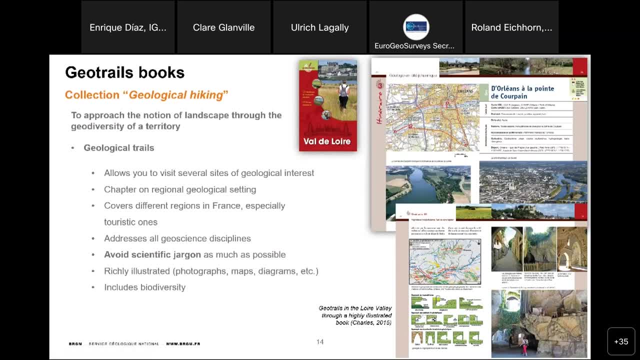 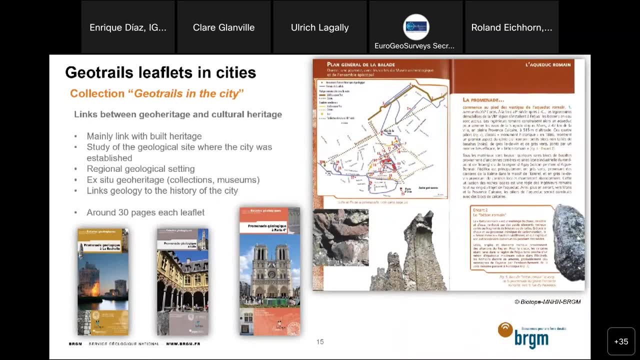 geology, but also include sites of cultural and biological interests. for example, geo trail can also take place in cities and not only in the countryside. here you have a collection of guides proposing tours in city, making the link between cultural heritage- mainly built heritage- and your heritage. you can present why the site was historically established in this place. 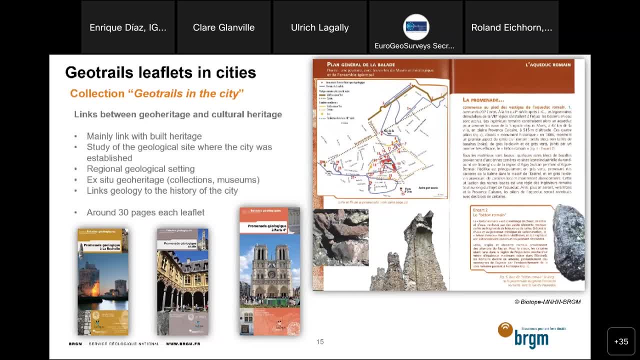 and not in another one. cities are often established for natural reasons, such as the presence of waters, the high topographical points that can be easily defended and the presence of mineral resources to build the city, and most of these reasons are linked to geosciences. you can also 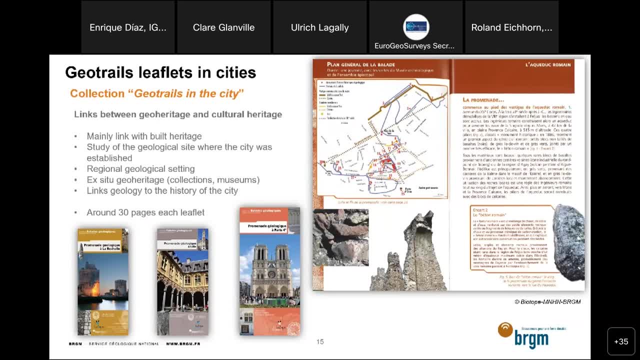 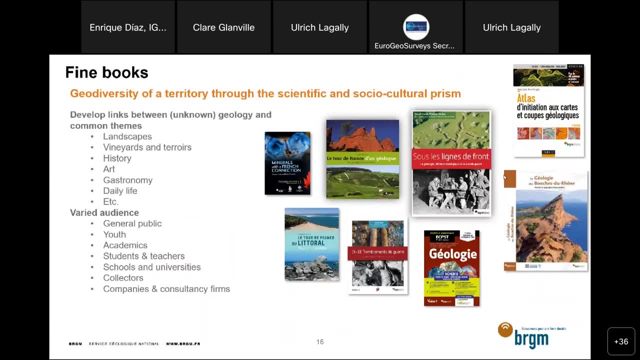 valorize the exitude jewelry page with the visit of museum collection with mineral fossils and work on the site. you can also find more information about the site in the description of this video. thank you, um. you can see the link in the description of this video you. 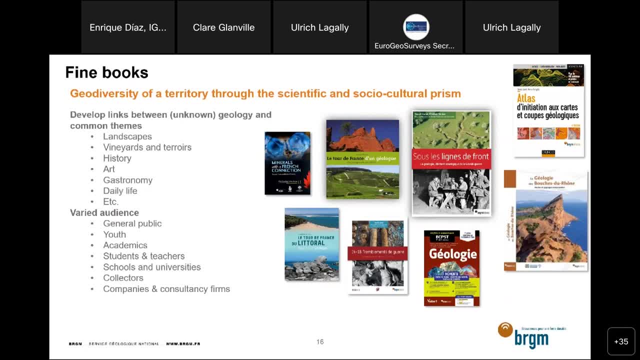 can see the link in the description of this video. you i have sent a message to the secretariat of egs to see if they can see what has happened because, please, everybody closed your microphones. she was telling me that some people are opening them. hopefully we will. 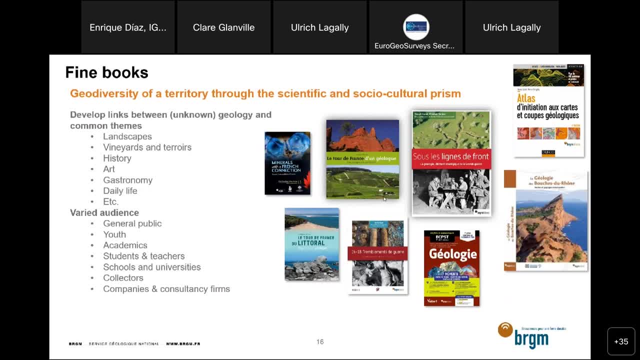 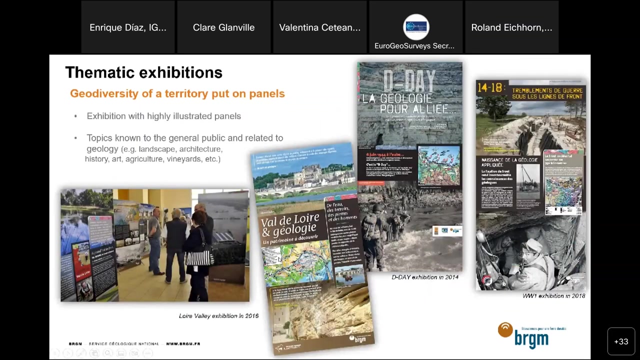 continue hearing the presentation, But we are not yet hearing. Well, I don't know if we can continue with the video, Hopefully, because it is very difficult to stop and start again. diversity- Okay, No, it continues from a touch through exhibition Illustrated panels that you can see on this slide. 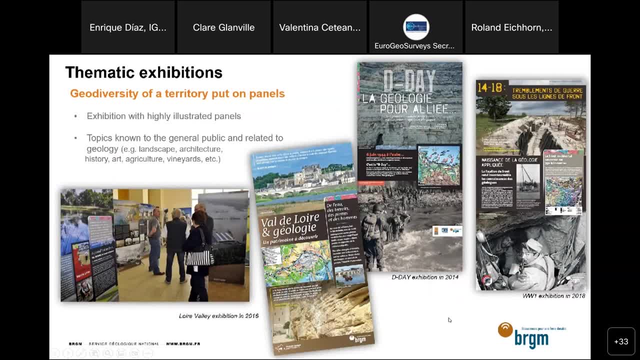 To diversity of her territory can be promoted through exhibition with highly illustrated panels that you can see. on this slide You can see some example of panel dealing with geology or the link between geology of beaches in Normandy or during the 1st world war. 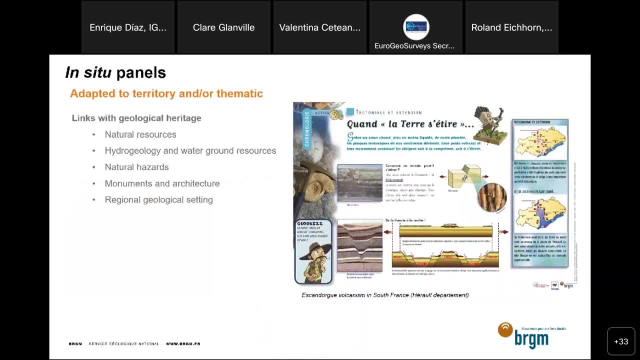 From panel illustrating an exhibition. panels can also be used in situ. Panels are adapted to a territory and or the thematic and a lot to show the link between your heritage and natural resources. Or I do a lot of geology and what a ground resources and natural has that. 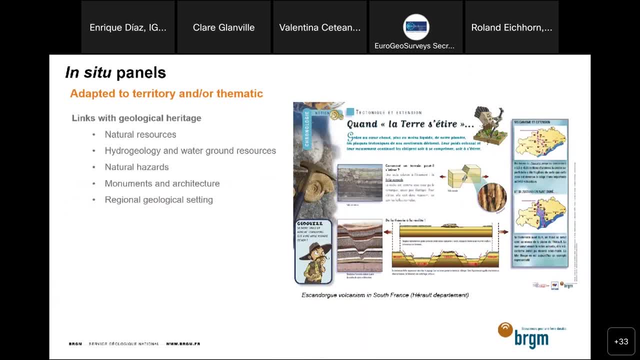 So monuments and architecture, or to expand the history through general geological setting. Here you can see an example to explain. Uh, in South of France, close to the city of This panel shows how the first is stretched and how was generated volcanism, which is still visible today Thanks to Joe, sites where we can observe flows, or basaltic prisons, or 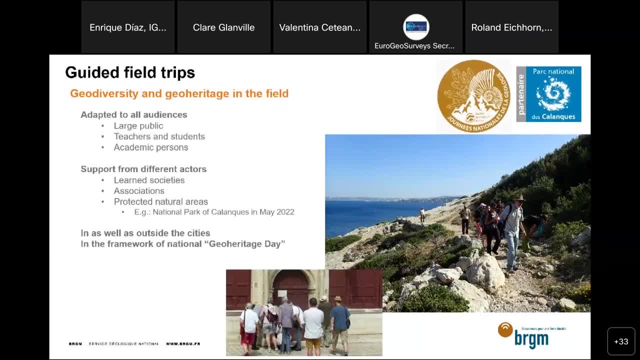 Okay. Geology is a natural science based on observation in the field. Bring public in the field during guided trips is a good way to promote your heritage. guided field trips is adapted to all audiences and can be co organized with different actors of a territory, as well: societies, association or protected areas. 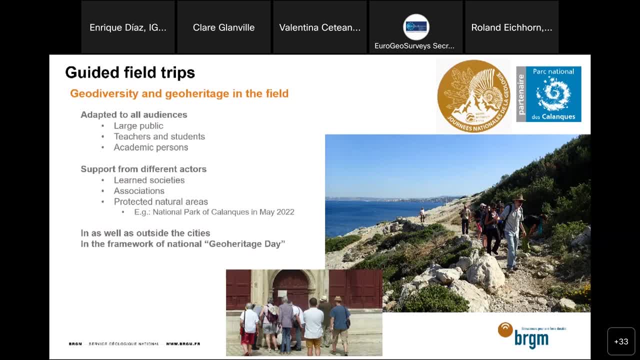 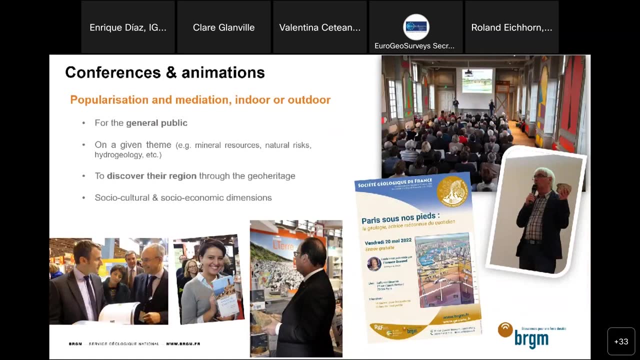 As, for example, the national park of- here in photograph, close to the city of Same, And also why the trips can be carried out in as well as Outside the cities. finally, talking about our science in front of an audience is very, very good, interactive, important, awareness rising moment. conferences or animations are always appreciated by your varied public and can cover different teams for a given territory. 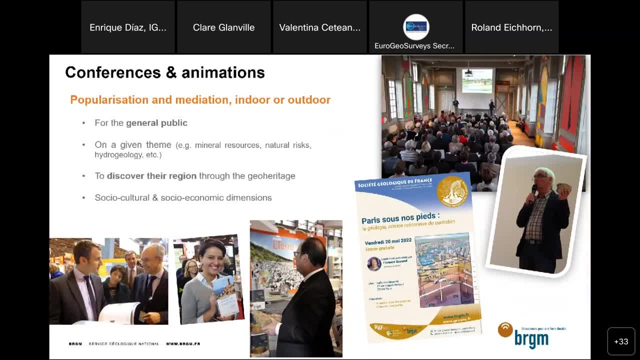 Or, more widely, Allowing people to discover their regions, to zero heritage and then go off discovery- often neglected social, cultural and social economic approaches and their links with geology should be given a priority. For the anecdote you can see on the photograph down center president around during. I remember it was during a book uh exhibition in Paris and we explained to president alone that on the on his electoral lands in central France. 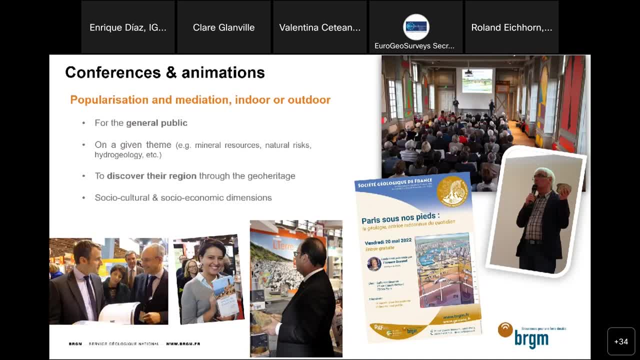 So you can see on the photograph down center On his electoral lands in central France. Um, and then we explain him When he's trying to find a way to have an A A Exhibition In Paris. And we explain to president along. 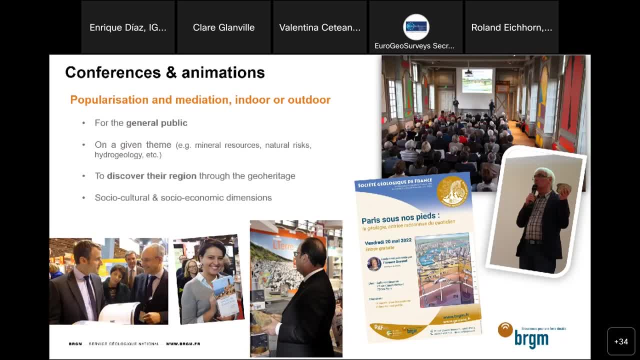 That on the on his electoral lands in central France that he has now Uh I, uh, uh uh. several geosites made it possible to observe the witnesses of an whole meteorite impact some 200 million years ago and you can see he is looking a specific rock and impact types of stage. 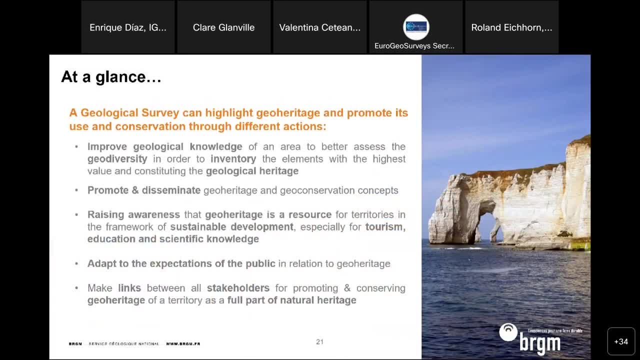 okay, so here are some main points to summarize what can be the role of a geological survey: uh, for highlighting the heritage and promoting its use and conservation. geological survey has to improve geological knowledge, to better assess the geodiversity, in order to inventory the elements with the 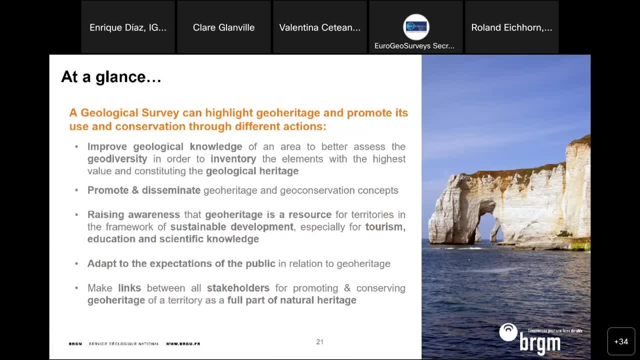 highest value constituting the geo heritage. promotion and dissemination of geo heritage and geoconservation concepts are also essential. indeed, geo heritage is a resource for territories in the framework of sustainable development, especially for tourism, education and scientific knowledge. as scientists, we need to adapt to our audience and not the other way around. 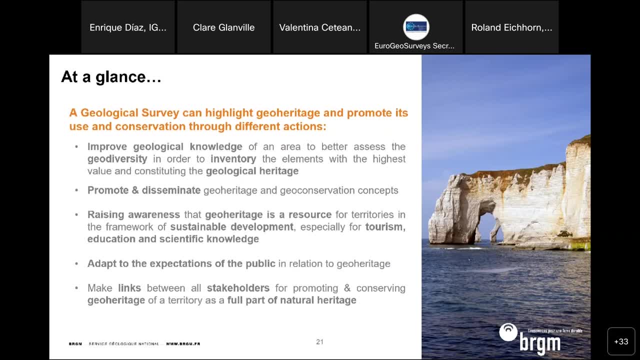 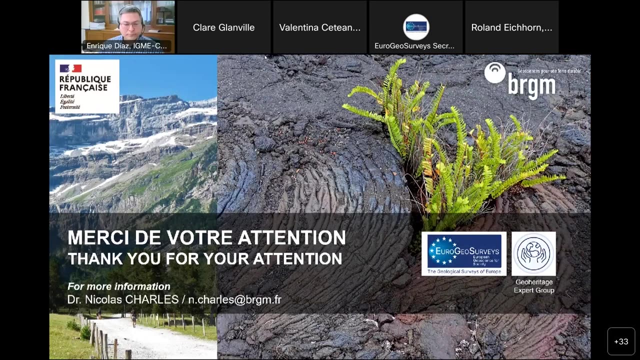 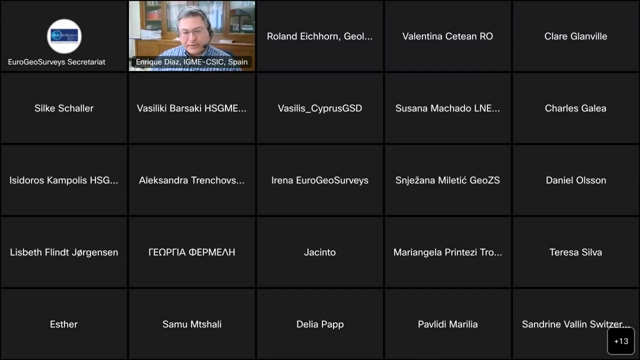 the final point is to make links between all stakeholders for promoting and conserving geo heritage of our territory as a full part of natural heritage. thanks for your attention, thank you. well, he's not present, nicolas, but thank you very much. I will let him know and 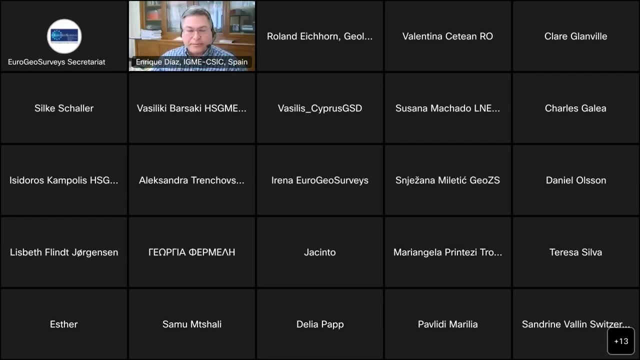 also, if you have questions, we can always transmit to him and he can respond in written. but maybe we can also answer if it is something general, not specifically about france or his presentation. so now, after the three talks, the three presentations that we have had, We will open for questions. I was already reading- There was some question post to specifically to me in in Spanish- from a colleague who works in the in the national park. 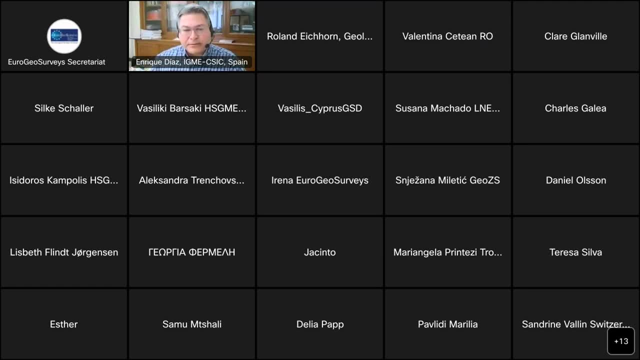 Uh, and this was uh. he was asking uh to Roland if, if you can open, let's see, Yeah, I'm hearing, Okay, And Claire, if you can also open your your video on the audio. So the the question for for Roland. he was mentioning, uh, is this discussion that you have? 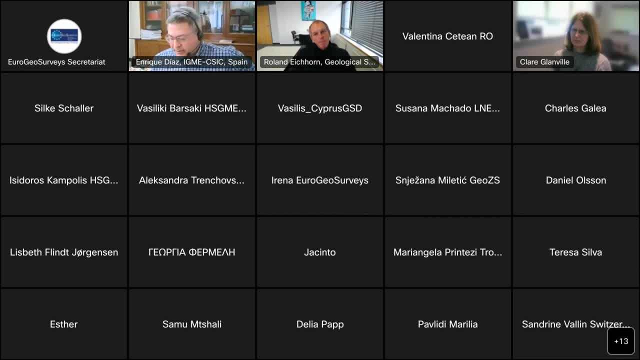 And also, I think Claire at some moment, and even Nicolas has been speaking about the, this challenge that we have between making things simple for the public outreach, But then this Generates in a in accuracy, and you were saying that. 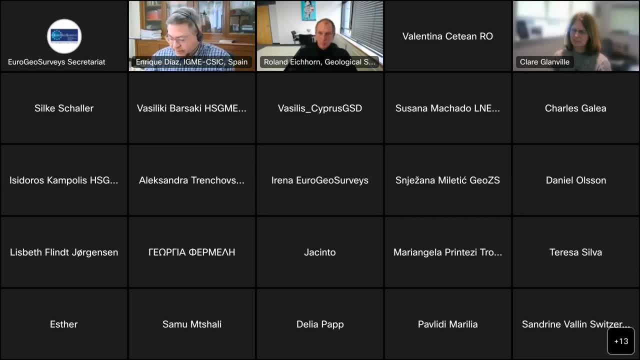 That this is sometimes, uh, it generates this, uh, That you were not very happy at some moments, maybe because you were feeling that you are, you were not doing the appropriate thing, Uh, but because when scientists see these things, then they are not happy of what you are saying. So I would like- I mean what he, he would like to mention at the same time, the this: 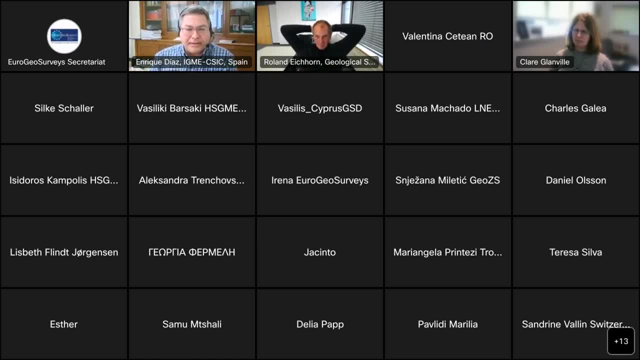 Uh branch of public outreach, which is the. it's called the heritage interpretation. You know the this from the suggest a uh that has generated a lot of uh. You know schools for interpreting uh. nature and culture for the public in general, and uh about always talking about simplicity. Are we talking about uh? 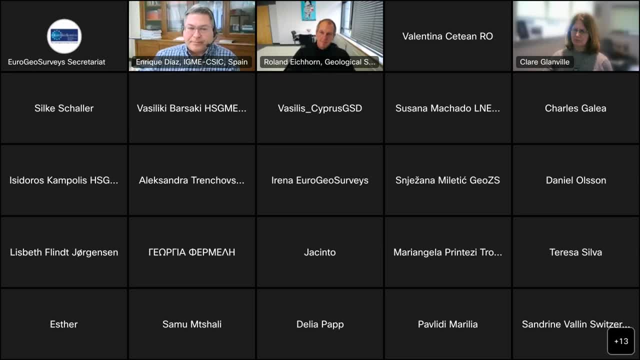 Capturing the attention of the general public in general, which is the important thing. No, so I would. Maybe Roland, because the question was posed to Roland, but maybe if you also want to say something later. uh, Claire, think about it. So, 1st, Roland, please. 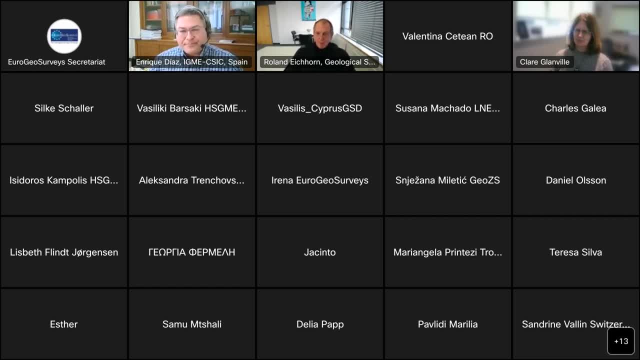 What do you think about it? Yes, it's a permanent struggle. We will love Our work and we always invent very complicated names And we think if we explain another geologist All about the geology, he will understand me. 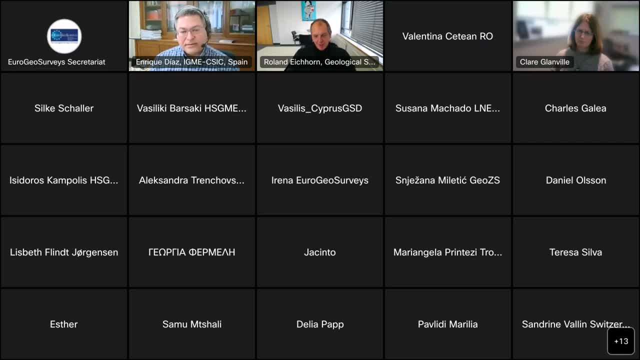 And the problem is if the other 1 is not a geologist Trouble and therefore it is absolutely necessary that you have A professional who is Able to translate the scientific language in a popular science language. And we have been both in and maybe you remember, um, I presented the talk about the, which is a very famous bird. Essentially It's an old chicken. 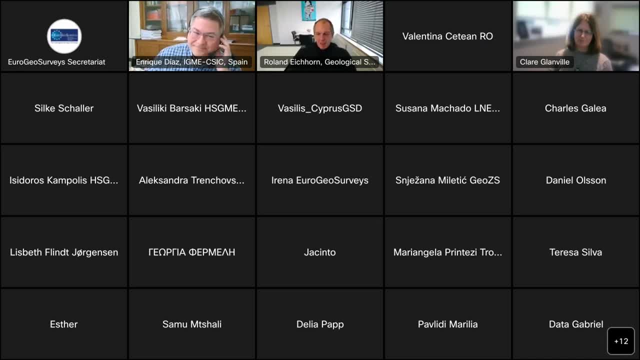 But if I say to a paleontologist that this is an old chicken, he is, he's not amused. So yeah, this is a struggle We have to, We have to deal with on a daily basis. I would say: 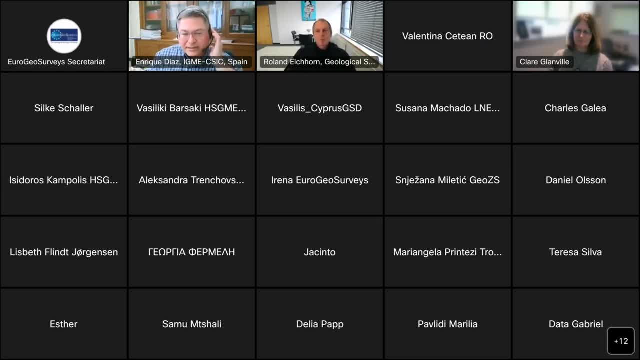 But I suppose that the- Um, I mean this- has been for generations the ability to be able to explain things to people who have Absolutely no knowledge, and the 1st thing is to grasp their attention. So usually you make certain you know, uh. 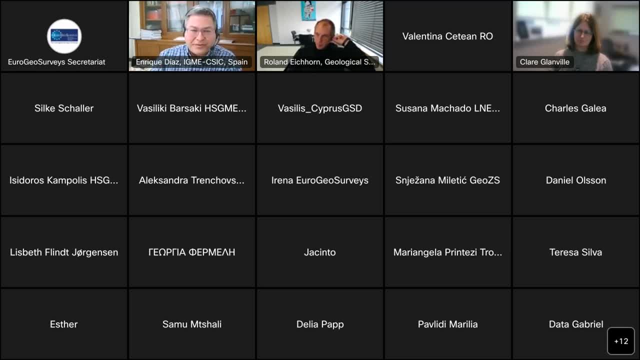 Uh, abuse of the, of the way of explaining things to Just making it so simple, so simple that it may seem stupid or just funny, but at least you have captured them and now they are willing to listen. and when, Uh, and you're right, as a scientist, you have to train that, that you explain it, let's say, far too simple in your opinion. 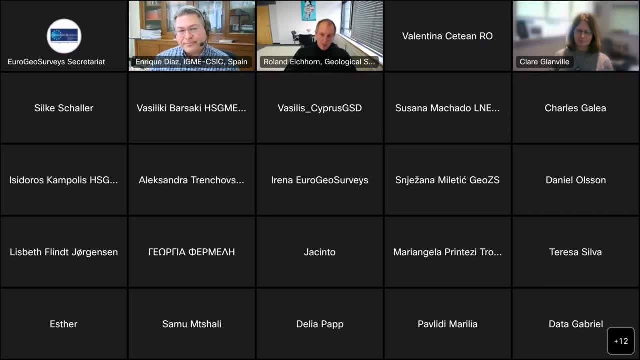 But it is not too simple and in Germany at least we don't have. if you study geology, you don't have a special uh course about uh Talking. simply explain it simply. you are not used to that, but if you work in geotourism you have to learn that. 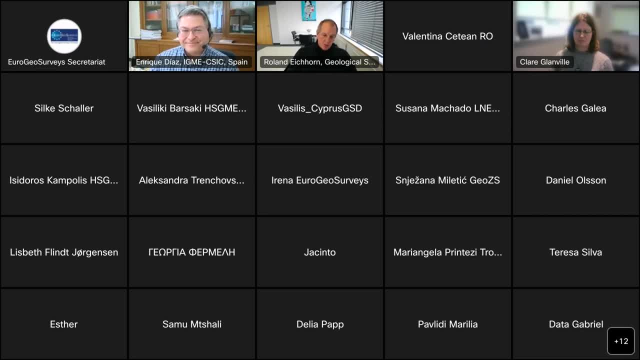 Uh, at least in the hard way, if you want to, to Get acceptance. uh, in the neighborhood There is a simple family and you have to convince a family that they should work on protecting a teal side. So you can't speak about uh. 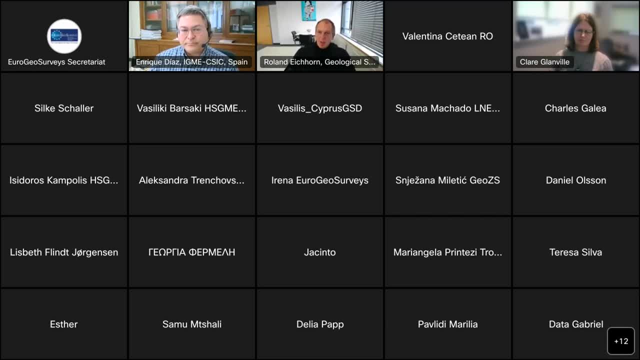 Special words, Which no 1 understands. you have to use a simple language, and the people are not stupid. They understand what you want, but you have to use uh simpler words to understand it. So you have to do it and you're: yeah, you, you can, uh, you can. 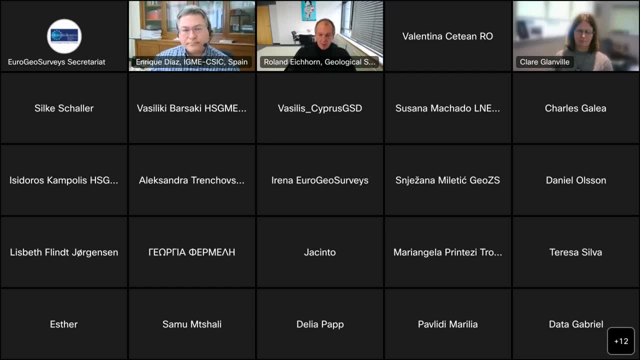 Get some critics which uh think this is now too simple. But uh, in my experience you can't be too simple. Uh, um it, I would hear. uh, I would Rather say it is a kind of arrogance, if you think. 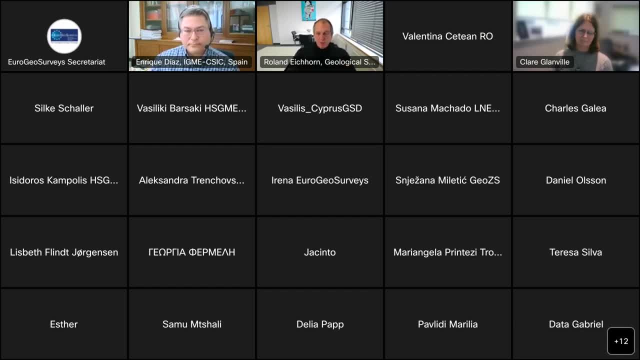 Uh, you have to use your special wording. No, you don't have to use it. Keep it simple and uh, you will be loved. Thank you, Yes, Do you want to say Yeah? well, I just agree completely with Roland. It's very important for us um to speak in a language that people can understand. 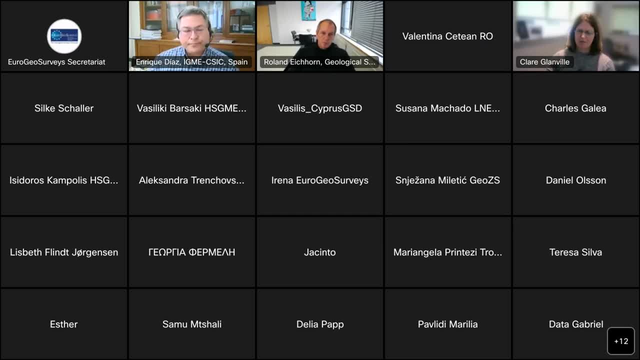 Uh, if we talk only in scientific Language that other geologists understand, we're only ever speaking to ourselves. We're talking to the converted. And what's the point? Because these people already understand, they already have an enthusiasm, They already have an interest. 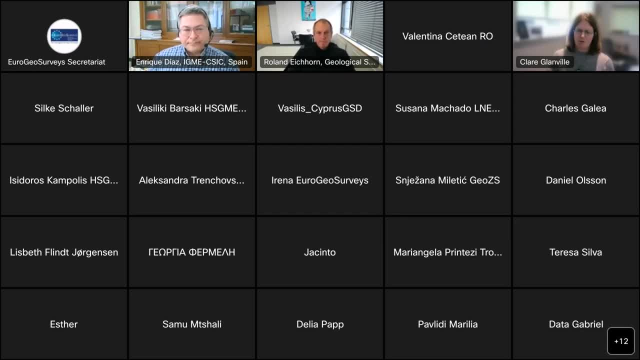 So if we want to Make more people aware and share our enthusiasm with more people and bring more people's awareness on boards, Then we have to speak to them in a language that they understand And- And as Roland said, they're not stupid. they just don't have the vocabulary perhaps that we have, And so I think it's really important. And for the critics, you can always have different levels of information. 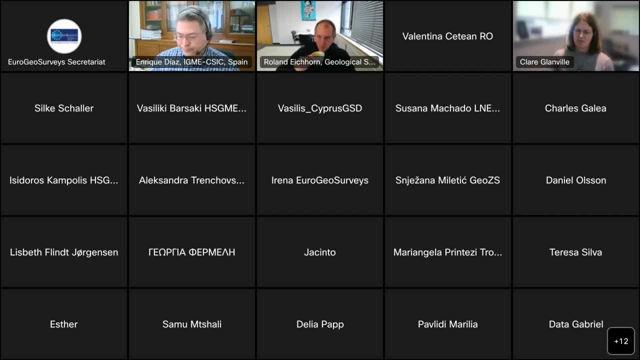 So you need to speak to your audience, So you can have a level of information to speak to the general public. You can have the same information, More scientific, if you're talking to a different audience. Yeah, that's exactly what Nicolas was mentioning in one of his last. 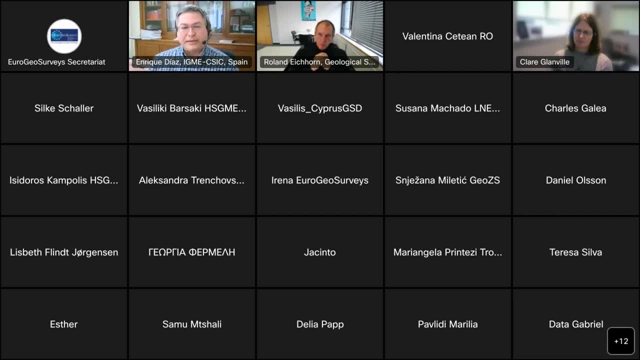 slides in the conclusions that we have to adapt to the audience. If you have a scientist, talk in the scientific language, but if you have lay people that are just basic school, then there's many ways of making it funny: making it simple, making it attractive. 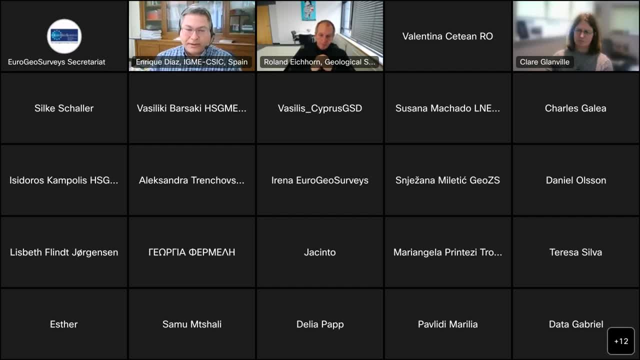 as we were all mentioning- that once you have their attention and their willingness to continue listening, then that's when you are hoping that they will engage with the site, that they will want to learn more, And that's the opportunity. And I think it's most important for GeoHeritage because it's 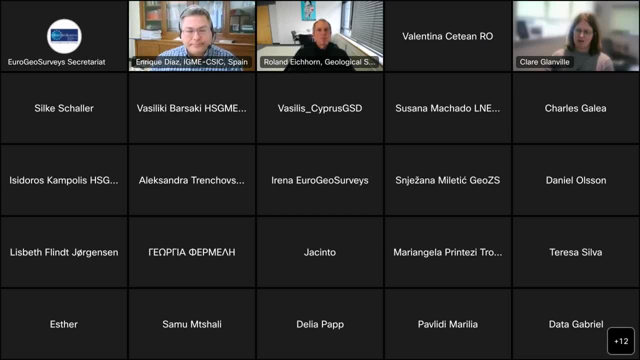 everybody's GeoHeritage. It's heritage for everybody, It's not just heritage for geologists. You know, I think it's most important in GeoHeritage to speak in those simpler terms. you know, perhaps if you're in other disciplines of geology you might have a different audience and you can speak more technically, but in GeoHeritage I think it's really important. 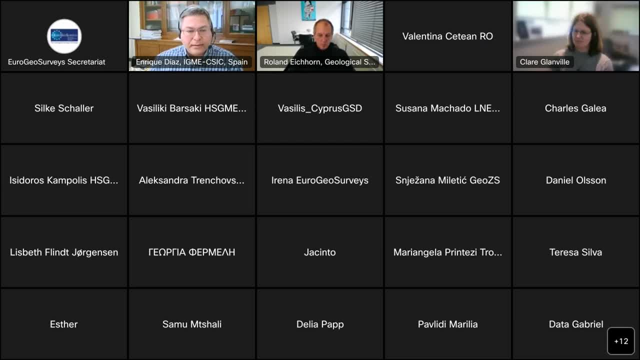 I don't know if there's anybody that wants to raise their hands to make a question and Laura can open their mics. Um, I don't see anybody. Well, there is one issue, I guess. Who is this? There is one question? Hi, there's one quick question from Greece, um to. 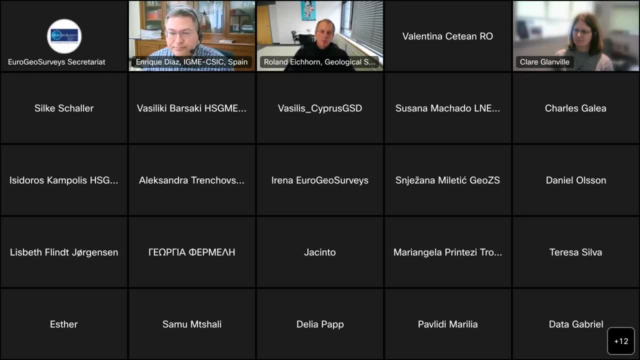 In the chat To Claire. Yeah, Have you considered making a 3D model of the coastal geosite which is threatened by erosion in order to preserve the scientific knowledge? A 3D model of the coastal geosite? Yes, um, thank you, That's a great question. Um, we uh have. we haven't done a 3D model uh for that. Um, we have 3D models for some other sites. Uh, it really comes down to um resources and our availability. 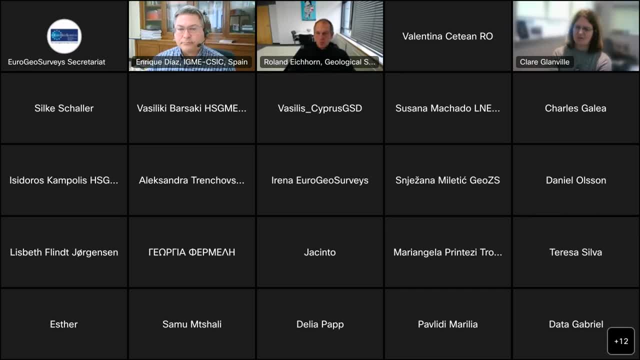 Um. so within geological survey Ireland, the GeoHeritage team is very small. It's myself and one other, So although we have all the other staff in the survey to support us, it does come down to uh resources and if we were able to encourage the developer to put some more um. 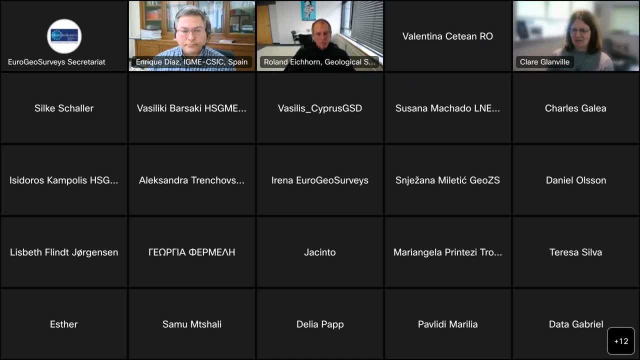 Effort and energy into it. It's something we could have worked with them. but because the geologic- I didn't say it in my presentation- but the county geological sites, they Aren't protected by law. They have no statutory protection. They're just protected through their inclusion in these county development plans. So 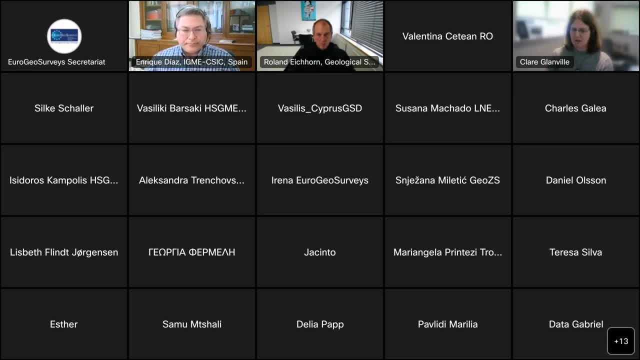 In this case. in many cases it works, but in this case it was Just by our working together with the developer that we were able to Implement any sort of change, and the developer had no obligation uh to Uh under law to to do anything. he could quite happily just covered up the whole geosite. 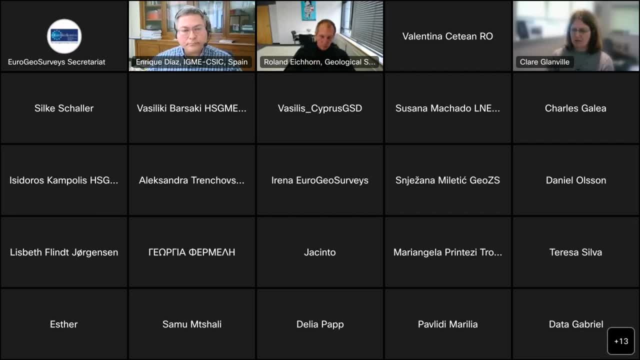 And moved on. but, uh, by working with him and making them understand the importance of the site, they were happy to to look at these alternative. uh, cliff defenses It and that is at their own cost. So, Um, a 3 D model would be lovely to have and we did look at other. 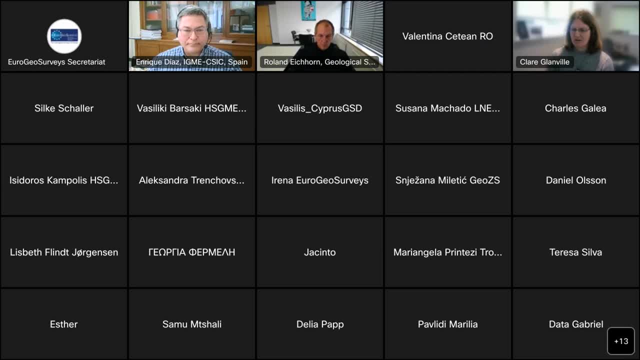 Measures for um, recording the heritage at the site if it was to be Covered up. so whether we could do um things like 3 D models, whether we could do some Uh drilling, whether we could do some trial to record some exposures further inland Um. but in the end we didn't need to do these because 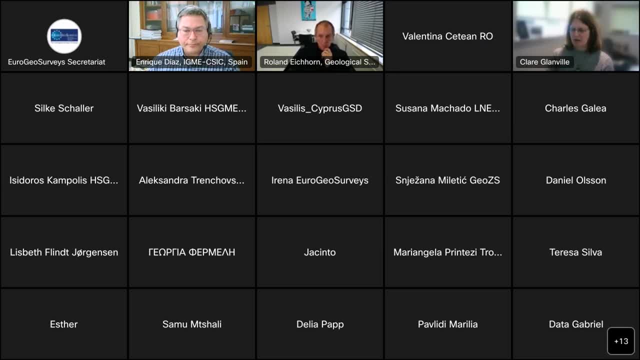 The developer was happy to work with us and, uh, Change and um Amend their defenses to to retain this section. So it would be a lovely thing to do, but we haven't done it. That's a long answer for a short. Oh, it's, it's good, Thank you. And also there was a comment that was just seen from Lee Smith. 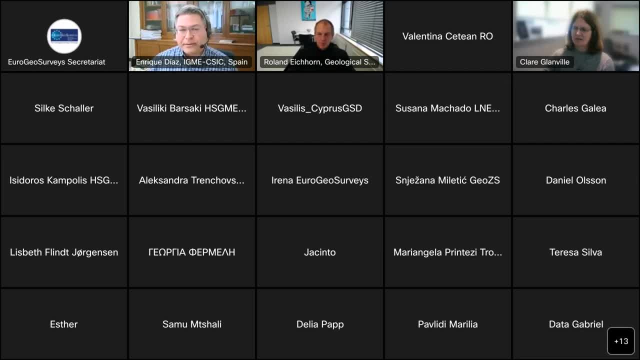 Clean. uh, if you have read, read it. it was mainly to Claire. uh, regarding Your presentation, Claire, um, but she's mentioning. it's not a question, It's just a comment. uh, That looks like the geological survey of Ireland had contributed to these. 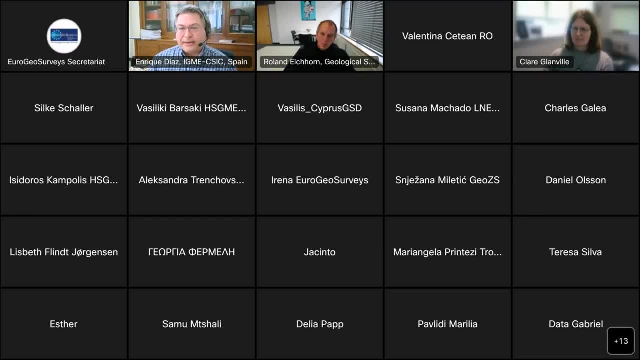 Tourist mine sites- tourist mine- That was uh included in the mineral intelligence. They mean Intel for you. you were also involved with that. Yeah, I wasn't involved with it directly. My, my, um, The person before me, my predecessor. 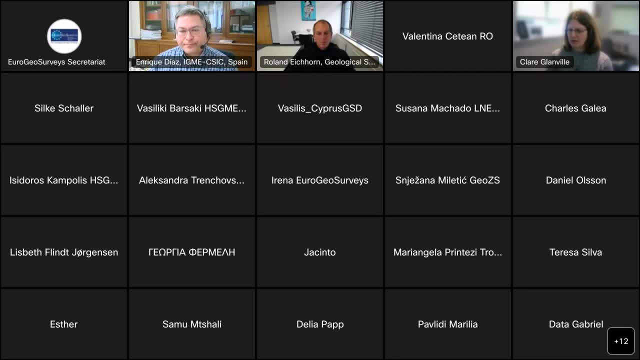 Was involved with that uh, and it was a project uh that we did With, uh, the EPA, our environmental protection agency, and we actually have um As a result of the project, a um historic mines database uh, which was, as you say, fed into the project Um. 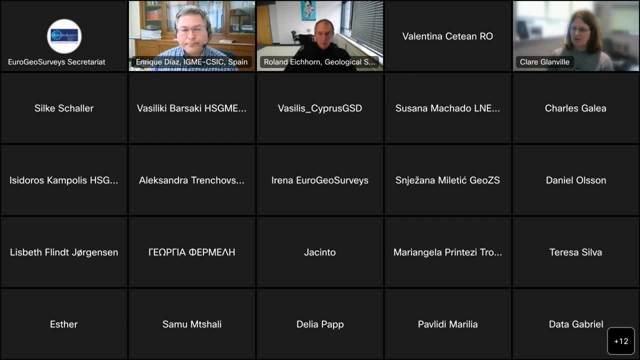 And yeah, many of those, uh, historic mines are also um geological sites and National heritage sites, so it The question talks about the and a feature map on your sites, um, which is something we've talked about as a heritage expert group within, and I think that's something that we may see in the future. 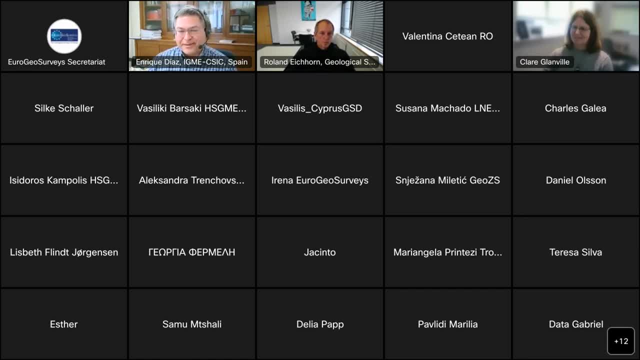 Is that right? Yes, Yes, Yes. Well, that's the idea. The only thing is that we have not announced yet because it is not yet there, But the good thing of this is that it's available For everybody in the web and that's so that anybody in the local communities, in the municipalities, they are able to see what is around them, What is. 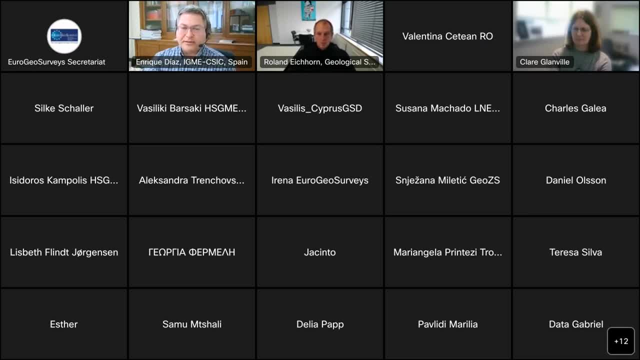 Both for, in our case, for your heritage, also in this Uh database that is already entered, that can be seen already through through the web. uh, about the, the minds and Uh. 1 thing that I liked a lot, uh, that the uh, the uh I've been doing- was this: 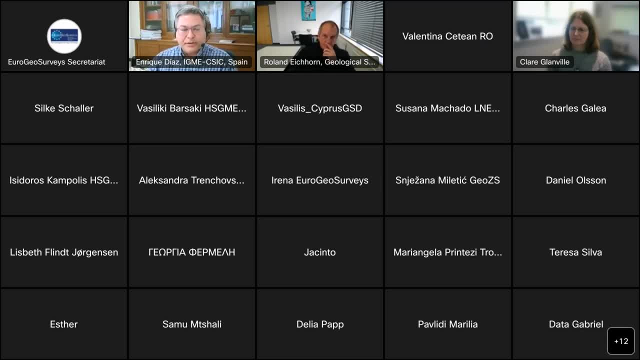 Collaboration with the, with the mining companies to, to emphasize that your heritage that Appears in the during the mining, during the development of quarries or whatever, and and how they can Uh collaborate with the local communities to or the associations or whatever to. 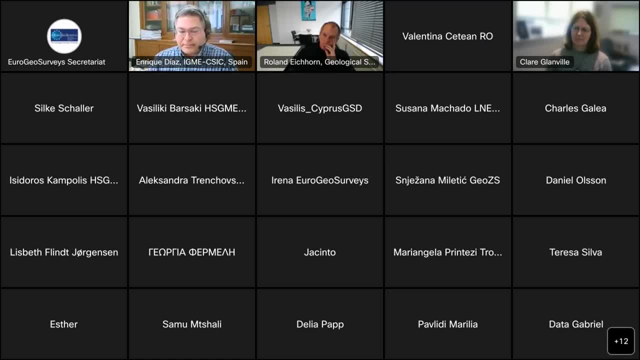 To include it to protect some sites that may may be important, maybe relevant and hopefully in not very far in the future We will also have also a database with the Geological heritage and uh, so that everybody can take a look and see in their countries around them. What is more important, of course, the, the main database is supplied by the national 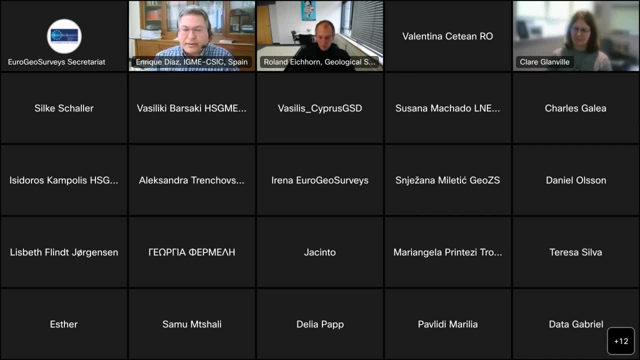 Uh government from the geological survey or or the the local surveys, like uh Roland, the Bavarian geological survey. but all this uh is best um taking advantage. you know it's, it's good. 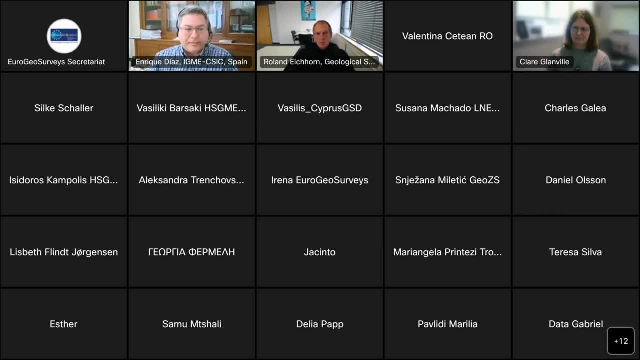 Uh, it's to be used when it is available to for everybody. And if you want to add anything else, let's see. we have some. We have from somebody from the, From the organization of African geological surveys. They're saying: uh, thank you so much for the webinar. 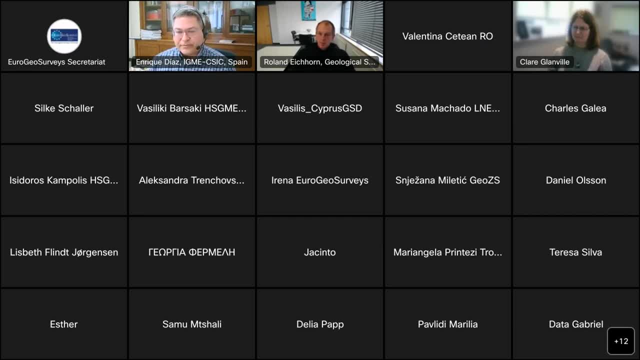 Informative and something to encourage Africa geological surveys to promote your heritage in their respective Uh countries, and surveys- Okay, We also have people with from Bolivia and I, but we are not getting many questions. I think we agree in some things, uh, that are very obvious. 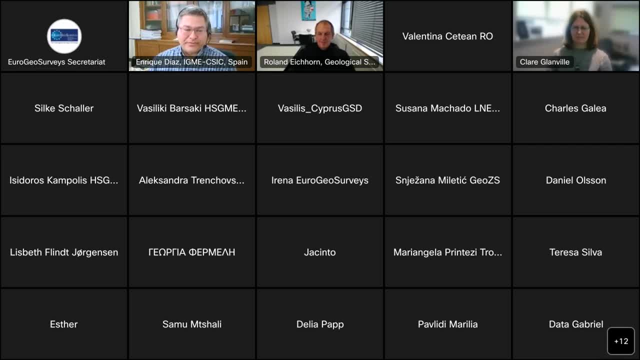 Uh, and the the good thing, I think, to conclude, uh, if For those who have been present at the At the session for today for this webinar about the, the local, I mean the socioeconomic uh, the contribution of geological survey, the theoretical heritage, also to the local socioeconomic development. 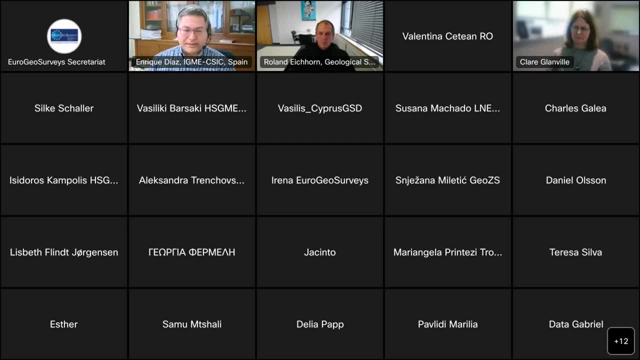 Is to learn that there's many possibilities to take advantage and that if this is Properly inventory, properly eh Valued, and we know what we should do with it and what we should not do with it, Then it is Possible to to obtain many benefits from from from this. 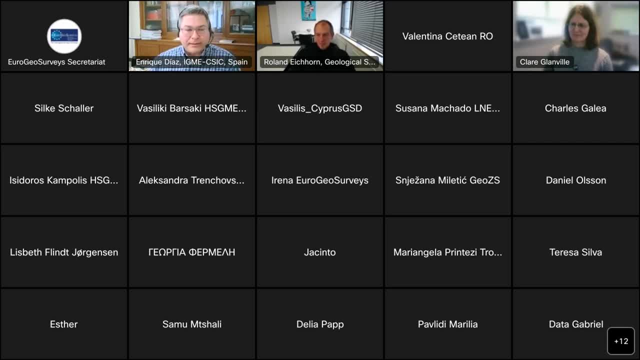 And, if you want to, I would like to hear a Roland and Claire, if you want to add the, or you know the, the main Conclusion that you would suggest for those people that are listening, That a contribution that you would like to emphasize. 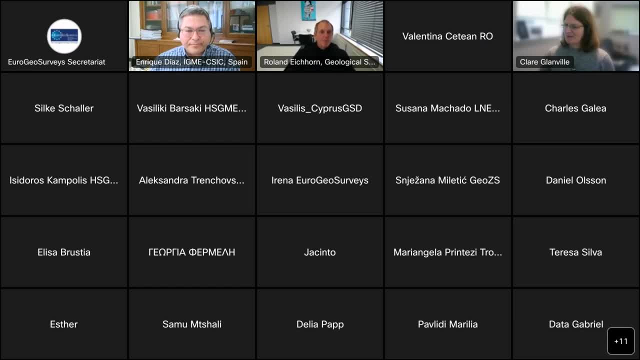 No, no, I don't think so, Enrique, I just um, I suppose, the importance of uh, Of the inventory, and the importance of this, the, the audits, and the um, The identification of the geological heritage sites. 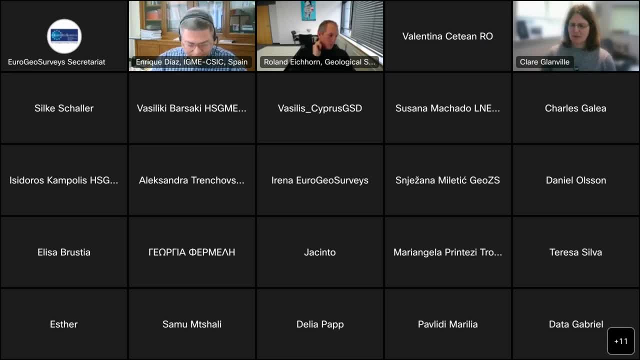 Once you have that done, uh, there's much more That you can move on to. like Roland spoke about, uh, you know, evaluating the sites, looking at specific management issues, looking at sites that are under threats, that need more promotion or need more protection. 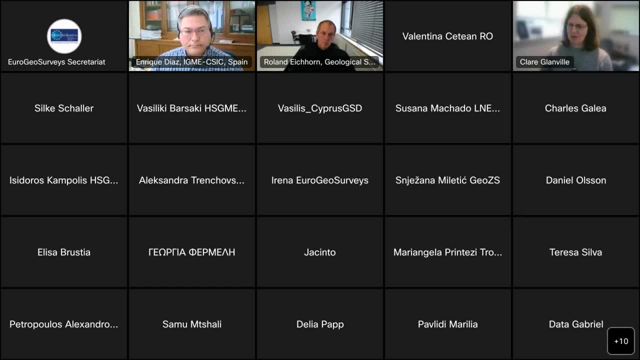 There's many things that you can do, but you as well- I was saying bottom up- you need to have The sites well documented and researched. 1st, Hmm, Well, close with the word. only You have to learn. 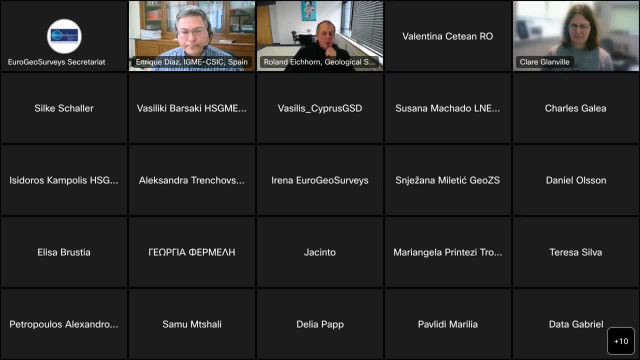 You have to know a thing Before you can esteem it, and if you esteem it, you're willing to protect it. I think this is the overall conclusion. Yes, that's right. Uh, that's 1 thing that, uh, when. 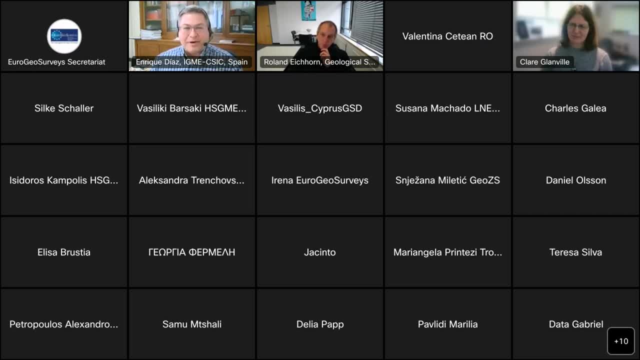 I remember in the 90s or 80s when we were talking about Environmental education. you need to know things and then, once you know them properly, then you will begin to To esteem, like you said, to laugh them, to enjoy them and then. 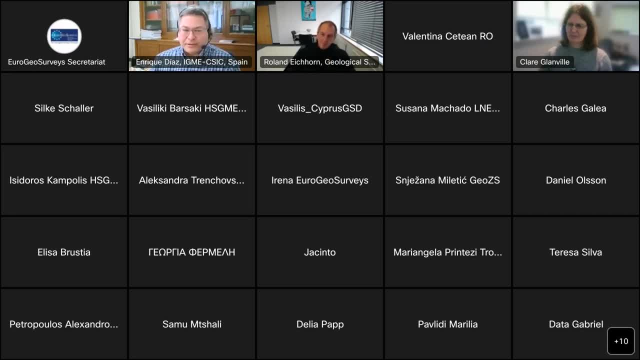 You will want after that, you will want to protect them and to use them properly, sustainably. That's right, thank you very much. I will let Nicholas know also, and thank you very much, Claire and Roland, And thank you to all the listeners I think we have had. 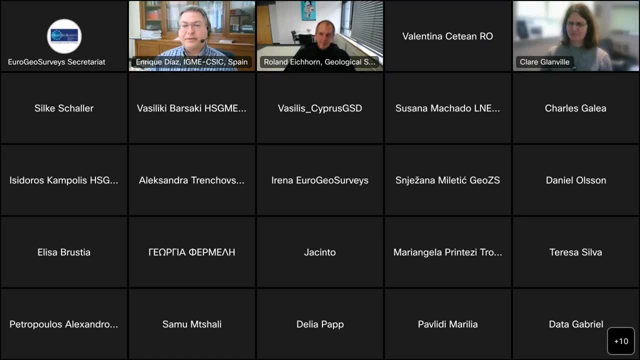 Uh, right now we have 35, but at the moment we had 42 people um present at our session and we will leave this, uh, uh, the the video in the YouTube channel of surveys, and we will later distribute or and also include the link. 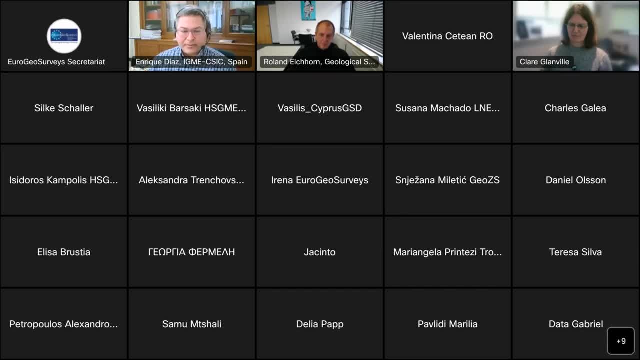 In in the surveys um Web page and also in the in our expert group and on the your heritage expert group, So everybody can See it later or share it with other people who might be interested. Thank you very much. thank you, The secretariat, for helping us with the. 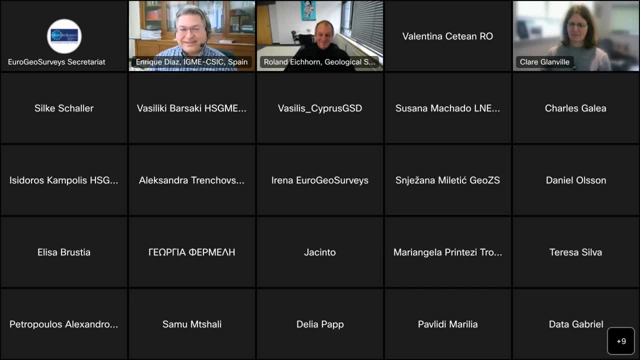 With the session, with the technical part and the Goodbye everybody and see you next year, for we will also have 2 other sessions related, or maybe 3 even We are preparing: 1 in relation to natural protected areas- Protected areas also the heritage injury in relation to mining environments- and another 1 of your heritage in relation to your parts and your tourism more more specific, to take advantage for the tourism. 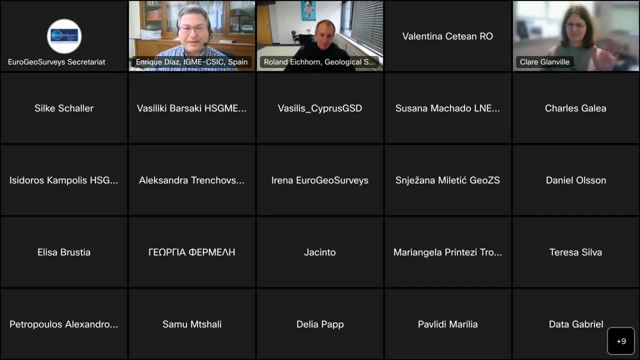 Okay, See you later. bye bye to everybody. bye Bye to everyone.